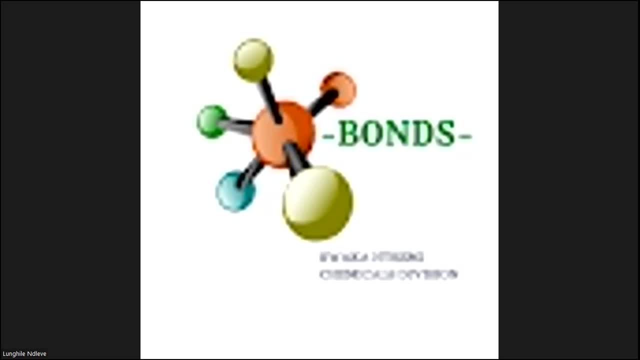 that are quite rare to find, especially for students that are doing self-study. So over the years I've worked with a couple of students. I joined master's students- recently even PhD students- to assist them with their design projects, And while doing that I myself discovered new ways of doing things And what I like. 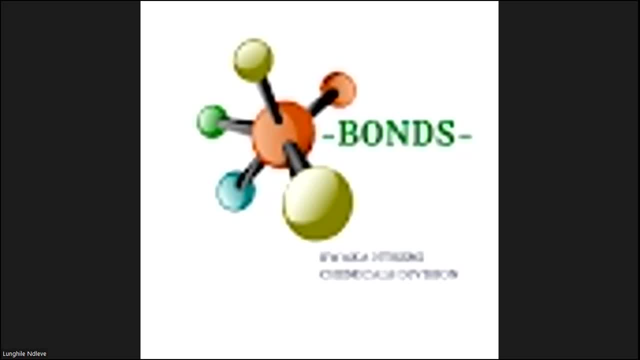 to do is to put them in document form, in template form, so that other people can be able to use them. So that's basically what we're going to be doing. We're going to be looking at the heat exchanger design. So it's a simplified heat exchanger, but it should. 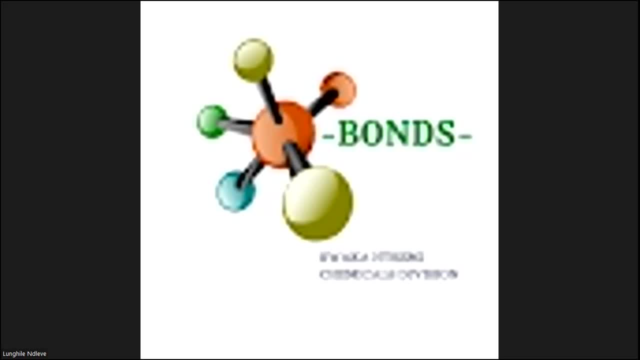 give you the concept and how to go about designing your own heat exchanger. So what I'll do now is I'll just share the screen so we can get started And we'll go through the different stages, starting with calculating your heat duty, then going on to your estimating. 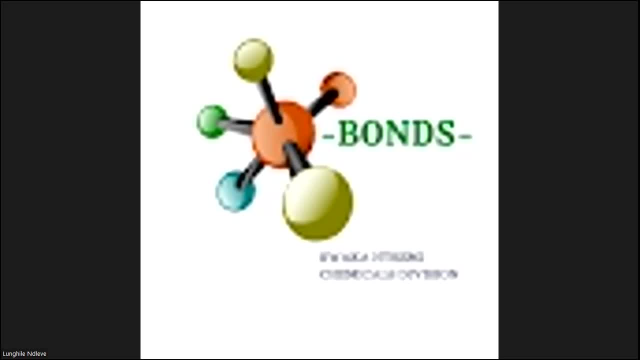 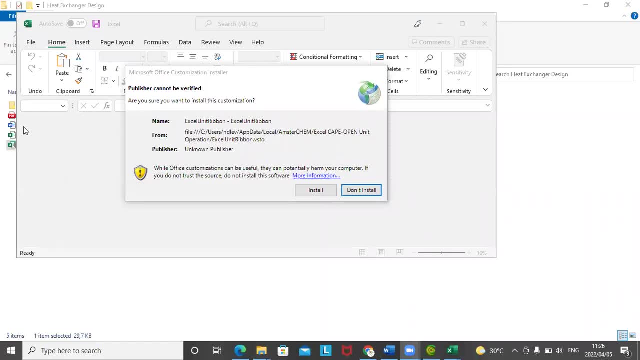 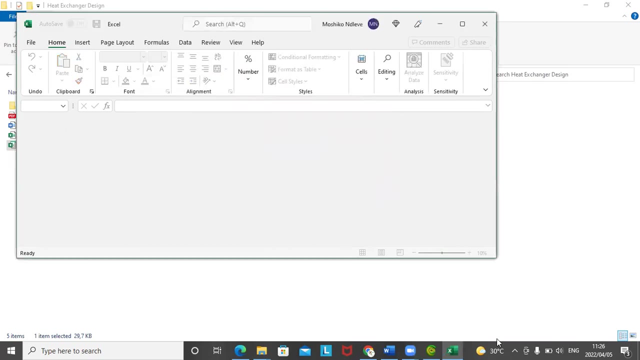 your heat transfer area and going on to calculating your transfer coefficients. What you need to do as a student obviously is you cannot just rely on the guideline that I gave you right. The most important thing is to go through your textbook, is to understand. 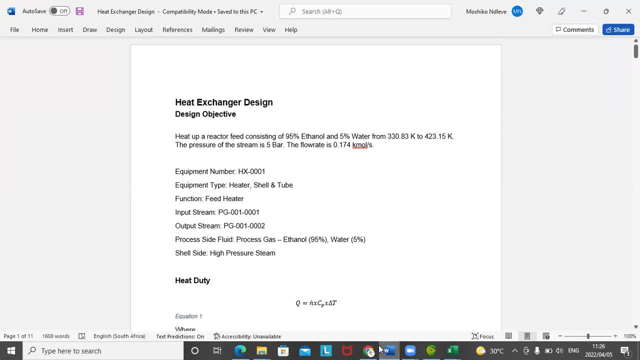 with this particular presentation. I won't go deep into the details of the method we're using, how it was derived, whereas for you, as a student, it's important for you to go through this thing so that you have a deeper understanding of what you're doing. So let's 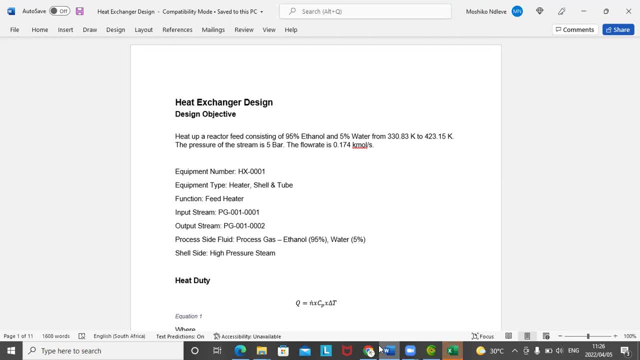 get started. So the first step is to heat up a reactor feed consisting of 95% ethanol and 5% water from 330 degrees Kelvin to 423 Kelvin. right, So the pressure is 5 bar and the flow rate is 0.17 kilovolts per hour. So this is just a random design question based on some arbitrary 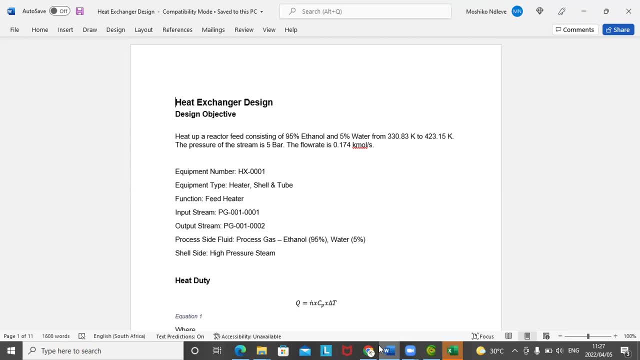 design project from one of my students. I just created it so that I'll be able to take you through the steps. One thing you want to do is you need to get into a habit of being formal in terms of your annotations, in terms of your equipment number, because that will help you when you get to. 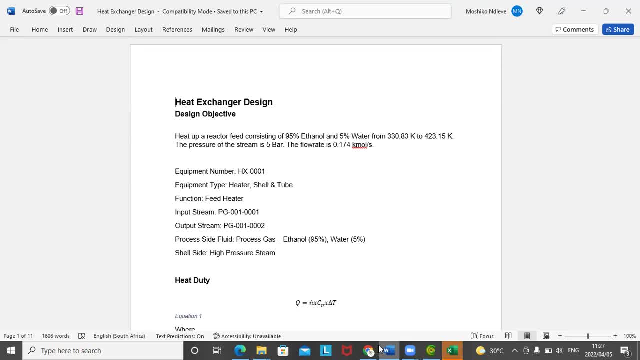 the heat activity to things like P&IDs, design PFDs, your documentation of your work, because what that helps is in the future, especially if you end up in a design environment, as I was in, that will help you a lot, because design is mainly about cataloging. 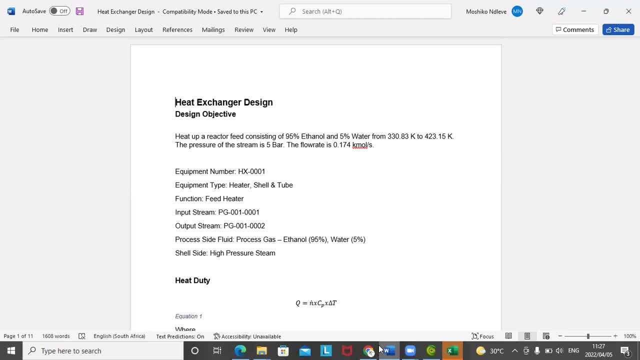 And documenting. you do a lot of literature review and you need to be able to document the literature that you read so that, when the time comes and you need to grab certain information from certain sources, you are able to find it. So get into a habit of cataloging. 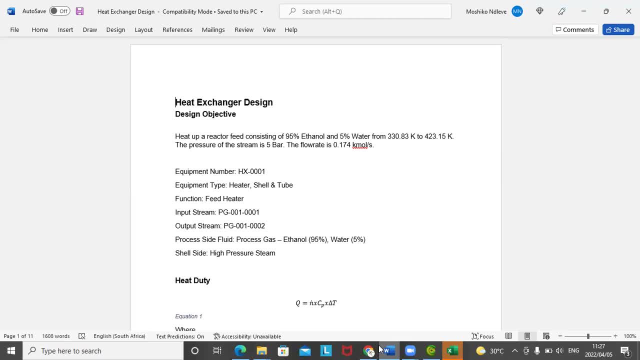 your work properly. So one thing: process side, we've chosen to put in what? The ethanol and the water, and then on the shell side, we're going to put in the high pressure state, right. So That's the heat exchanger we're going to design and I'm going to take you through how we will. 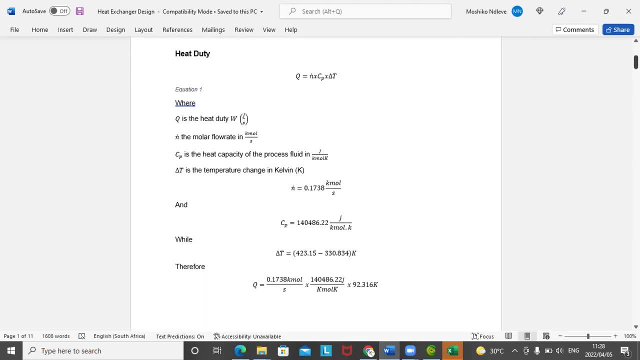 do that All right. The first step, obviously, is determining the heat duty right. So there are two ways of doing it right. You can calculate it manually or you can put it through a system like COCO, right COCO, which is a simulator which, by now, if you're doing a plant design, 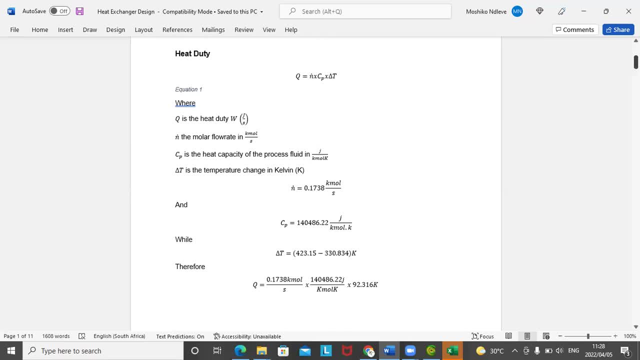 especially. Yeah, Yeah, Yeah, You should have been introduced to assimilated. So the first thing you need to do is calculate your heat duty right Manually. the formula we'll use is what Q is equal to number of moles. 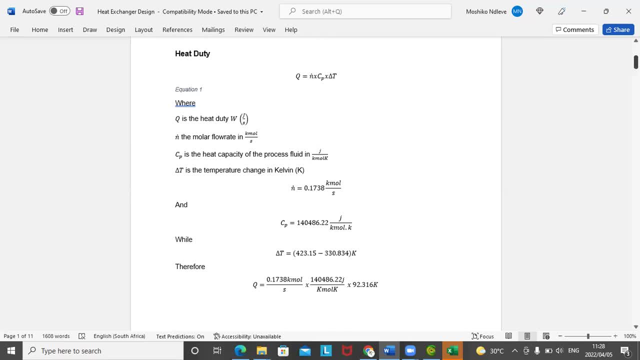 CP. Delta T. If you're using number of moles, you must make sure that your CP is given in what? In joules per kilomole Kelvin, Whereas if you're using mass, you must make sure that it's given in joules per KG Kelvin. Just be careful of unit operations. This is something that I will be. 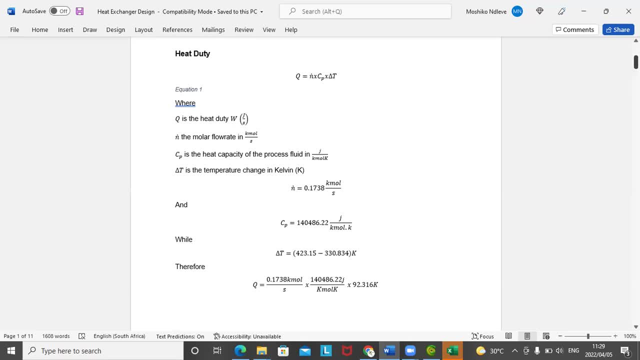 emphasizing a lot during this design, because you know if you're using mass, you're not going to be able to calculate the heat duty. Yeah Yeah, You're going to have a lot of heat duty when you're doing mass. 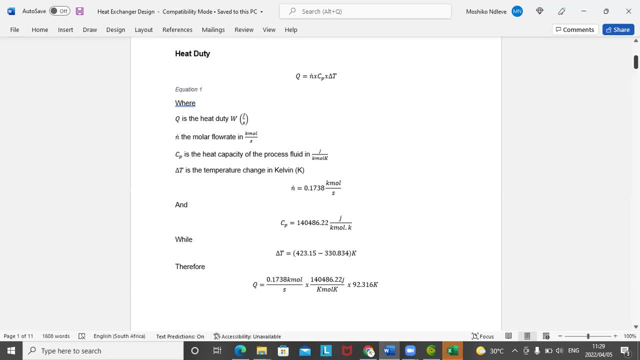 Yeah, Because the one thing that happens is you end up getting a reasonable size from your equipment and you're surprised: where did that come from? And one of the reasons you will have the challenge is not paying attention to your units. That is very important. So your unit? 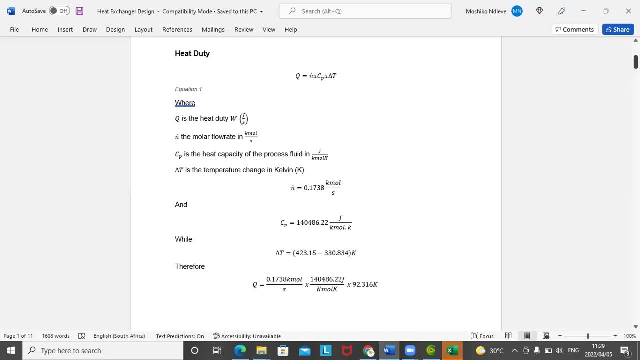 conversions are critical in making sure that your design comes right. So in the case where you calculate it manually, so you have your flow rate, you have everything. this is how you get your heat duty And in this case we are going to calculate the heat duty. So if 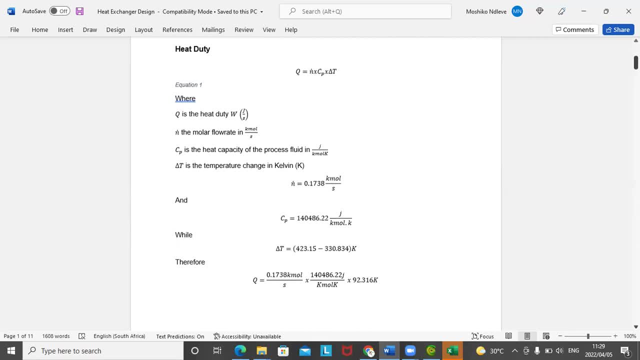 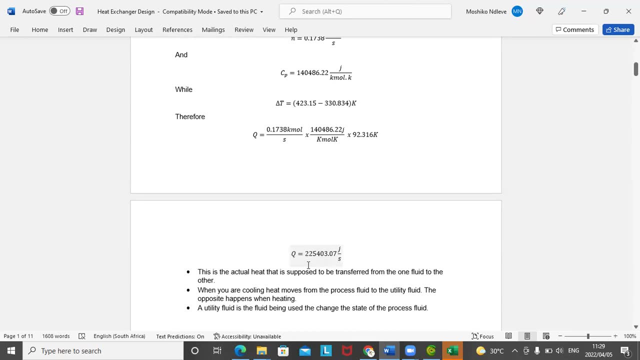 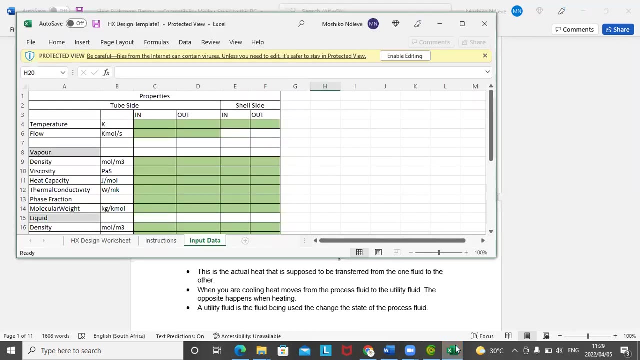 you have a steady flow rate, you have everything. This is how you get your heat duty and you're um. what you'll come to is the answer will be 22 000, but the 225 403 joules per second right. and then what we'll then do is, if you go back here, i've created um, i've created a uh. this the. 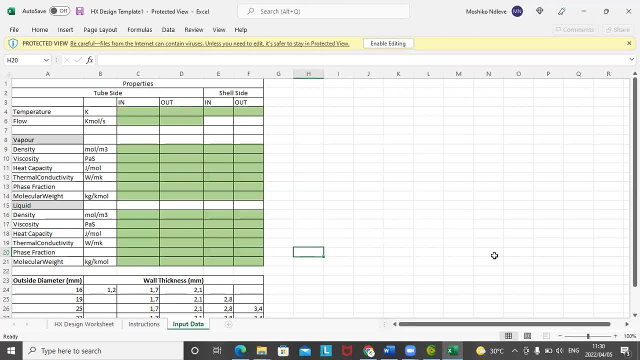 template i was speaking about is that um can be available to you if you want to use it. um. the whole point of this template is to, uh, one, have it available if students need it, and, two, um. this video will help you be able to navigate through this template so that the work that you do is 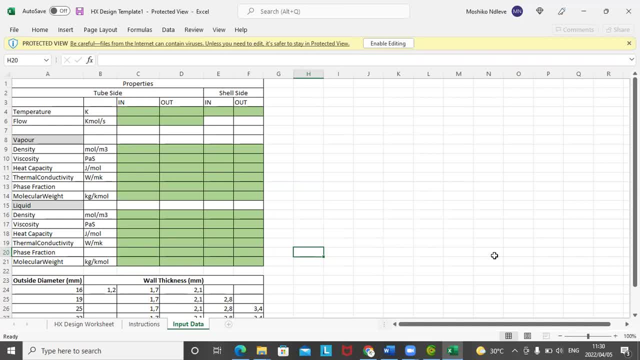 your own work, and the template is just simply a calculator that you use to punch out the numbers, but the one thing is it is not a shortcut to your design project. this is just a tool that you can use to work faster, and it's important that you also learn how to develop such spreadsheets. 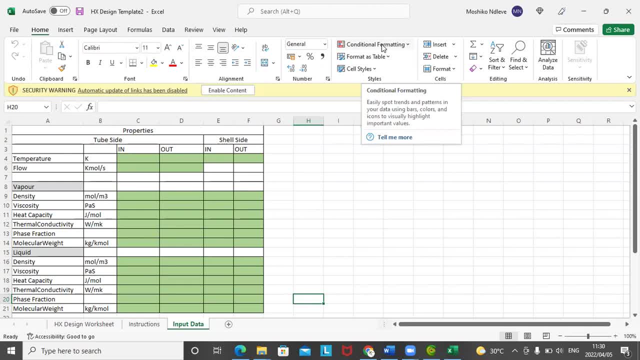 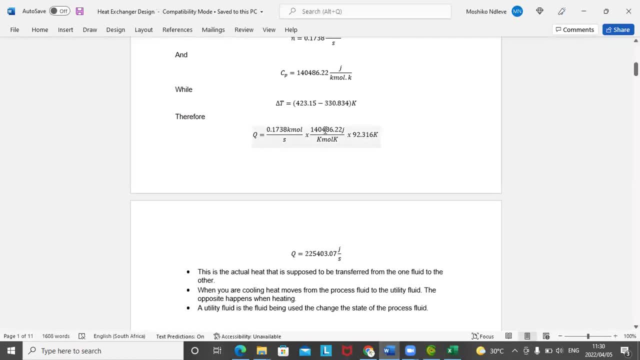 because design work is mainly about creating spreadsheets that will make your life easier. so, um, one thing you'll see here is now: we've just calculated the, the, the, the heat duty, right? so this is the actual heat that is supposed to be transferred from one food to another, and then when you're cooling it, 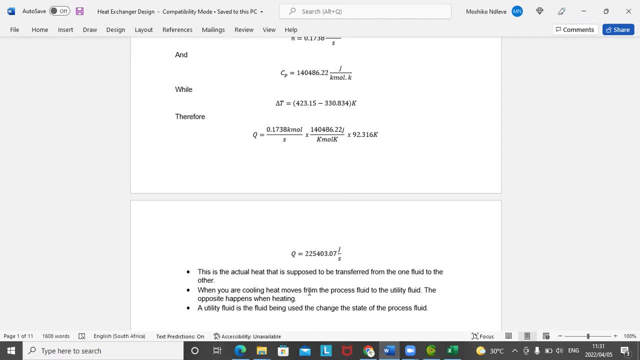 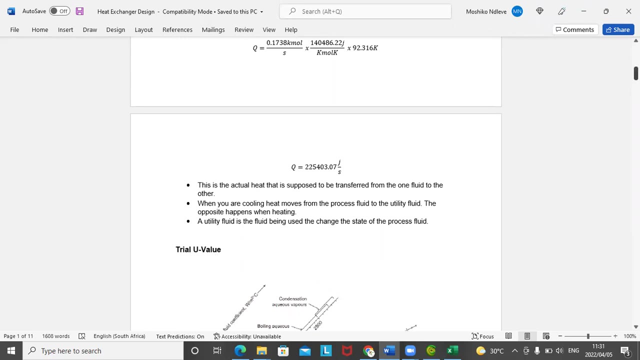 moves from where, moves from um the hot food. it's always when you're cooling the, the from the processed food, the utility fruit, and the opposite happens when you're heating right and then um. so if a utility fluid is the fluid that is used to change the state of the processed food, so um so. 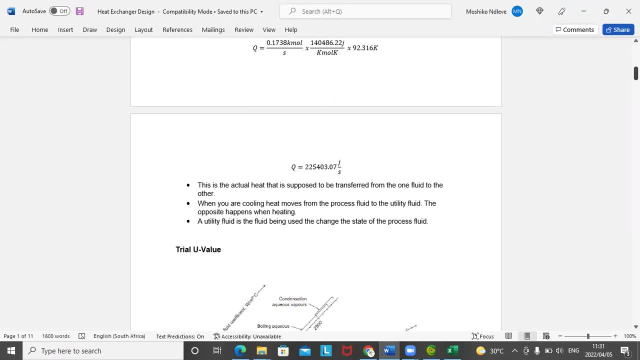 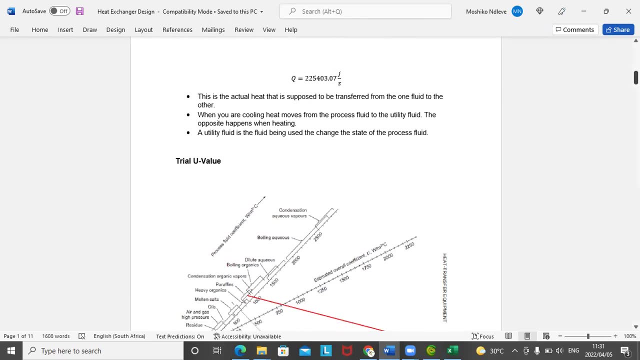 for example, if you want to heat something up, you'll get a steam that is hotter than that stream. that thing is called the utility, right, um? and then let's continue now, um, before we get anywhere, right, um, the next step that comes after that is estimating the trial eu value, which is the overall. 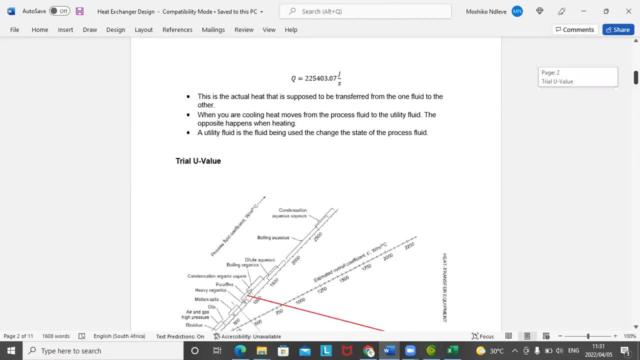 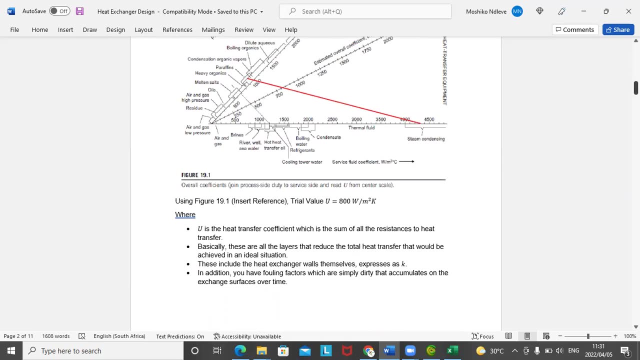 um transfer coefficient. now let me just take you through a few things about that right. so the heat transfer coefficient is the sum of all resistances, right of heat transfer. so basically, if you are doing um conduction through an electric wire, uh of electricity, your resist, your, your, your. 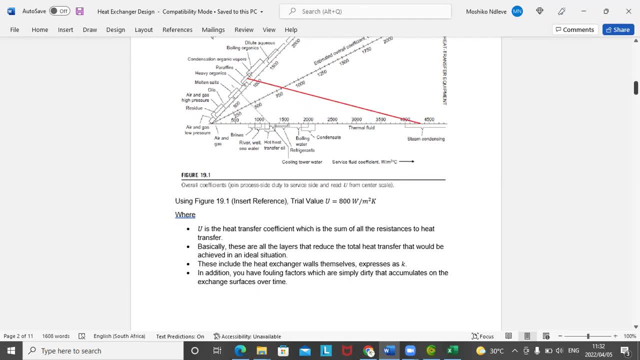 overall heat transfer coefficient is similar to the properties of the metal that electricity is flowing in that resist your flow of electricity. So your overall heat transfer coefficient is basically a total right. it's all the layers right of of of conductive material or non-conductive. 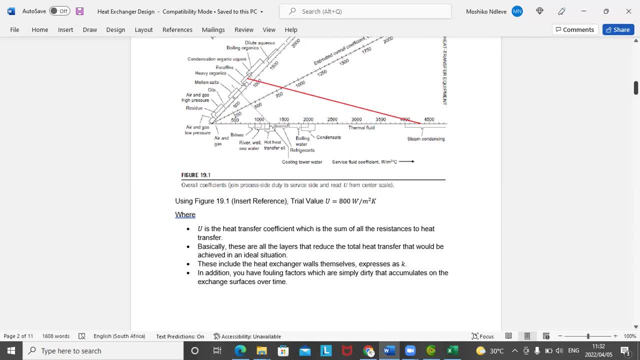 material, because obviously it can be completely non-conductive, of course, but it's um a collection of all those layers that will reduce your overall heat transfer right, and this includes the heat exchanger walls themselves and it expresses k. so if the material you're using will have a will have. 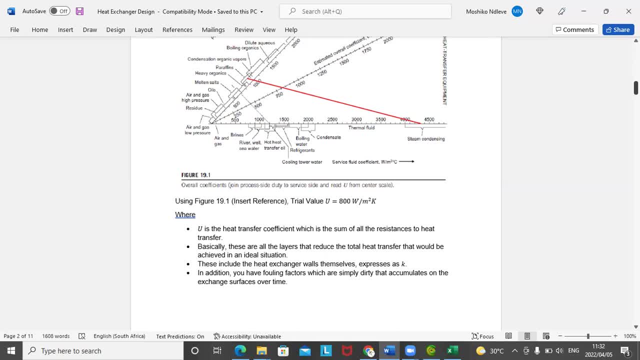 a conductivity. that is how much heat transfer it will allow through. We'll also have fouling factors. This is if you look at inside a kettle when you're boiling water, you'll see it will start accumulating a layer of flaky material. 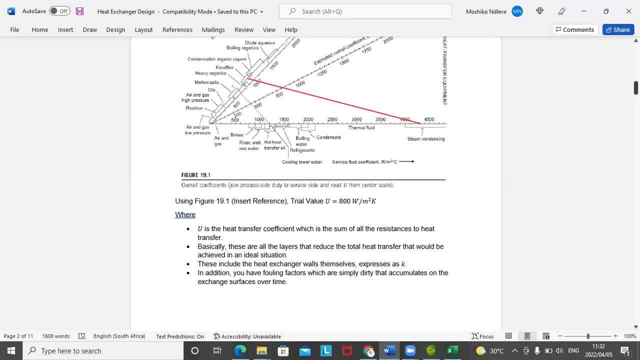 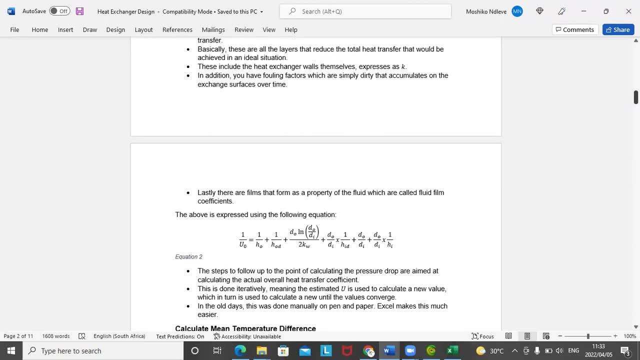 That's the same kind of material that we're talking about when we talk about fouling. And then, lastly, you look at the properties of the fluid itself, where a fluid will create a film if it's moving at least a certain surface. 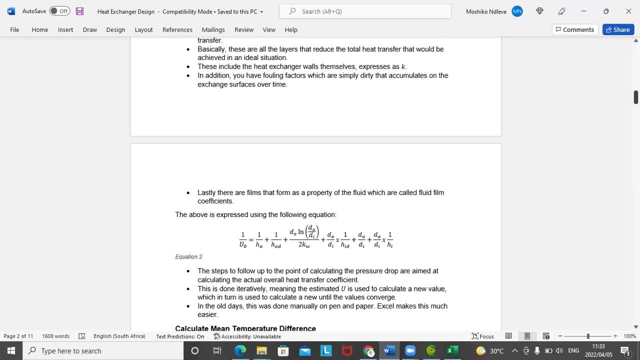 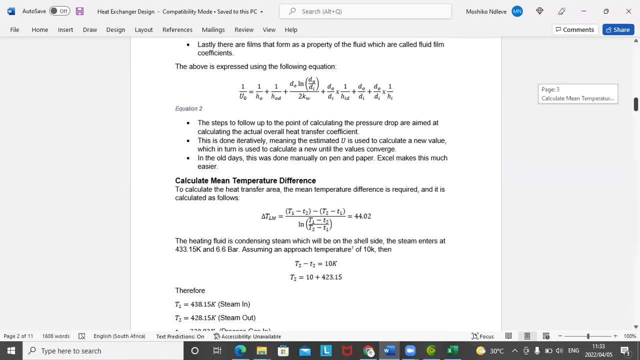 and that film will also create a heat transfer barrier. So this is the equation that we are trying to get as the first step to designing our heat exchanger, And just to jump ahead a bit so that you have a general understanding of where this comes in, right? 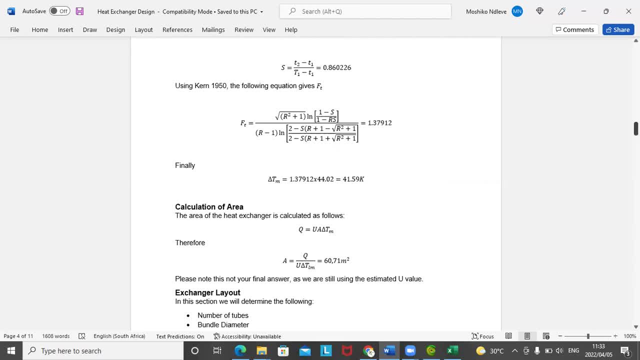 I'll come back to the equation above, but basically when you calculate your heat transfer area, it is heat duty is equals to your overall heat transfer coefficient multiplied by the area, multiplied by Delta T mean, by the mean temperature difference. So the whole idea is we are trying to get 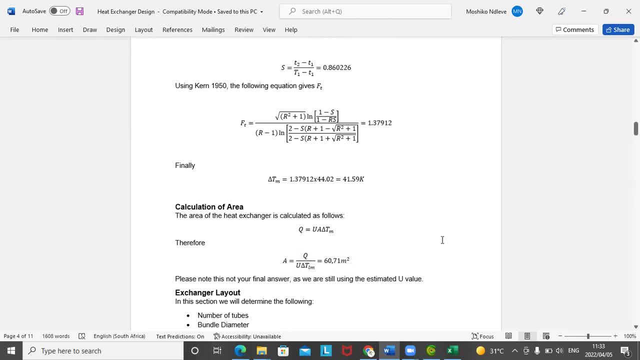 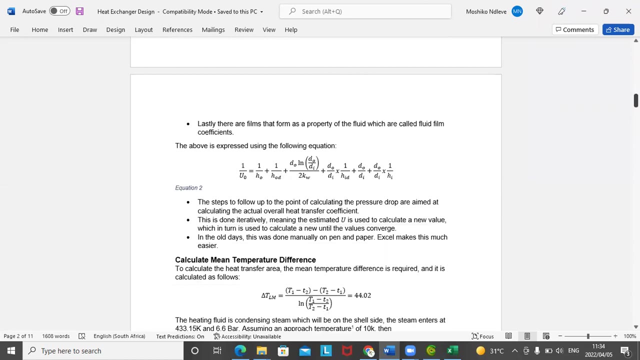 that overall heat transfer coefficient so that we can calculate the total heat transfer area. So let's go back and be systematic in terms of our procedure. So first step is you need to understand what your overall heat transfer coefficient does and that you can do more of it. 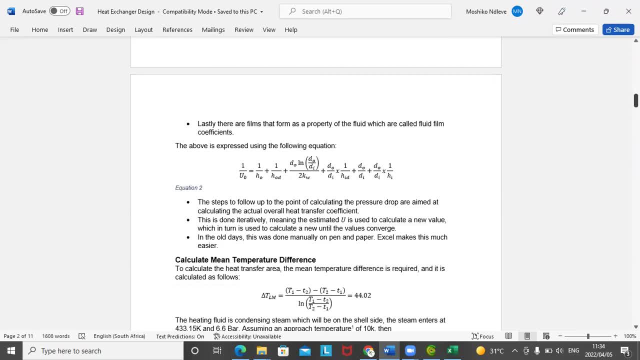 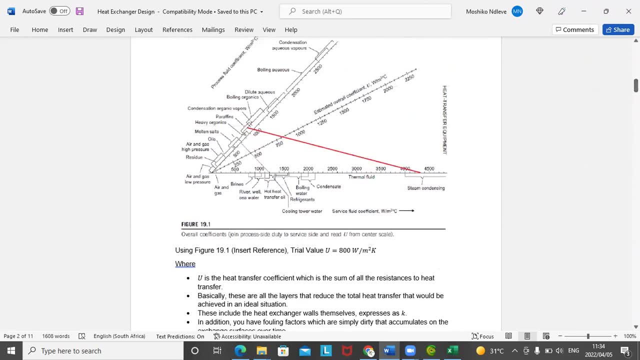 So, to get started, the first thing we're gonna do is we're going to estimate an overall heat transfer coefficient. Why right? The reason for that is, initially, you need to be able to get started with your calculations, because the overall heat transfer coefficient 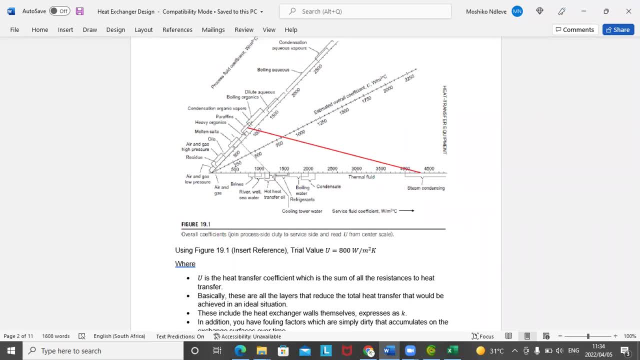 opens up your path in terms of being able to calculate everything else, right Just up to the present drop calculation. So it's the first thing. it's the first thing you need, And in order to be able to do that, you need to be able to estimate it. 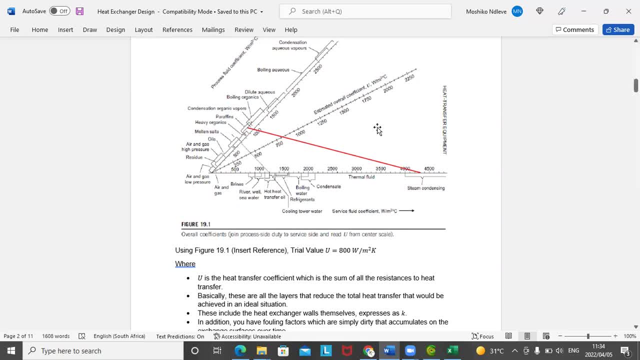 So if you go to your design textbook, you'll find this particular table where it has the. it has the surface fluid coefficient on the bottom and it has the process fluid coefficient on the top, And then the line here is your estimated overall coefficient. 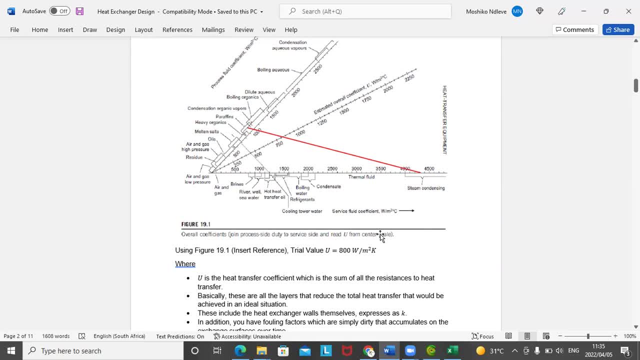 So the whole aim is to be able to join right Your surface fluid coefficient with your process fluid coefficient right And the way it intercepts the overall coefficient that is the value you're going to be used. So, because we're using condensing scheme, 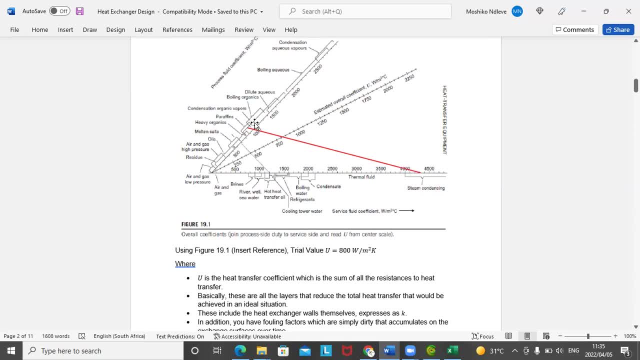 so between 4,900 and 4,500, and then I choose that point and then you draw your surface fluid. So we're dealing with with what's it? what is our with what? dealing with ethanol or dealing with ethanol? 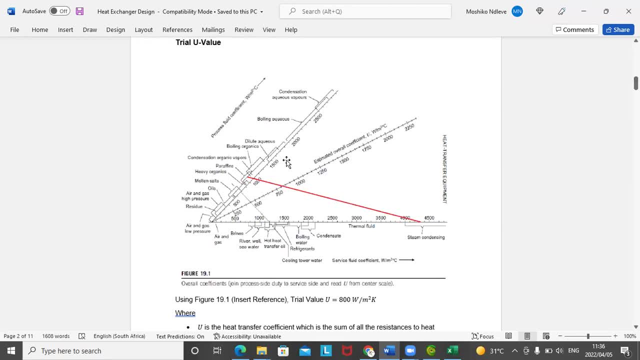 which is a light alcohol, which is an alcohol. Let me see if we are in the region. So so I placed it with the paraffins, which could be a bit wrong. It would be more suited in the region of your boiling organics. 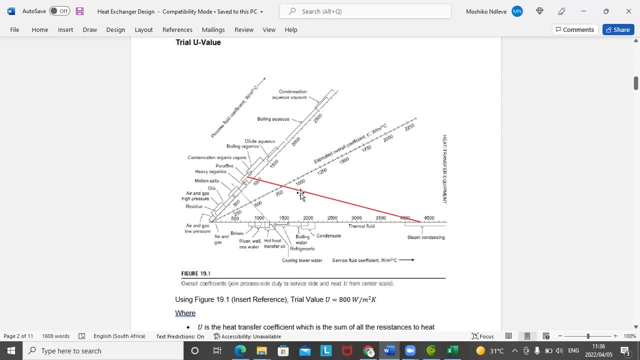 but you still come out to around the same number between 800 and so. So it's important that you identify your process fluid properly. I had placed it under paraffins, which is something you can correct. It's an estimate at the end of the day. 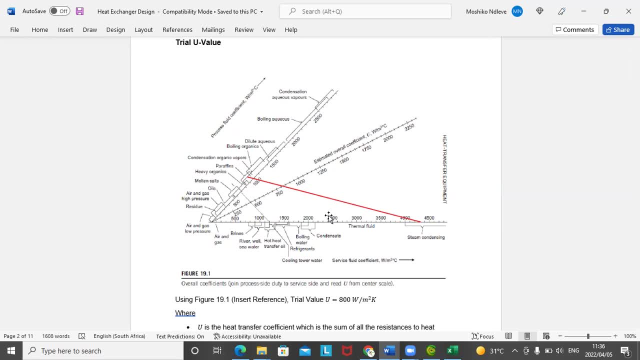 but it's important that you start off with the right estimate, because the method we're using is iterations, And one thing that can make an iteration go wrong is having a wrong initial starting V, which will throw off your numbers. That's quite significant. 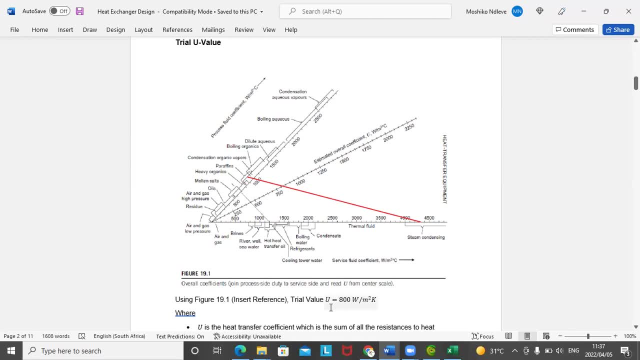 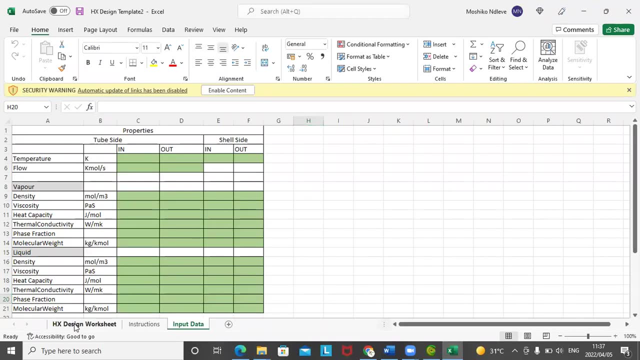 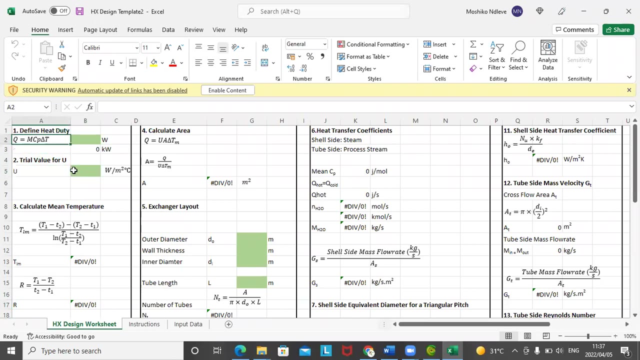 Okay, So we when I use our tile value of U of 800 watts per meter square Kelvin. So before we even proceed, let's go to our workflow worksheet And if you come here, you will see that already the template has been. 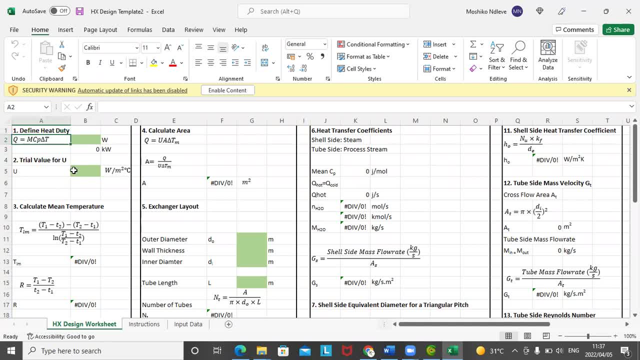 has been highlighted, where you need to put in values. For example, we've just calculated the heat due your heat duty. you need to put in your heat duty And this is where you will put in your heat duty, Your value. we just said 800.. 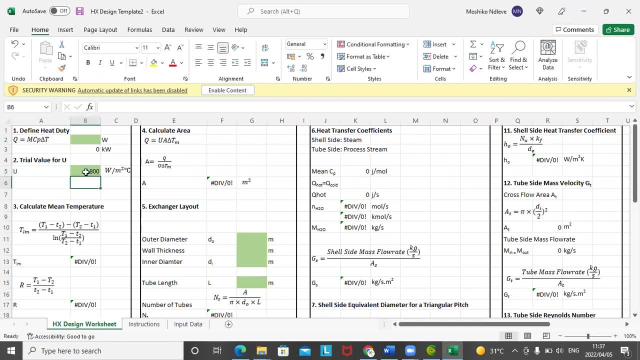 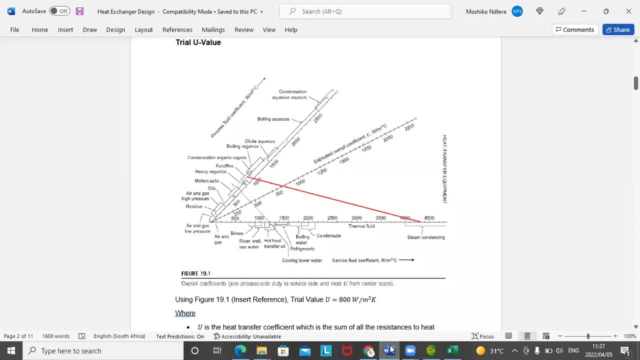 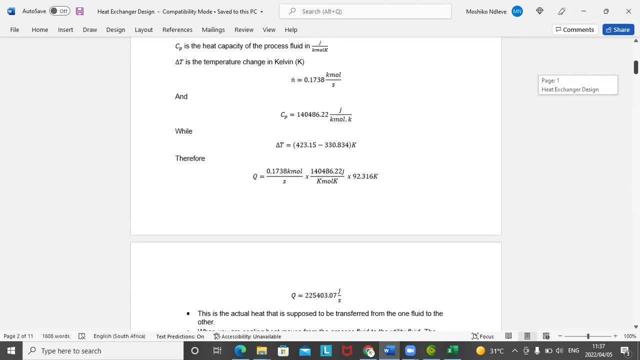 So let's punch in 800.. And then we go up and we then put in our heat duty And we said, oh, I heat duty- I'm gonna assume that my calculations here were okay- And our heat duty is 225.403 Jews per second. 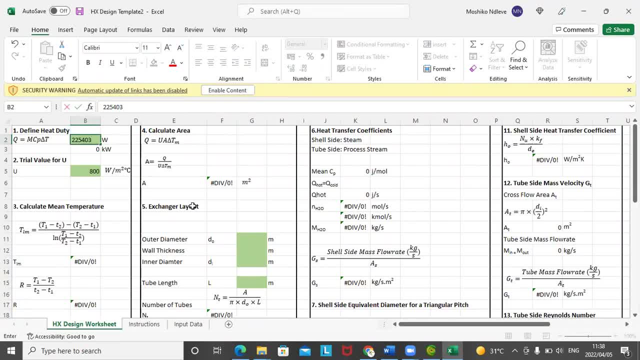 Two to five. Two to five: 0.5403 joules per second, which is one right. I think there was a 0.03 at the end. Then we allow that in. I'll assume it's not allowing us through. 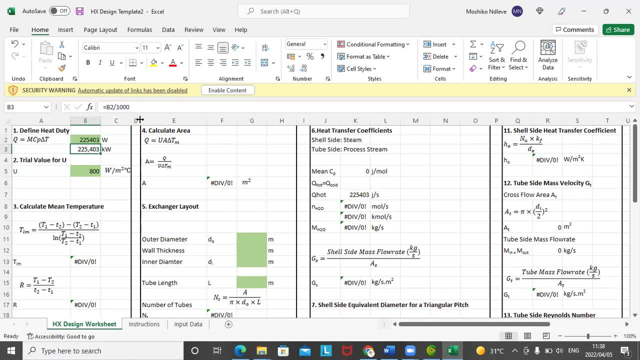 because of the formatting of the number. Okay, now, that's fine. So now we've got the first starting point, where you put in your heat duty and then you just punch in your estimated use value. Next we now come to calculating the mean temperature difference. 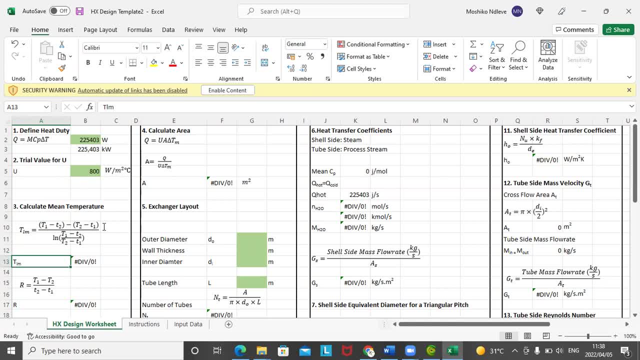 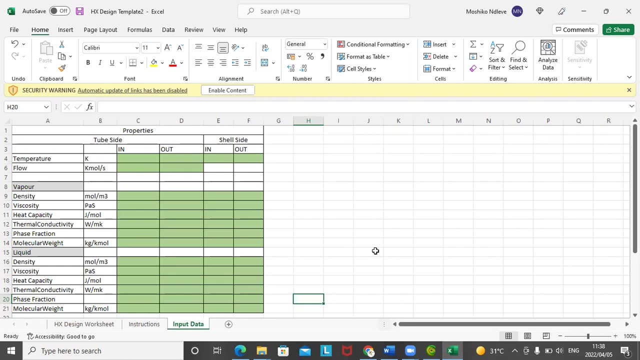 So the way this spreadsheet has been designed is that, in order for you to get answers, you need to be able to input the correct data where it is required, right? So let's go to the input data. So, before you even continue, what would be critical is for you. 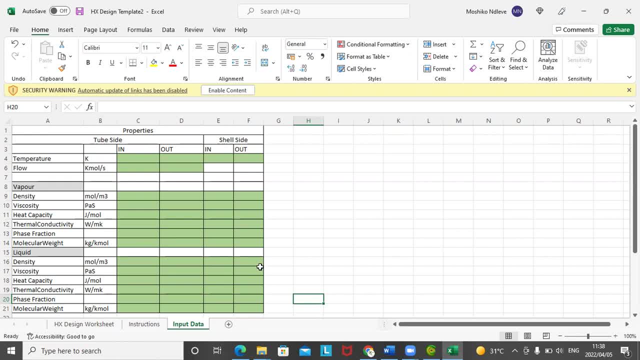 to fill out this committee right. And in order to do that right, as I indicated before, I use the COCO simulator, especially because now you want to get the densities, the viscosities, the capacities of a mixture which you could get manually if it was a pure substance. 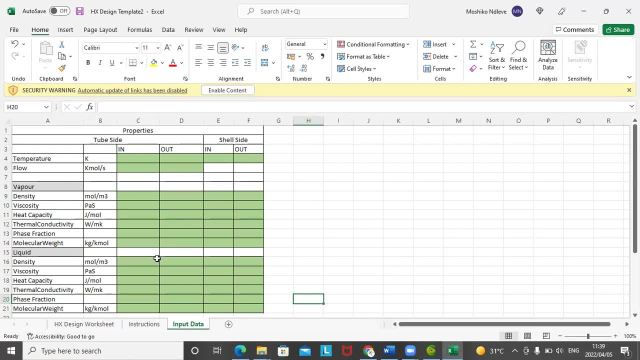 But the problem now is you've got a non-pure liquid which is 95% ethanol and 5% water, And the problem that creates is now you have a whole lot of calculations involving averages and all of that, whereas putting it through a simulator. 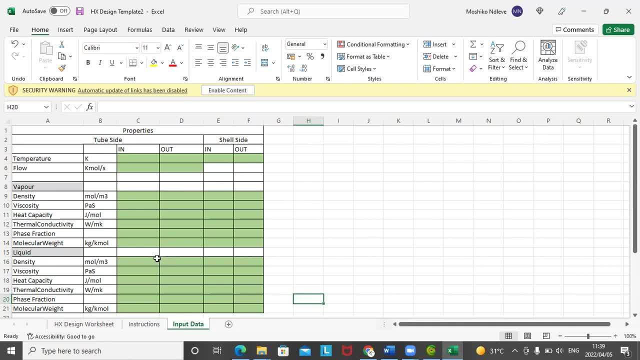 that will just give you a quick answer, and when you watch my other videos that deal with simulators, you'll be able to see why. So the next step obviously will be to fill out this table, but just so that we go step by step. 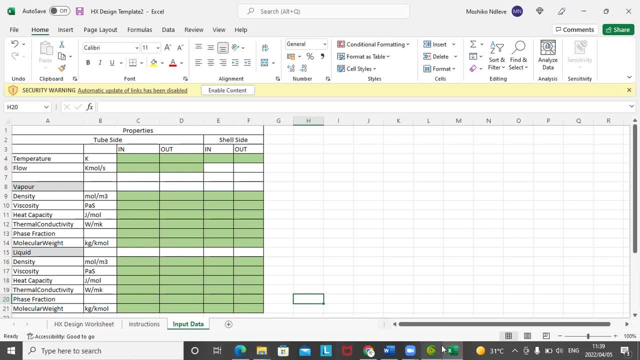 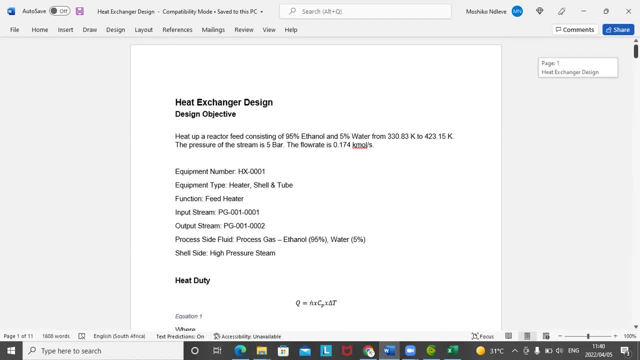 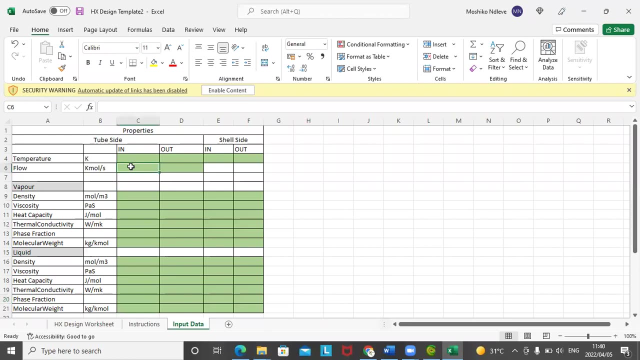 let's complete the information that we have already that we got as part of our design form right, So I'll just pull down slightly. For example, we know that our flow rate is 0.1, super plus 0.174 kilomoles per second, so that I can fit in 0.174, and because this is a non-reactive process, 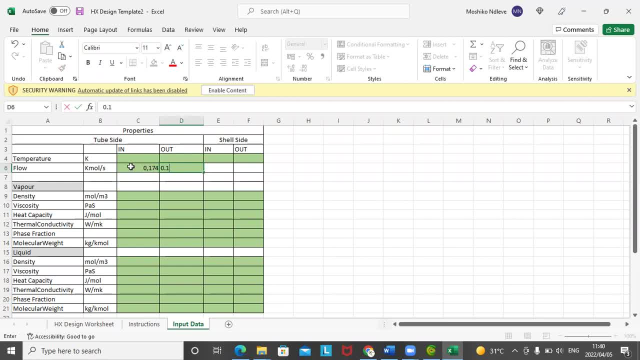 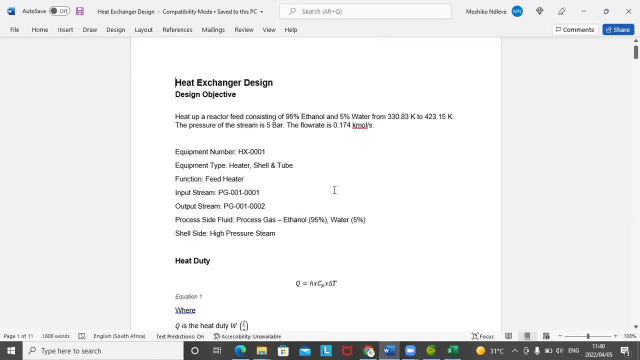 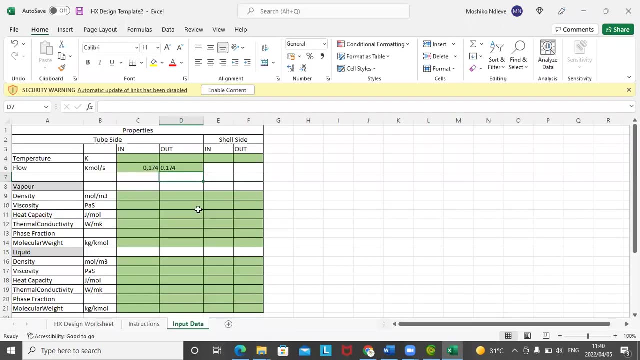 the number of moles coming in will be equal to the number of moles coming out right? What else do we know? We know that our process fluid is coming in at 330.83 Kelvin and leaving at 423.15,, so that we can already put in 330.15, and it is leaving at. let's go back. 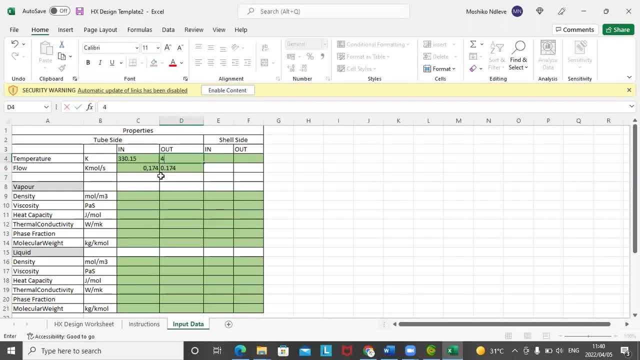 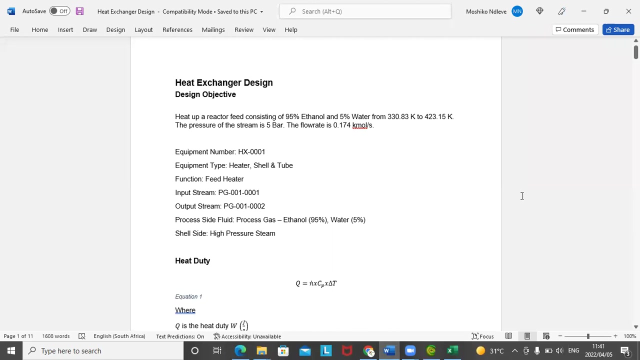 which you've got it right: 423.15 Kelvin, 423.15 Kelvin. It's coming in at 330.15 and leaving at 423.15, and then the one thing we can also calculate, of course, is the shell side, because we're using steam. so the one thing you need to be careful here of 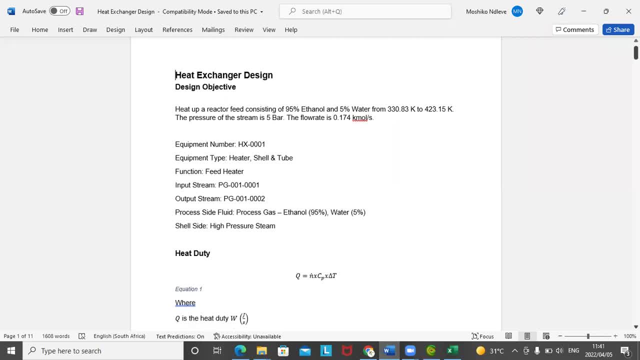 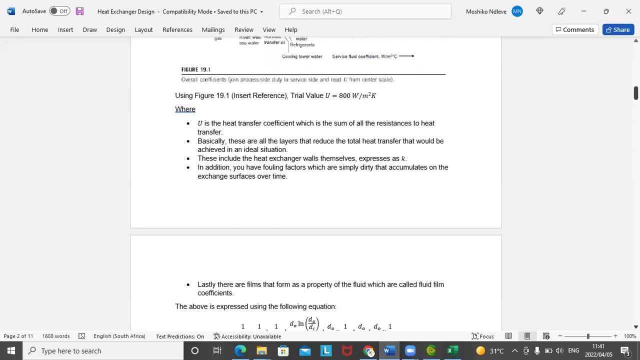 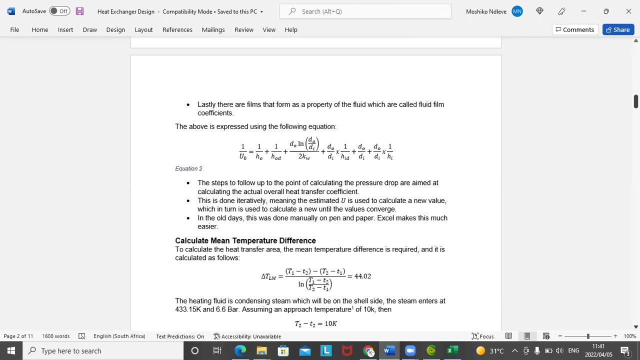 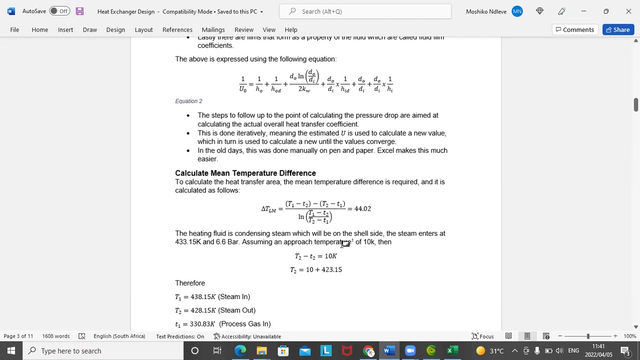 is, before you do anything, you need to understand how approach temperatures work and the difference between counter-current heat exchange and the difference between counter-current heat exchange and what I'm looking for: Counter-current heat exchange and counter-flow heat exchange. So the heating fluid is condensing steam which will be on the 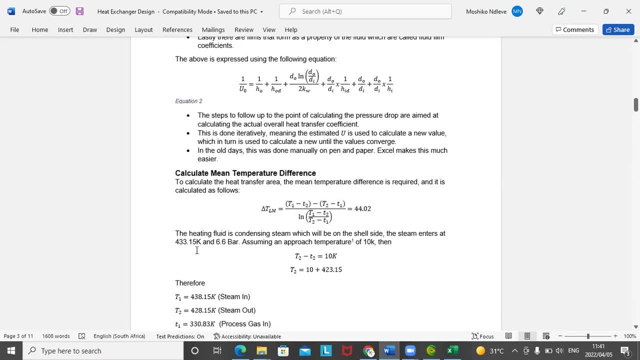 shell side, The steam enters at 433.15 Kelvin, 6.6 bar, Using an approach temperature of 10 Kelvin. then you take the difference between the steam and the cold fluid and you put that at 10 degrees, at 10 Kelvin. What that will then do is it will give you the 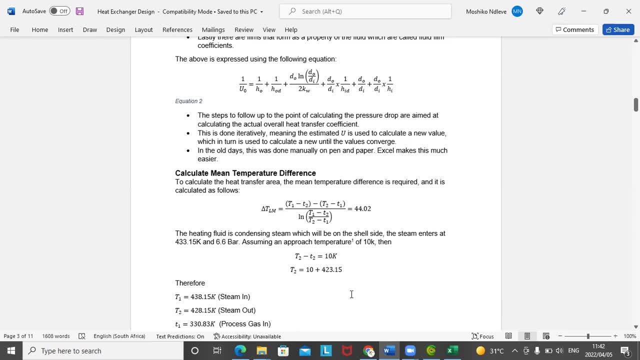 give you the value of the exiting steam right. The other way to do it is especially for counter-current, where counter-current does not have a challenge of overlaying, of crossing, where the overlaying or over-crossing, where the process fluid temperature crosses with the 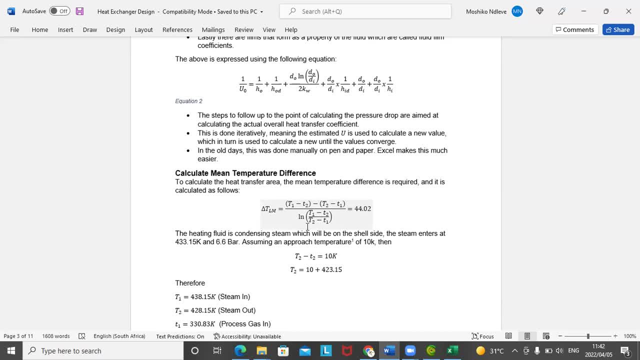 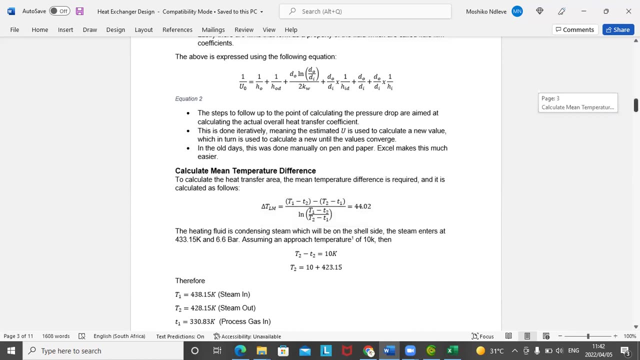 heating fluid temperature. you would then have to look at that. As I said, you need to take time to go through the whole approach, temperatures and how counter-current and counter-flow works right. So what you then get is that your steam coming in is at 438.15 Kelvin. 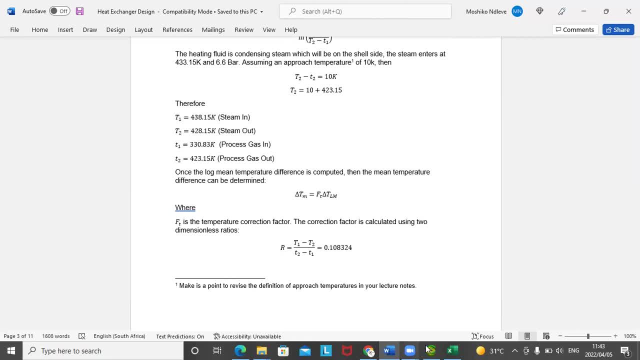 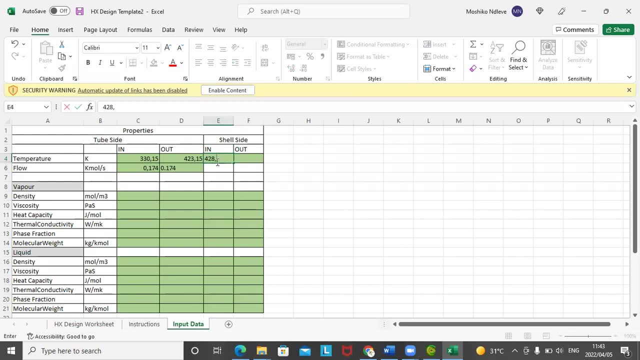 and your steam coming out is at 428.15 Kelvin, So I'll go back and put that into my input data: 428.15 Kelvin and your exiting stream is now this is 438.. So 438.15 and your exiting. 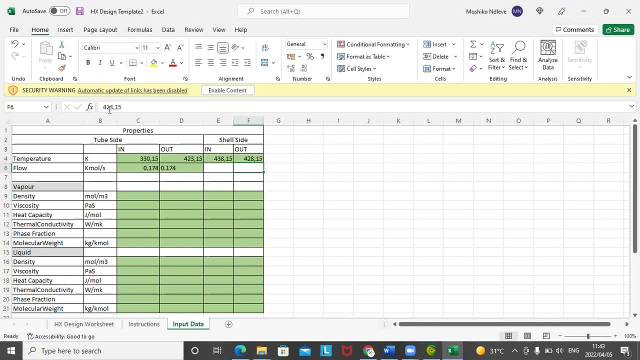 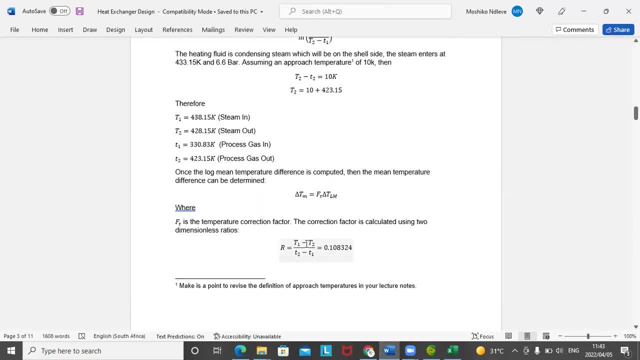 stream is at 428.15 Kelvin. And then I have a few notes for you here and once I've placed that in, it should immediately be able to calculate for you the log Thanksgiving. So I'm going to copy up and paste that into my input drivers. I'm using Combi and rangefront Now how can Icker input it? There's a lot of room on your network. right now, Trying to log-in with some arenas, you can sketch whatever data and most of the timeline opportunities in terms of data development, whereas when you are watching Materials and grandma Sylvia so you're looking at 428, but the data floating is about quarter 13,. 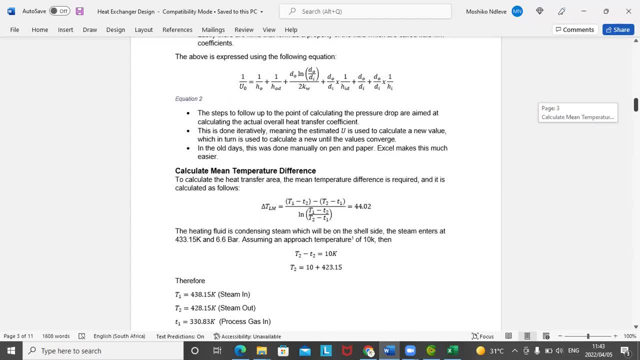 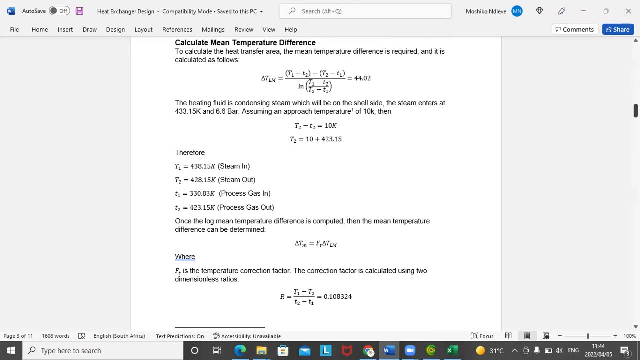 log mean, the log mean temperature and um. so that is the one step. the first step you need to take before you calculate the mean temperature is you need to calculate the log mean temperature. so let's go back to our template and see how far it's taken us on the information we have so far. 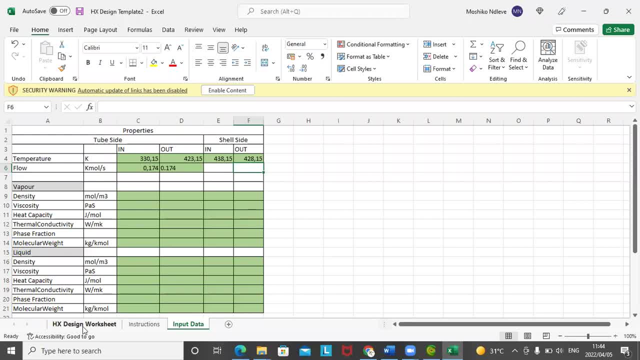 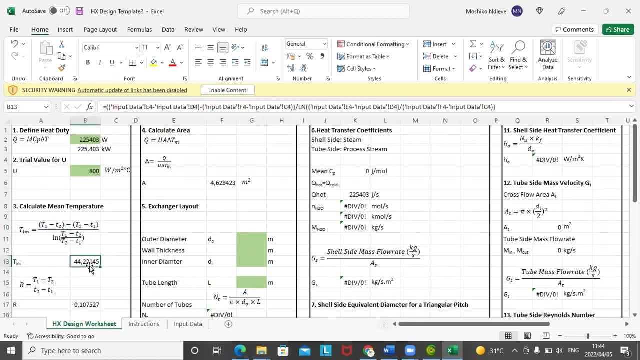 as far as i know, everything should be calculated by now. so let's go back. so, as you can see, because now we're putting our temperatures, it has given us the value for our log mean temperature, or log mean temperature, and that's the formula up there, which is the same formula as we have on the 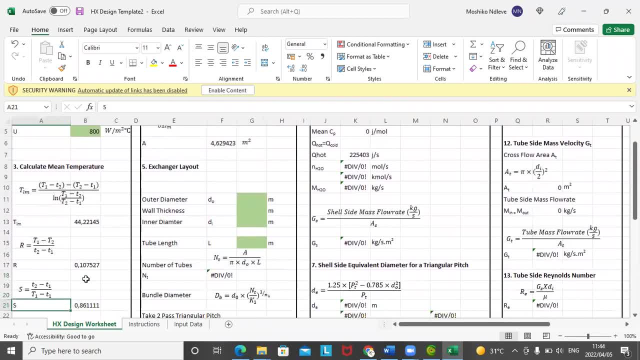 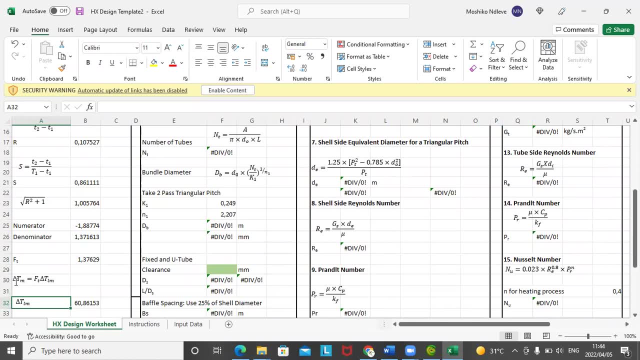 spreadsheet and if you come here from your design textbook, you will see that there are two constants that you need to calculate in order to be able to evaluate the formula for mean temperature difference, which is, which requires you to have a factor which is ft. let's just go back. 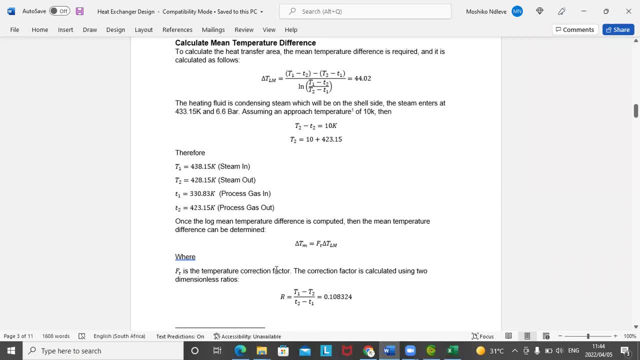 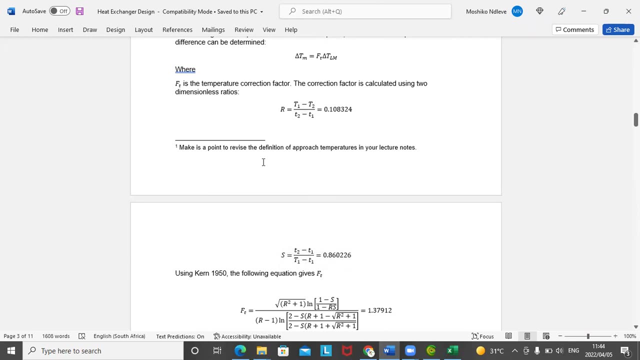 so ft is the temperature correction factor. so, in order to be able to calculate that you need to have these two, these two constants which are given by the two equations here and here, right as again, make it the point to revise the definition of approach temperatures in your lecture notes. 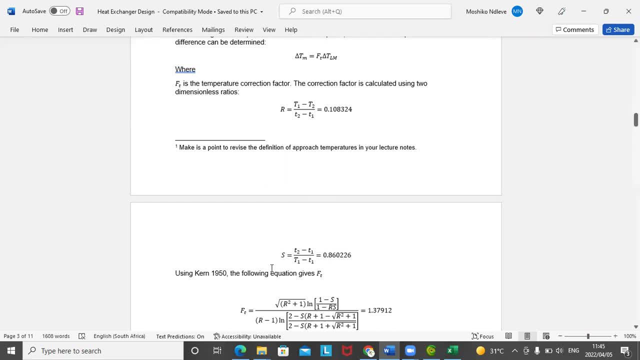 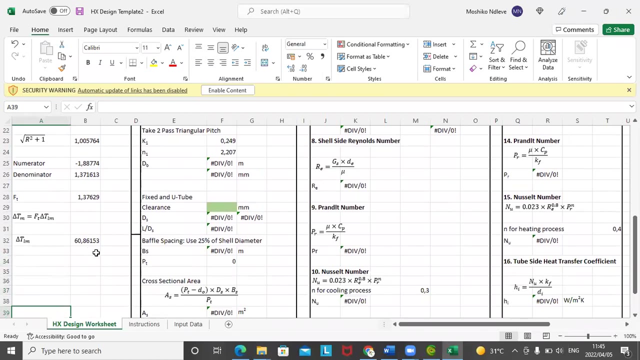 and make it a point to read your design textbook regarding the origins of the temperature correction factor. right, and these are your formulas and, based on the information we have so far, our spreadsheet, as i know it, should be able to take us as far as your mean temperature, which is here 60.85, and this will need to be. 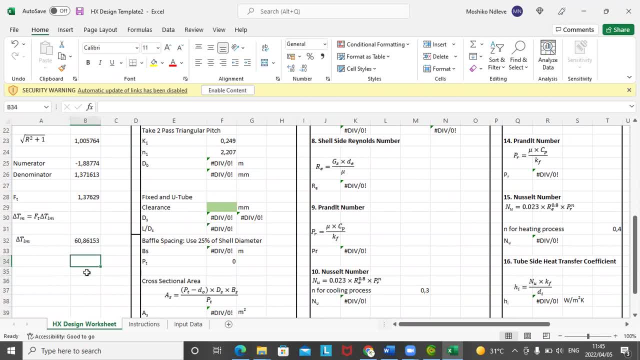 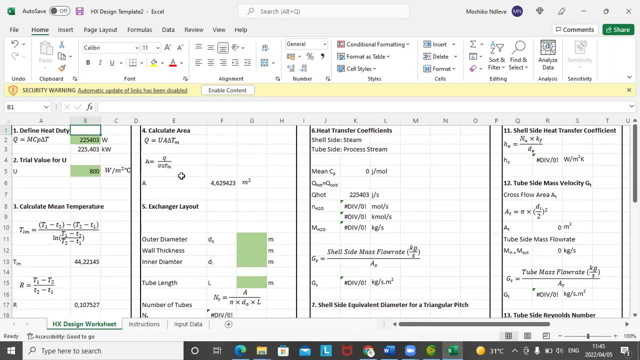 corrected. it still says log mean, but it should be just mean temperature and if we proceed, you will see that we now have all the information we need to calculate your estimated heat transfer area, which is 4.62. now let's go back to our spreadsheet. if you see here: 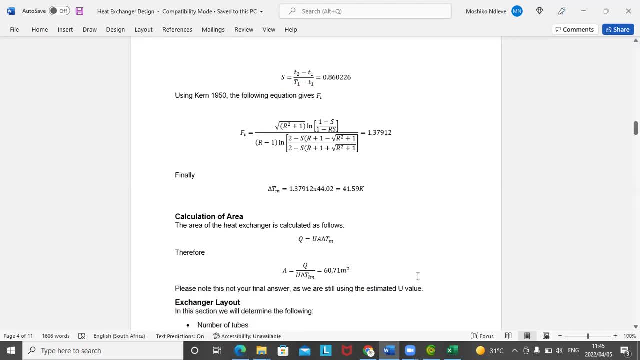 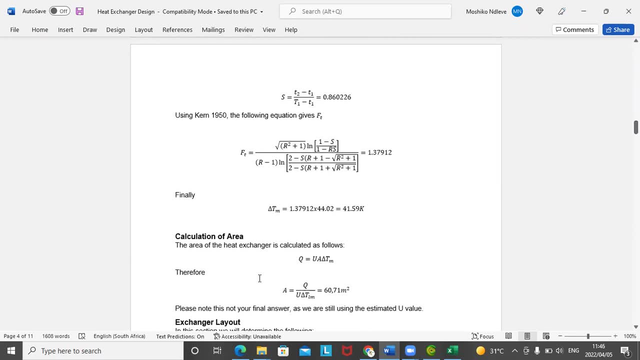 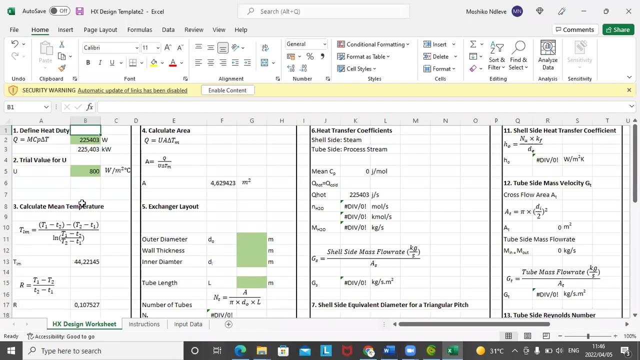 um must be an error somewhere, because that's giving us 60.71 um. i'll just need to review that. but again, please note, this is not your final answer, as this is an estimated new value, so let's go back to the template and see where the error may have come from. 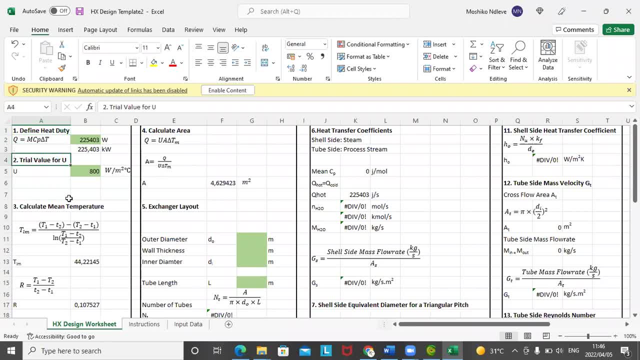 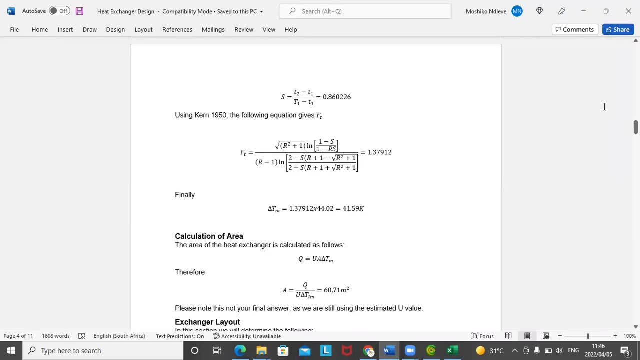 so as if this is an adjusted in fight envelope. usually we ignore these errors which may be, uh, probably told by a chemist or a geologist. it may be the sixteen, so it's a Doncango necessary solution asked to remove all these examples. so let's go back to the template. very should if we put two勢. 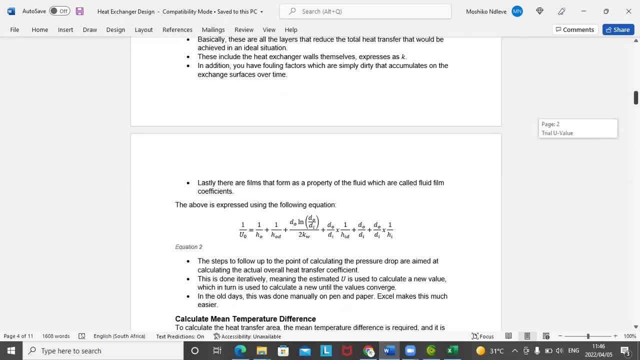 uh, the EC percent. so you got those three grabbed, so to hot, i'm six all. i just wanted to mention that you could put four, maybe. what else do you want to do? like this and everything was added to the front, then we could do like that. but then then here it was our formula, withöd t, which is the, the information collected by the many papers earlier in this video. so if, if you want to show them a good example of why that change is going to be behind this slide, because there's a little. next question, since IPtext, which happens in the 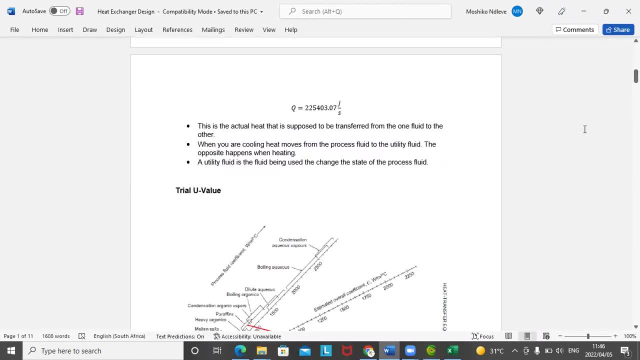 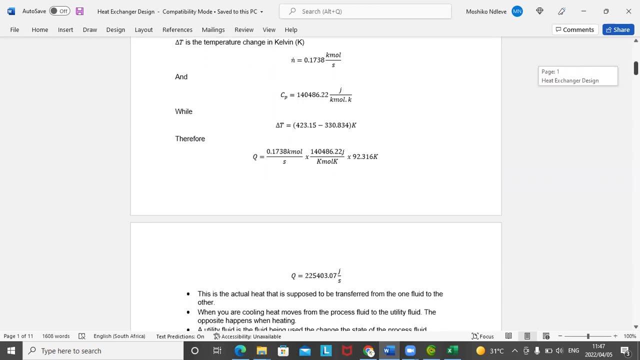 5403.07. just want to make sure that those values are correct. so we've got number of moles, we've got the bbcp, which is one one four four, one four zero four four eight six point one two. we've got the temperature difference. 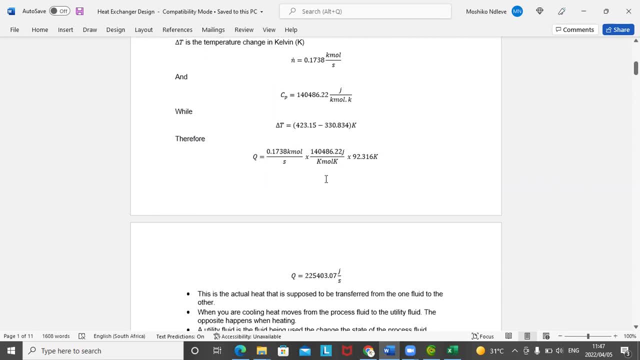 just want to do a quick calculation. make sure that our heat transfer is okay. um, that's not the area i was expecting, hence i'm a bit skeptical. um, it's always good to check your work, um, because numbers never lie at the end of the day. just hold on 1.738 multiplied by one. four zero, four, eight six. 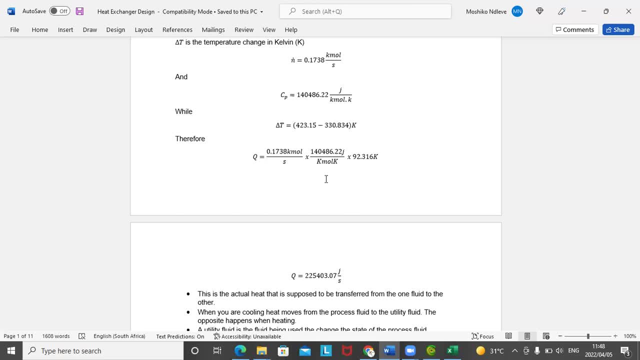 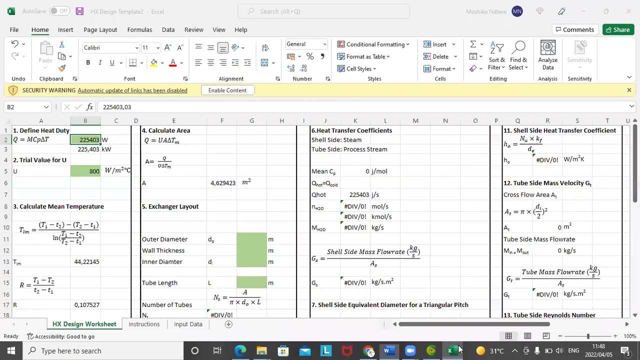 comma two, two, that will multiply that by ninety. two comma three, one, six, that's two point two, five million. so there was an error here. um, there was a definite error here in terms of value. um, this was actually supposed to be: uh, two, two, five, four, zero, three, four, four, one zero seven. 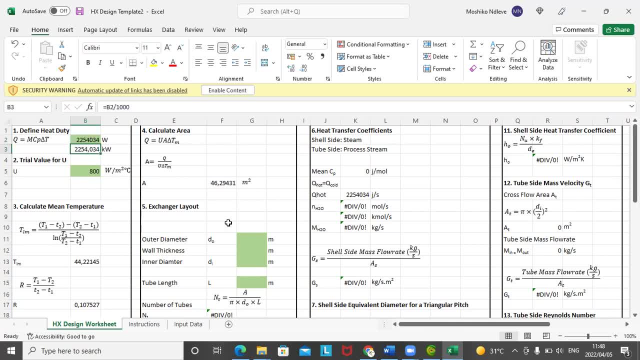 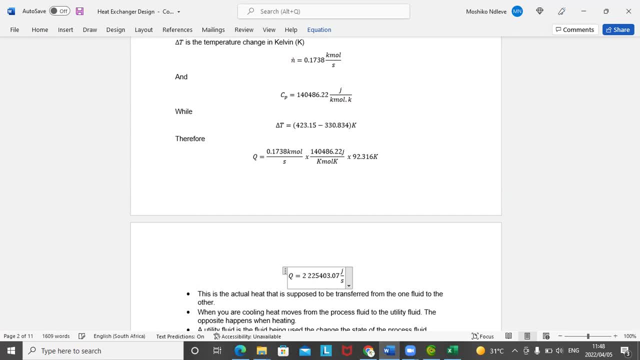 and that gave us. that gives us a starting value of what the six point two, nine which is squared, so we can then go back and correct those values. so this was supposed to be 2.2 million. you must always be careful in terms of how you present your numbers, because that can create an 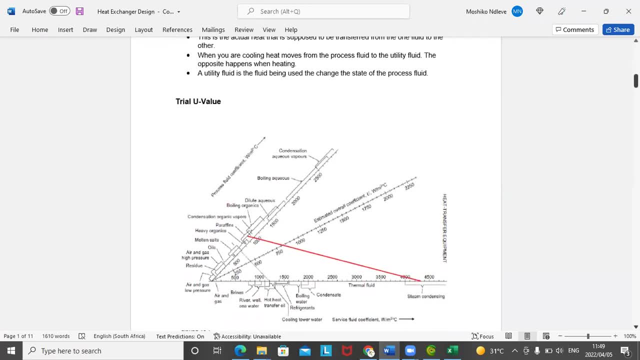 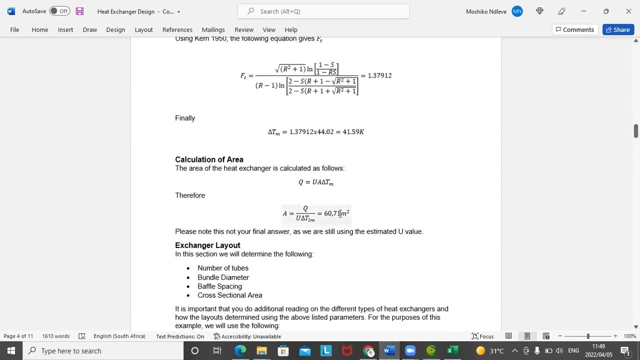 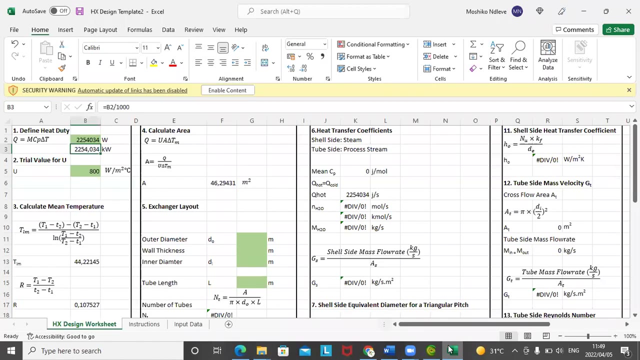 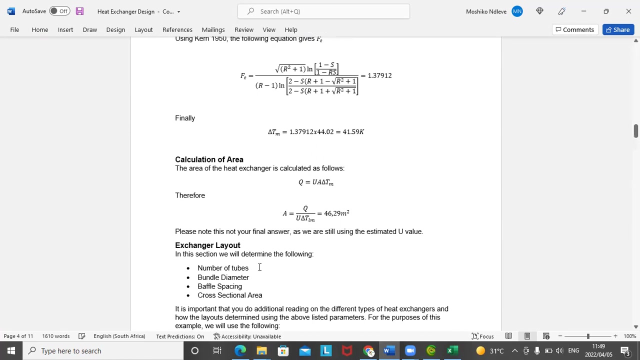 error going forward. so if you go down, then um up. so far, um, our calculations have led us to an estimated, um, an estimated initial area of forty six point two, nine four, three, one, forty six comma two, nine meters squared right, so, um, we can then go back to the old valid, hoping that we can separate all these. 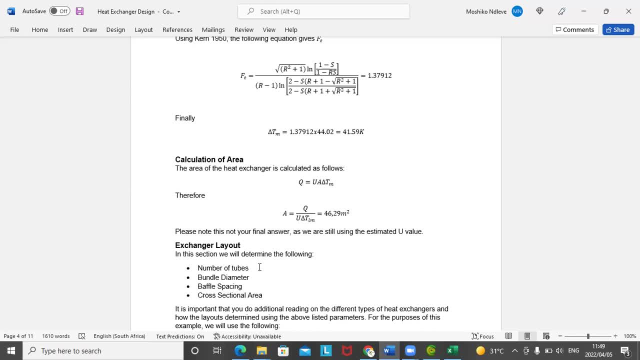 values without extreme correlation. so oh for so good. like um, without having to do any simulation, we are able to get as far as estimating the total area of date exchanger. now you'll see later, when you're doing your plant design, that you'll be required to give, for example, the costing of the 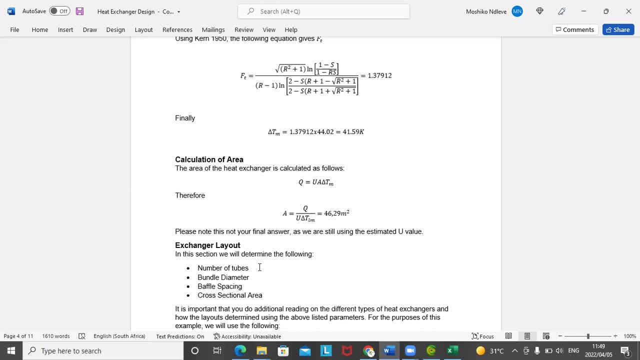 total plant, where you'll find that you only did the. you will need a quick way to estimate your heat transfer area, and this is it, so. this project that i've designed for you here allows you to do that, and at the end of the lecture i will discuss what. 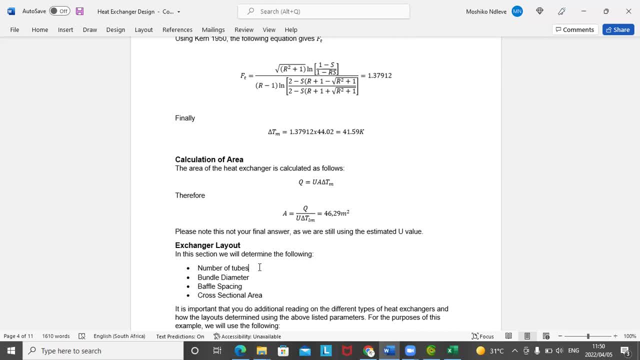 you need to do to get this uh template, because it will be for sale and um. for students who contact me through um after watching this video, there will be a discount on it. however, we will discuss the price at the end of the lecture. so now we've gone as far as completing our area. now we need to 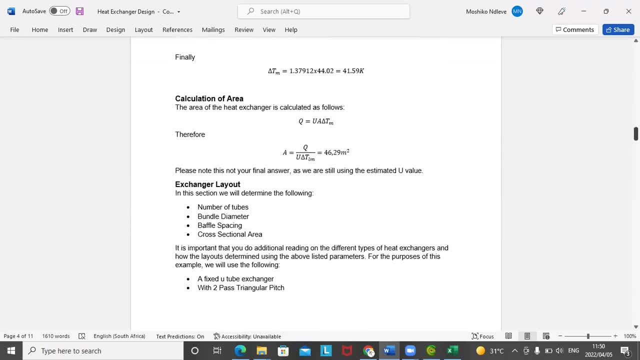 do the exchange and layer, and in order to do that, we need to determine the number of tubes, the bundle diameter, the bevel spacing and the cross-sectional area. now it is important that you do additional reading on the different type of heat exchanges, because the above that we've 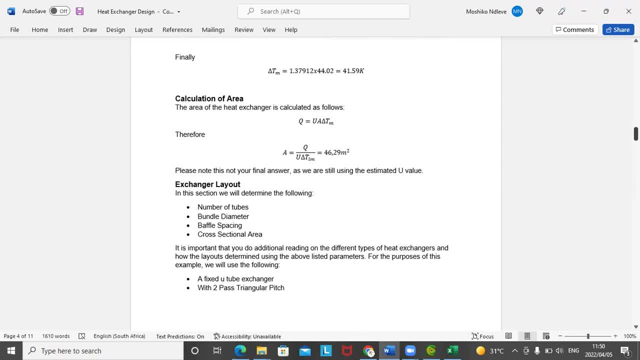 just mentioned now are dependent on the type of heat exchange you are using. for example, in this particular design, we'll be using a fixed youtube exchanger with two pass triangular pitch. now that in itself will determine make a huge difference in terms of how our heat exchanger. 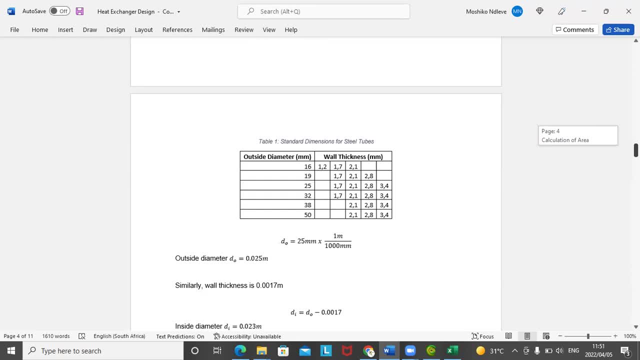 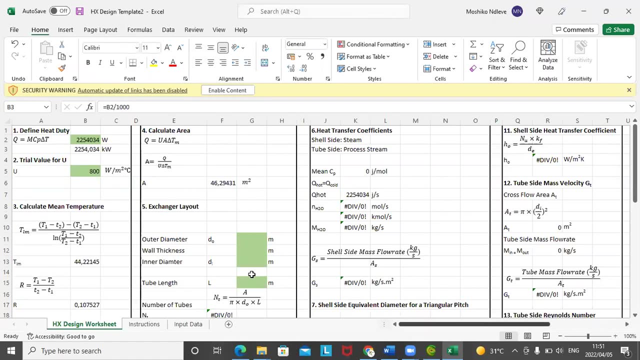 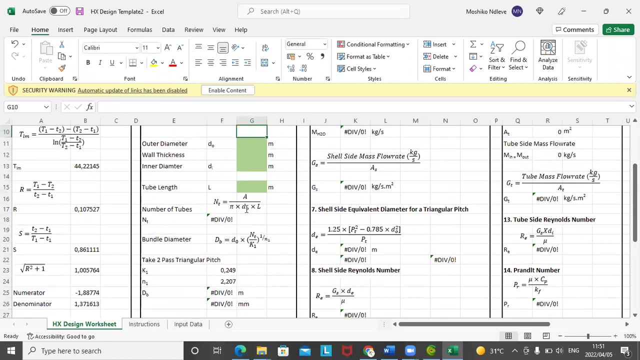 will work. so these are your um dimensions for- for still tubes. so, if you go back to our next step, what we need in terms of our information is what we need to get- our outer diameter, our wall thickness, our inner diameter- and that will help us calculate that tube length right. so, um, oh, no, no, also our tube length, and then what we'll then do. 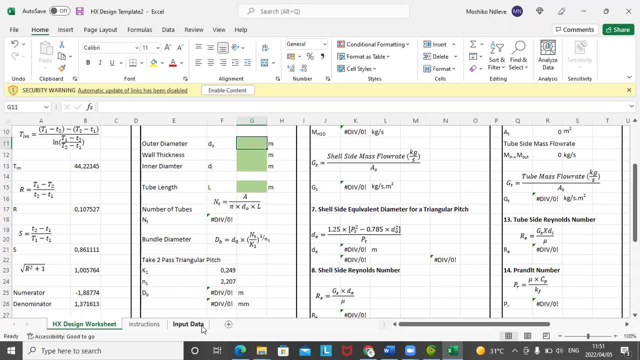 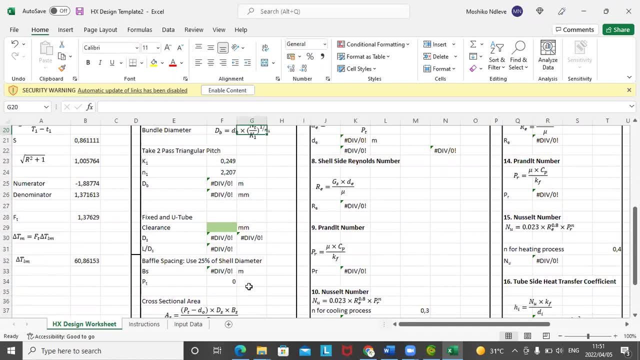 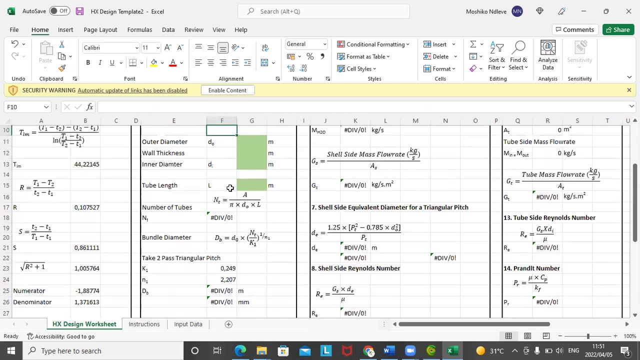 is we'll be able to get our number of tubes and everything up to. by doing that, i believe we should be able to go straight down up to um, up to area once, including our clearance as well. so let's go get that information now, for this one i've already put in. 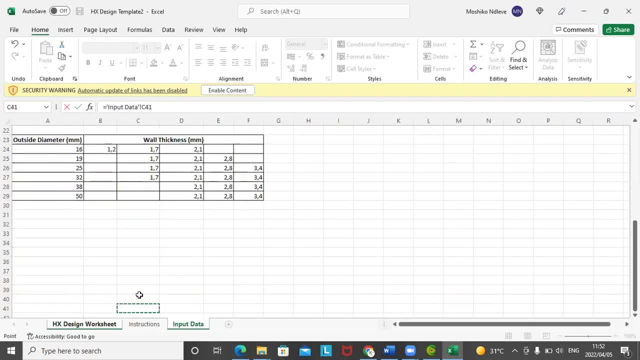 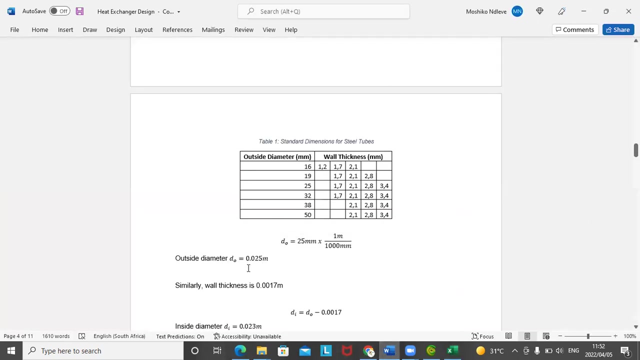 your input data um here. so, as you can see, you've got the wall thickness in, in, in in millimeters. so it first wants um outer diameter, which means, uh, if your outside diameter is 16. let's see what we chose for this particular design. we said our outside diameter was 0.025. 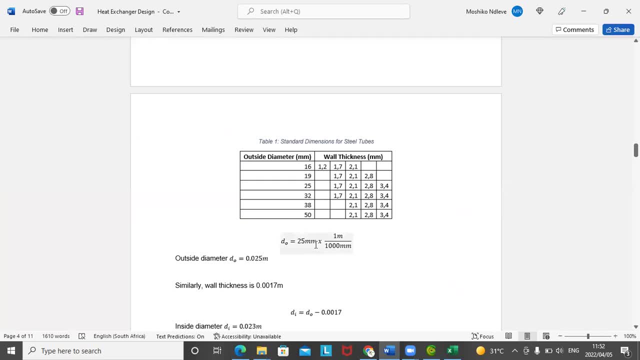 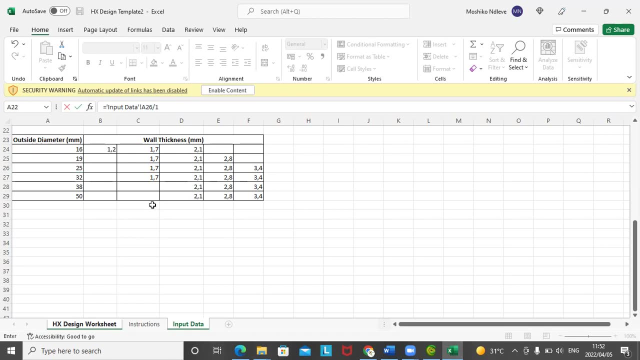 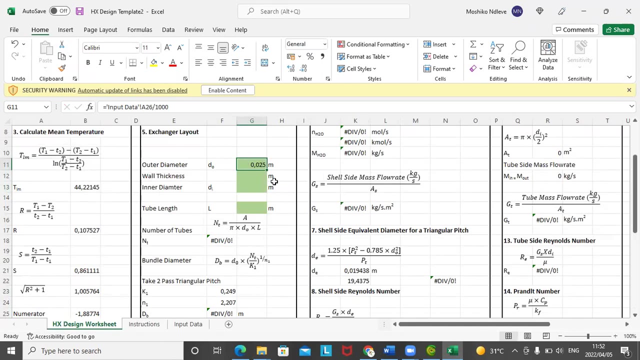 and you need to do that uniform version as i can to make sure that it's fine. um, so you need to divide by a thousand. so we'll do that on the spreadsheet. we'll take 25 and divide that by a thousand, and now we'll have our, our, um, our uh, diameter, and then, if you go back to 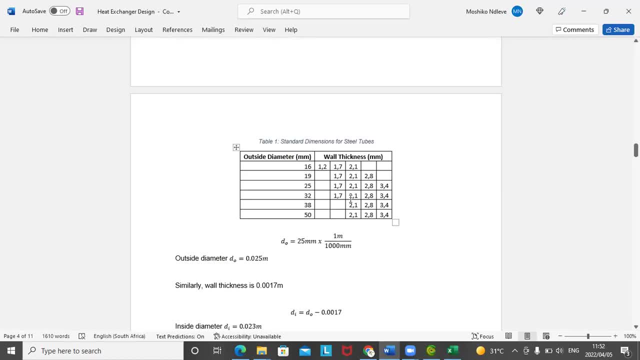 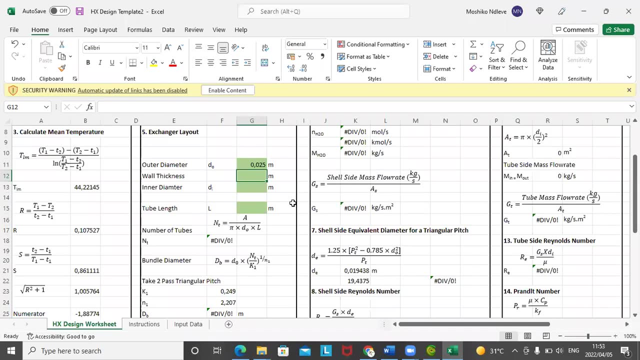 the first same table. it will tell you that if you are using 25, then your wall thickness is what is 1.7, right? so if your wall thickness is 1.7 mil, then what you need to do is: i can you go to your wall? 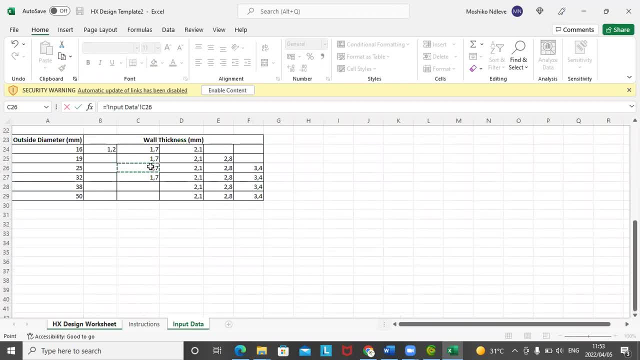 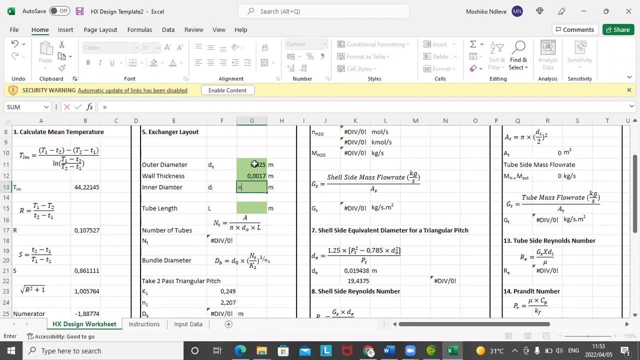 back to our table 25. you divide that by again a thousand. it's important that you don't forget your conversions. therefore, your inner diameter will be your outer diameter. subtract your inner, your, your wall, your wall thickness, and now you have your outer diameter, your inner diameter. 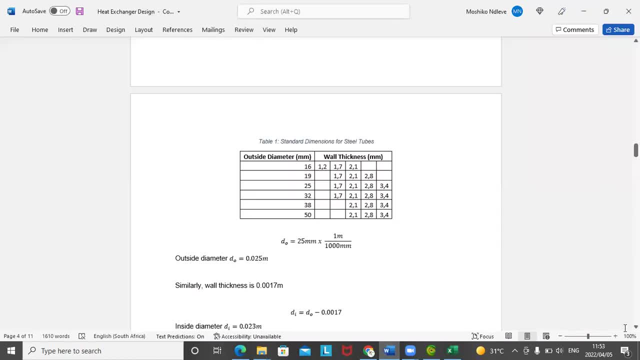 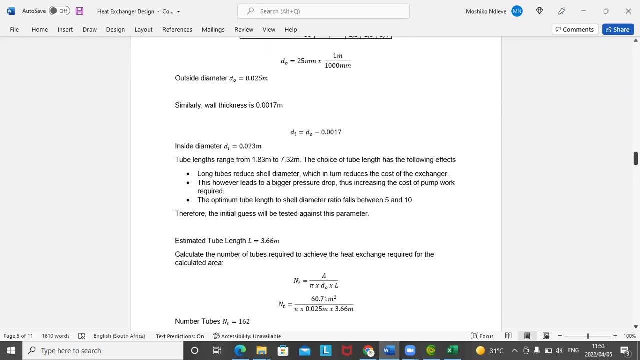 now tube length. um, let's go to our nodes with the tube length. what we did was, uh, the range starts from 1.83 meters to 7.23. again, this is, this is in your textbook, right. and then the choice of tube lengths has the following: 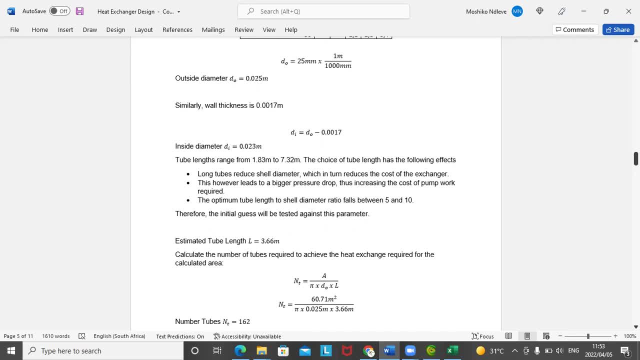 effects. now, long tubes reduce gel diameter, which in turn reduces the cost of the ink exchanger. but that will obviously permit the cost because, um, this will lead to a bigger pressure drop. that's increasing the cost of the pump block. so design is a given. so your optimal tube length, shell diameter ranges between 5 and 10.. and you'll see later. 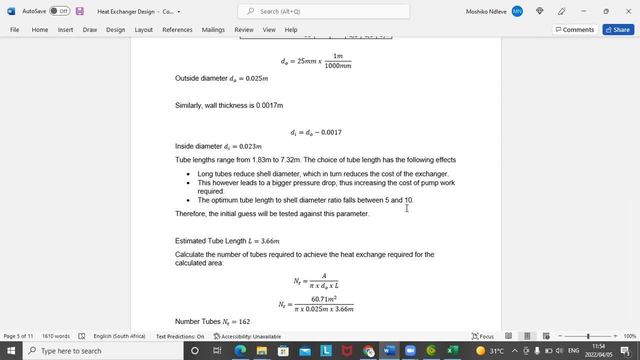 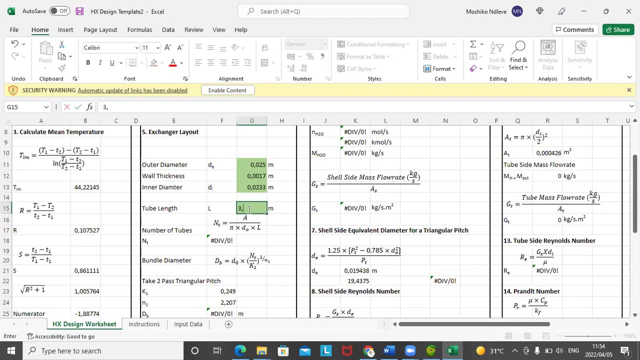 we'll use this range to be able to determine whether or not our heat exchanger is within range, and we will take our estimated tube length to be 3.66, which is between the two values. now let's go back and punch that in. so now we'll punch in 3.66. 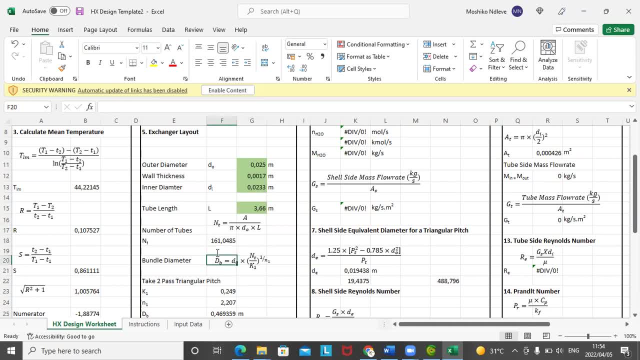 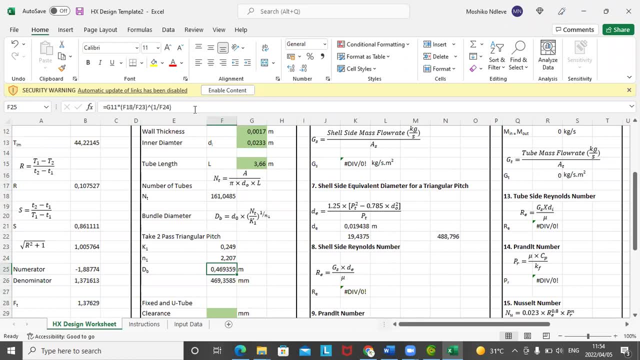 and you'll see it will immediately give us your number one, number two, number three, number four, number five, number six, number six, number six, number seven, number seven, number six, number six, number seven, number six, number six, number six, number seven, number six, number six, number tubes. immediately populate your bundle diameter. and once you have that, because everything up to 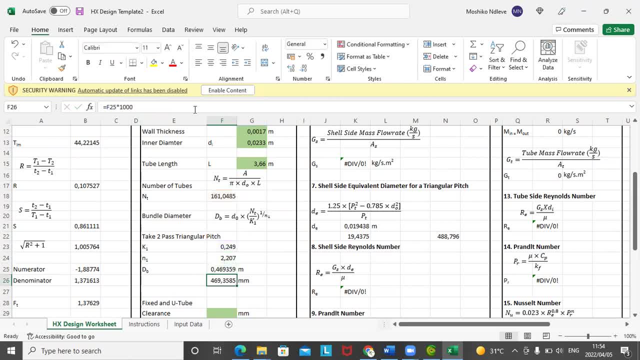 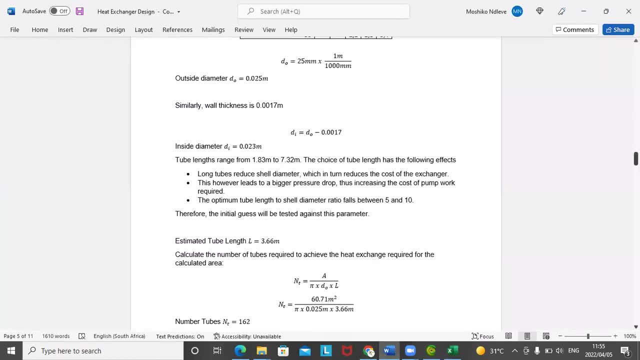 here depends on the information that we've given upstairs, and immediately after that, you'll see that you'll be required to provide a clearance. now let's go back to our our notes. so the guideline- this is a design document- is designed in order to be able to take you through exactly 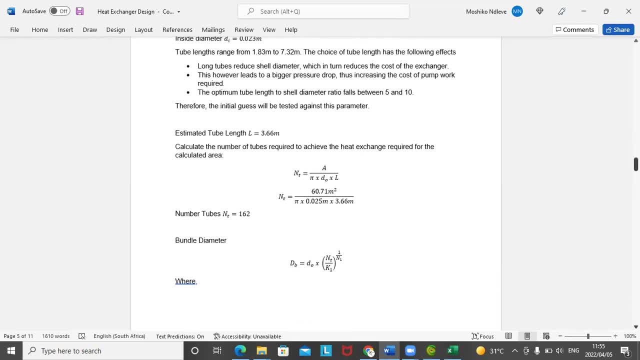 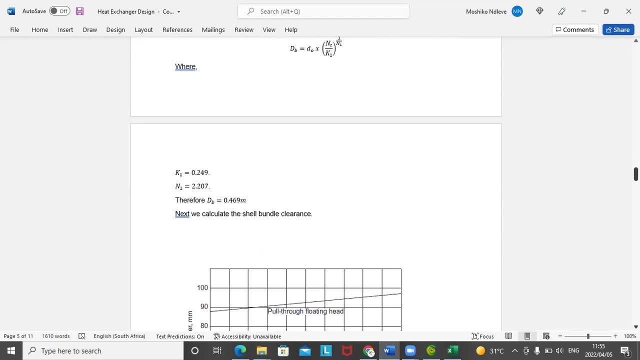 what you need to do and how you do it. um so, by by, it is used to do just all the several disgusting things material here. but by the time you finish studying this document and practicing how to do, uh, the actual design, you will be able to do your own design, no matter the type of feed exchanger you use, because the methodology is. 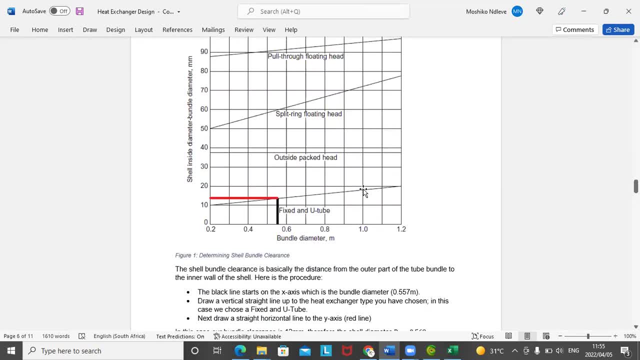 almost the same for all of them and no matter, your, your substances again. so this is how you determine your bundle, your bundle um, your, your clearance. so what you have at the bottom is: can I bundle diameter? and you have your shell inside diameter right now. if you go back um what are? 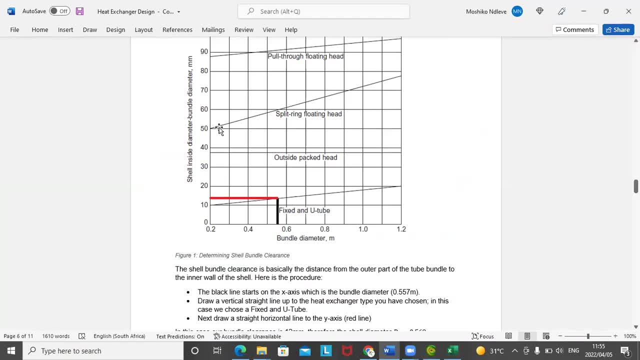 we looking for, looking for the clearance. so what you then need to do? so this is your clearance: shell inside diameter. so that's your clearance, right? so? so, shell inside diameter to bundle diameter. so that is the clearance we're talking about. so what you then do is you take your bundle. 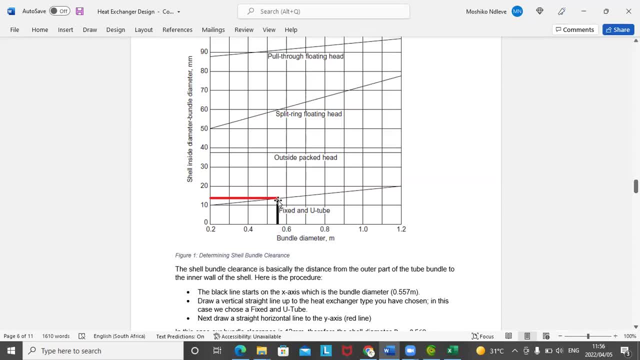 diameter, which you already have, move in a straight line up to the fixed and youtube- and that's the one that you said we're using- and then you go in your straight line up to your shell side, inside diameter to bundle diameter and, as you can see, if we're moving from 10 to 20, that should be sitting. 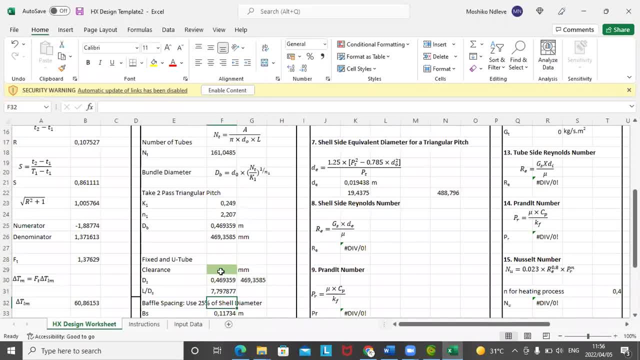 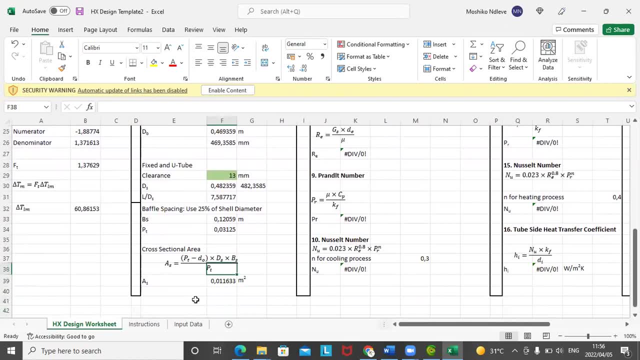 at around 13- 14. so we come back and then we input 13.. once you've done that, you'll see that automatically your spreadsheet will take you as far as your cross-sectional area, and if we go back up here, you'll see that we are. 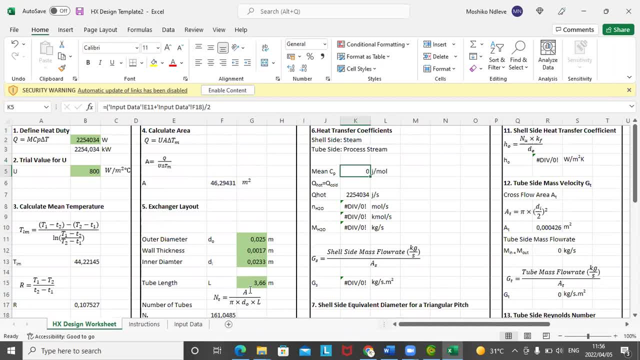 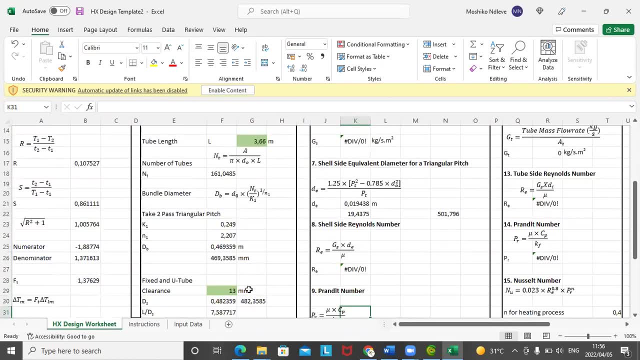 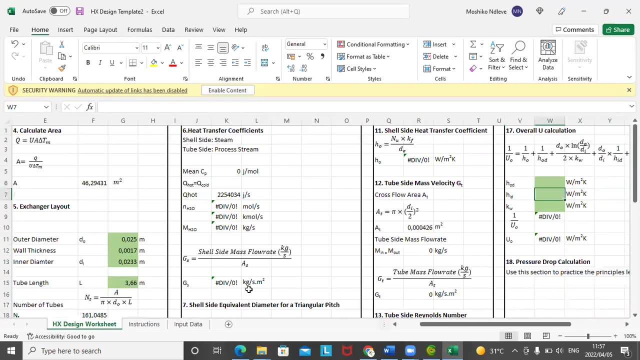 almost on our way home. now. here's the problem. now we're almost done um with what we've included so far. your spreadsheet should be able to calculate everything else in um, in this, in this um, in the scenario, uh, up to where i've highlighted in green: the able- it's not able, the reason it's not able. 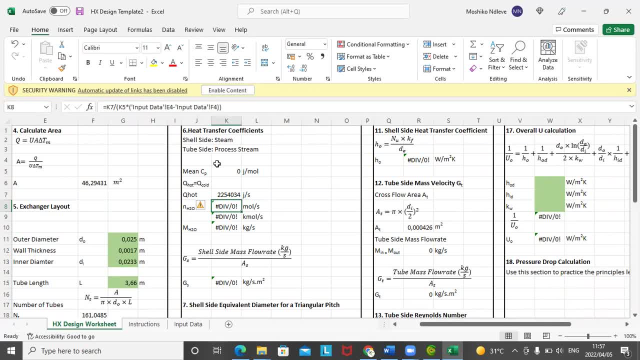 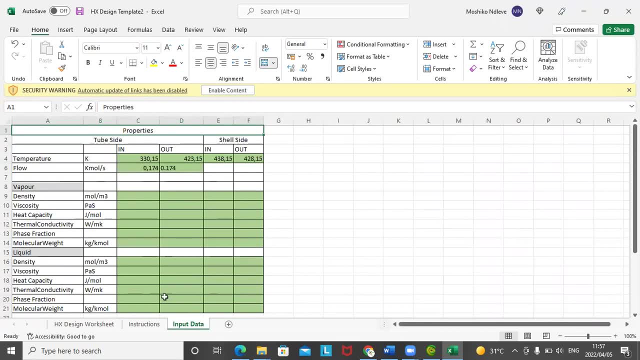 to do. that is because you haven't inputted your what? you haven't included your process information, so let's go back to input data. so now we need to fill out this whole, this whole section, in order for us to be able to do what? in order for us to be able to complete our simulation. right, not our simulation, but our heat exchanger. 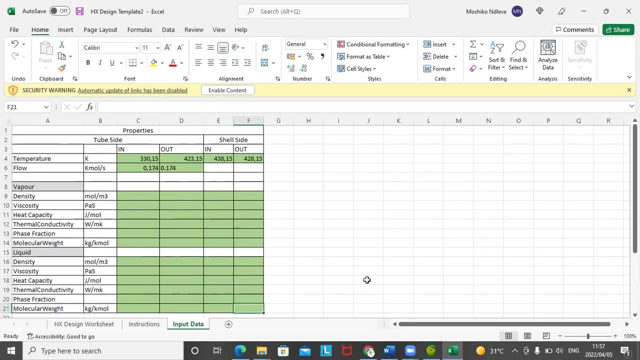 design. apologies for that. okay, let's go. so, as i said, um, this can be done manually. you can get information from, for you can go to tables like your queries um your paris handbook, campaign engineers handbook. you'll get all this data that you need. uh, you just need to make sure that you're. 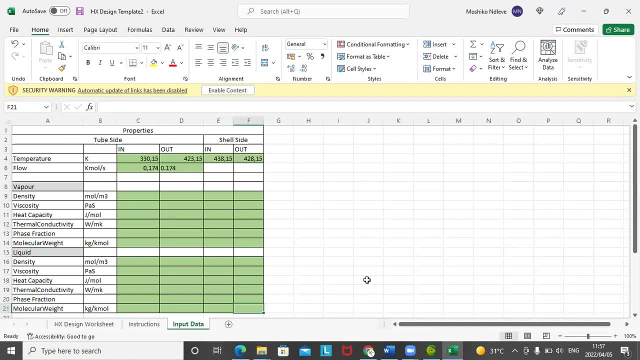 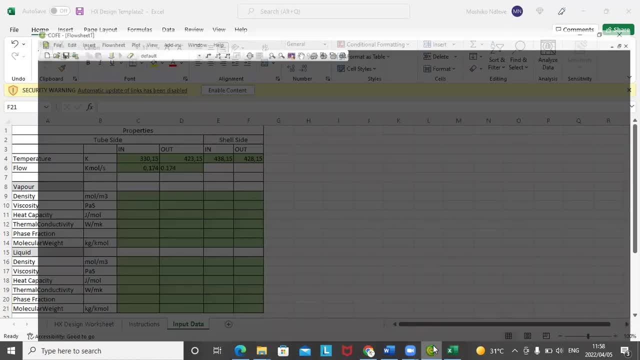 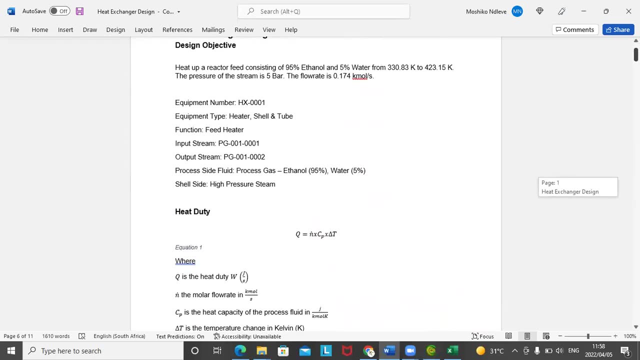 working within the right temperature ranges. otherwise you can use a simulator. so let's get started. um, what i'll do now is i'll go to coco, and we just need to remember what the dream was simulating. so i'm just gonna shoot back up. um, and it's 95 ethanol and water. so if you've used coco, 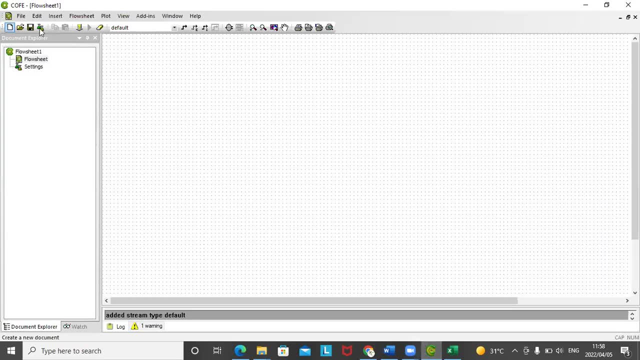 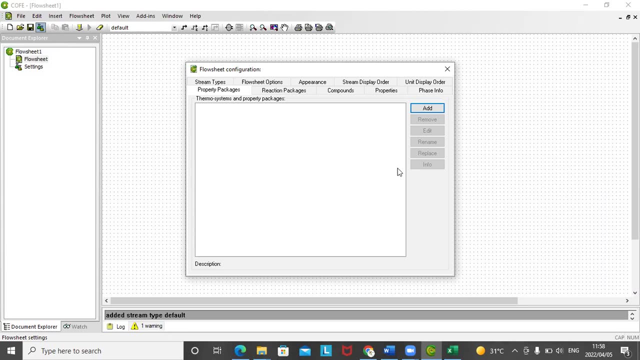 before i won't dwell too much on this. we do have a, we do have a a cost on. we do have a video on the on youtube, on our youtube channel, that deals exactly with this. so please go there if you're still a bit rusty on coco, um, and, of course, don't forget to sign up. so i'm just gonna do it quite. 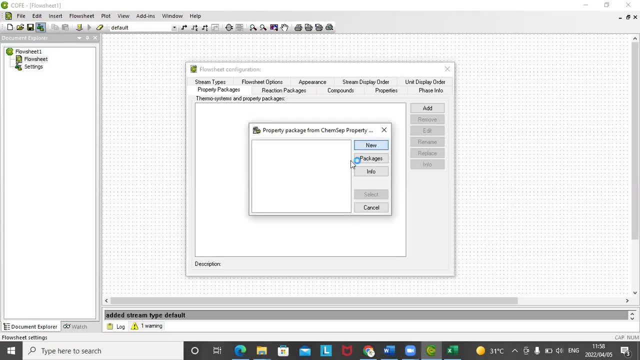 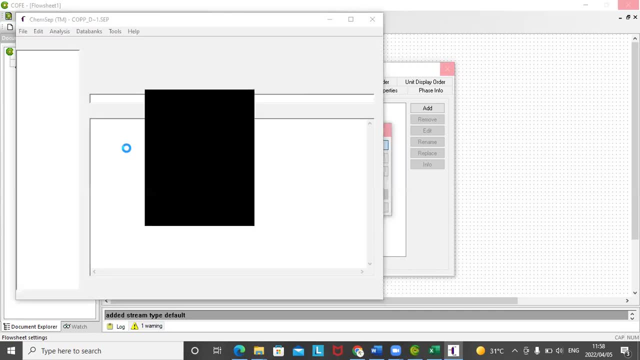 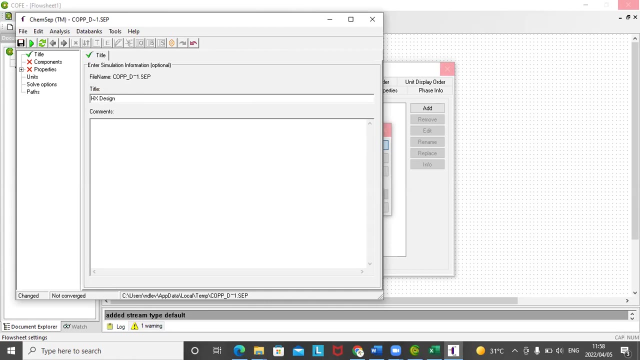 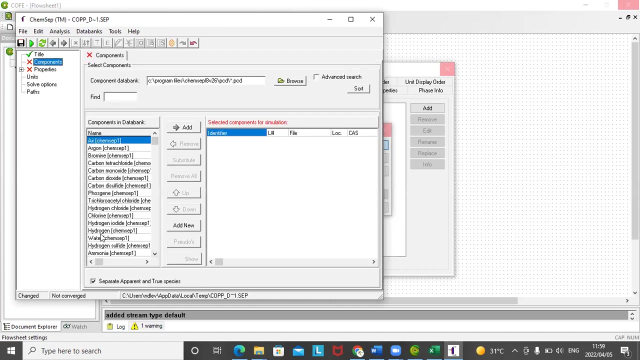 quickly, um, just to show you how we get the information. um for an in-depth lecture on this, you can go to the coco website um to check it. so, um, you can give it a title and we can call it our hx design. and then components. we will need what? just water and ethanol. there's our water. 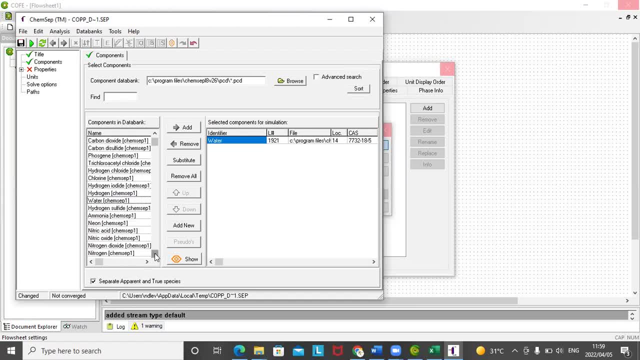 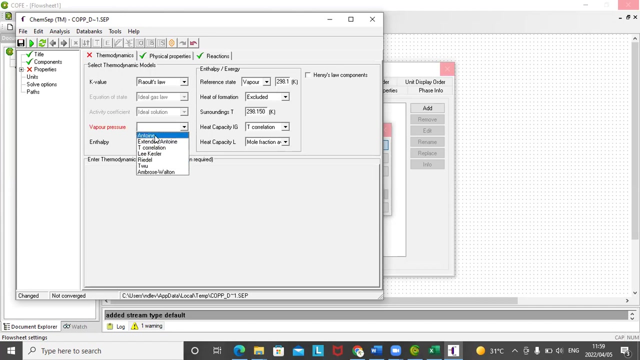 let's edit and we need ethanol as well, and then, um, from there we go to properties. then you just need to choose the right way. um, so, uh, let's just go to the pilates facilities. uh, ibibs uhวก funcion. uh, i am a cyber pod which works really well in the web. uh, the dta drawing kunne. 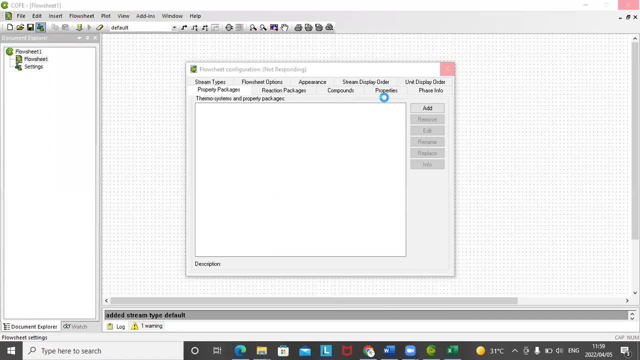 we just need to also make sure, um, our data is impacted, right? so if the perfect flying model that is the same uh video model, then that's good. so, uh, again, for a better understanding of this, go through some of our simulation videos. it'll explain to you where to get the symbol dynamic. 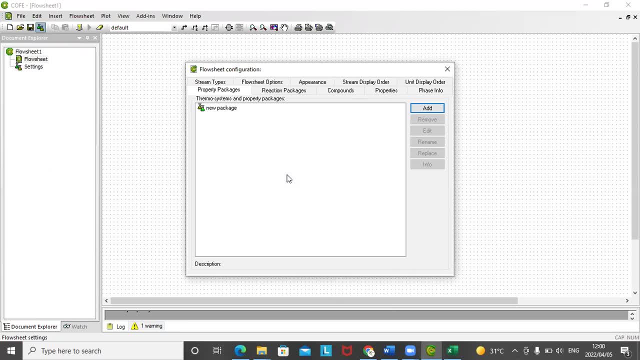 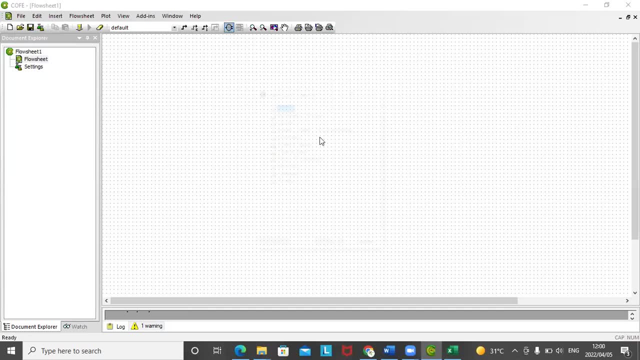 Feth is the first heat exchanger design. It was at Feth we had to estimate its properties. So let's put in a heat exchanger. So again, we're gonna simulate what we're calculating manually that side, so that we understand the process conditions coming in. 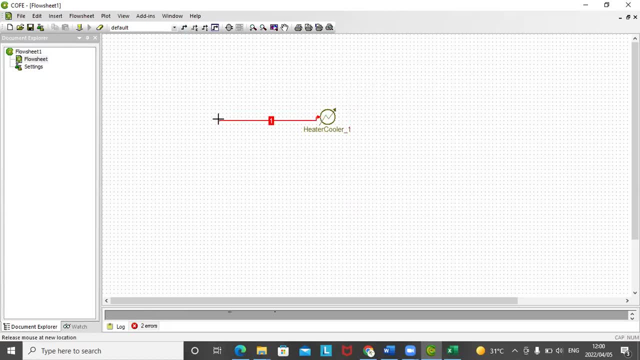 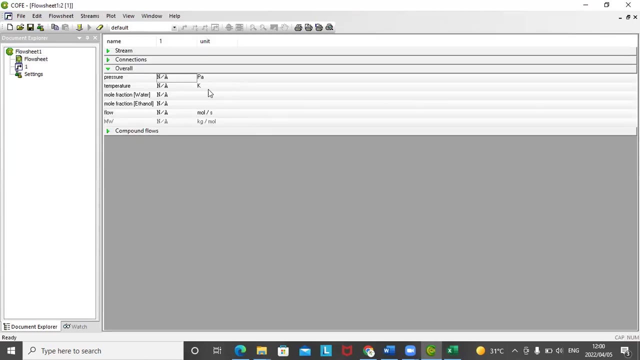 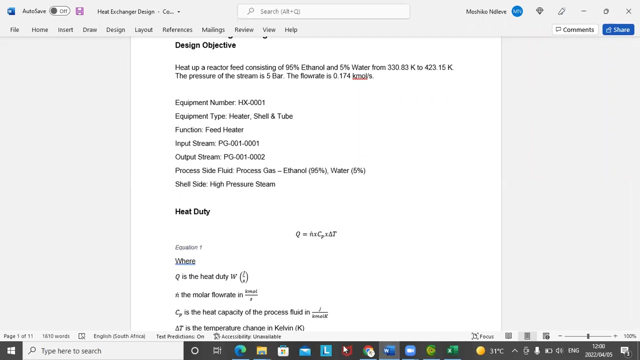 and leaving the heat exchanger. All right, and what needs to come in here is: we said we're operating at five bar, so I'll change that to five bar. Five bar. our stream is coming in at 380.83.. Let's go back to the simulator. 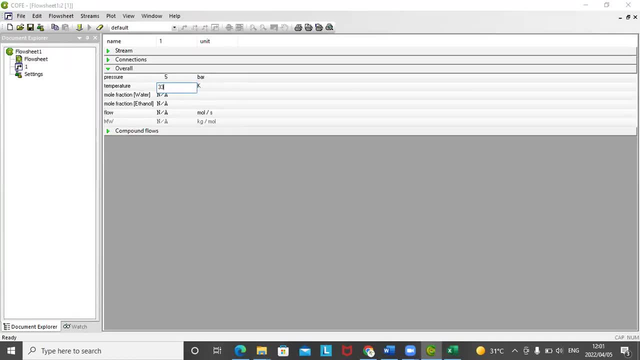 Let's go back to the simulator. at 330.83 Kelvin right And the most fractions we have syntax error. it means it's not using the same format. So it's sort of the value We said we were coming in at 330.83, 330.83.. 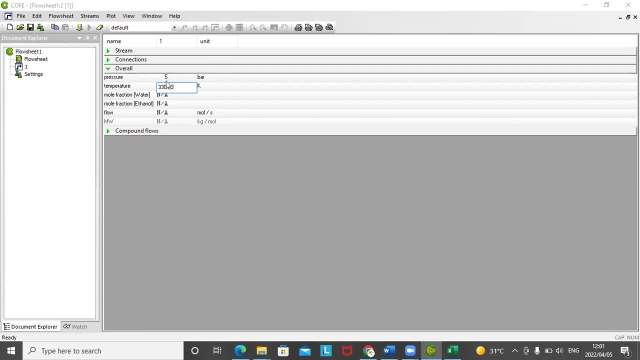 330.83.. Excuse me if I'm rather moving head first. I'm recording this on Zoom. So, as you know, Zoom has a 40-minute limit. So I want to make sure that we cover as much as possible At 5% water, and let me just confirm that. 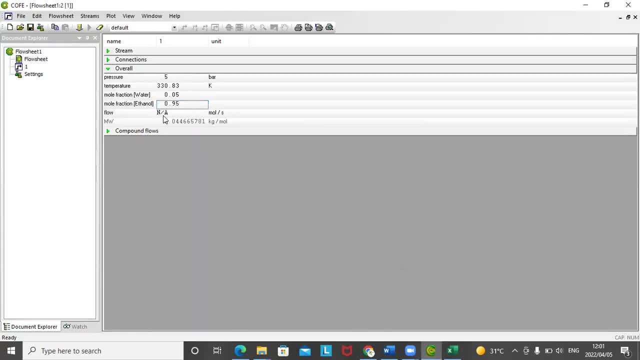 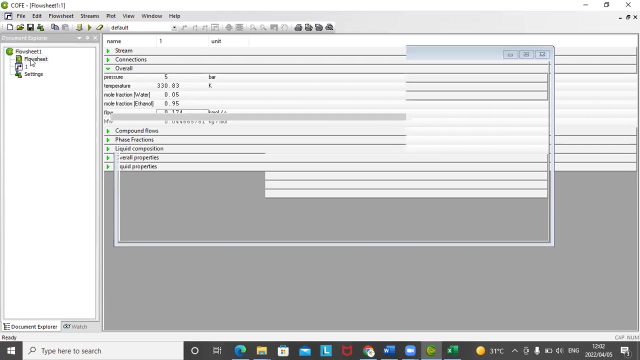 And 95% ether that's given us. And then our flow rate was given in kilomoles per second And that flow rate was 90%, Not 0.174 kilomoles, not 0.174 kilomoles. And then we know that our heat exchanger 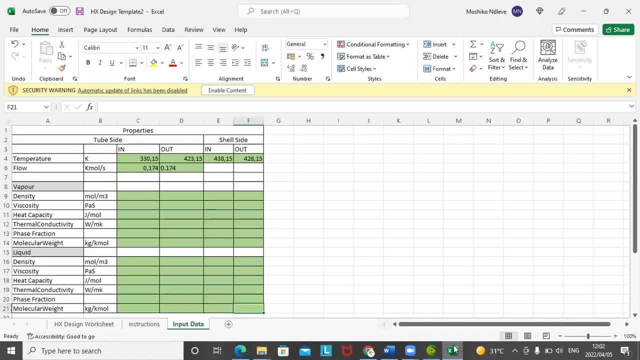 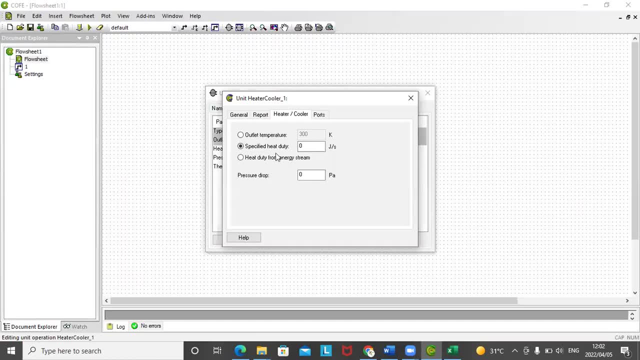 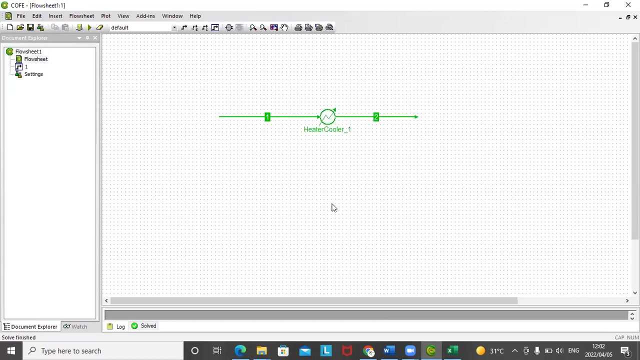 we need to heat up the stream to 423.15 Kelvin. Need to heat it up to 423.15 Kelvin, So our outlet temperature will be 423.15 Kelvin. Close that, close that and we run it Now. once you run it, you'll be able to have all the information you need. 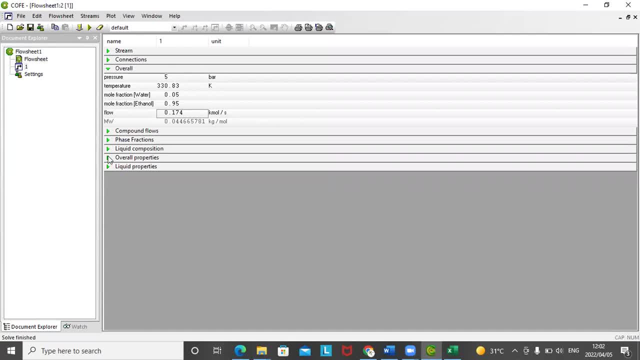 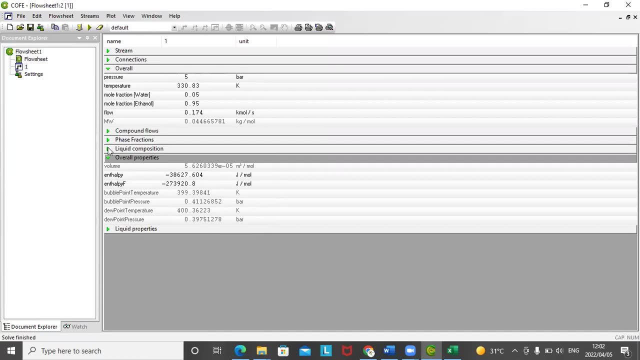 Because if you double-click on that, you'll see you've got overall properties where it will give you the enthalpy and all of that. But then you also have here where the incoming stream. first of all, you need to check The incoming stream. first of all, you need to check. 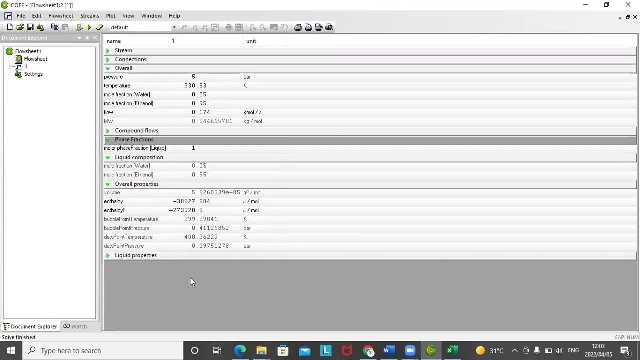 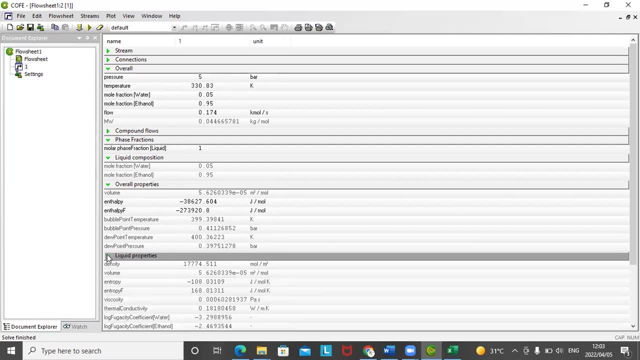 The incoming stream. first of all you need to check The incoming stream was fully liquid. So if it's fully liquid, it means the information you have will be on liquid properties. So if you drop down liquid properties, you'll now be able to get your information. 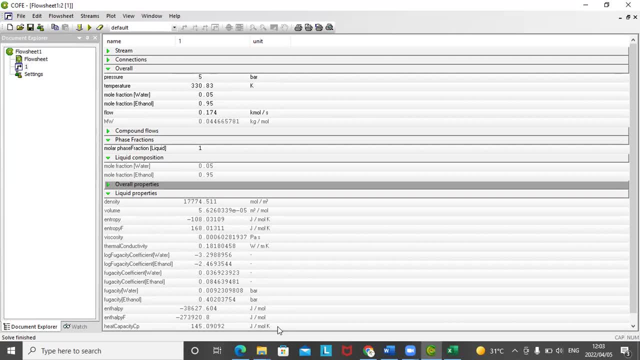 Just a few things that you need to make sure your units have to be similar. So make sure your viscosity is in pascal seconds, Make sure that your- let's go down- your CP is in joules per mole, because that's what we worked with initially. 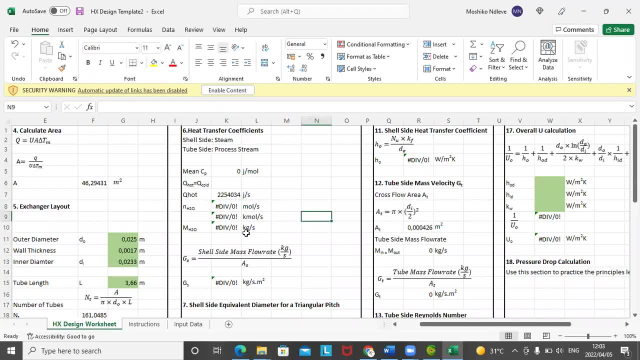 So what we can do to check that is, if you check everything is in kilomoles, let's see initially. So we set the CP here to be in joules per moles, So it's important that you use joules per moles on your CP. 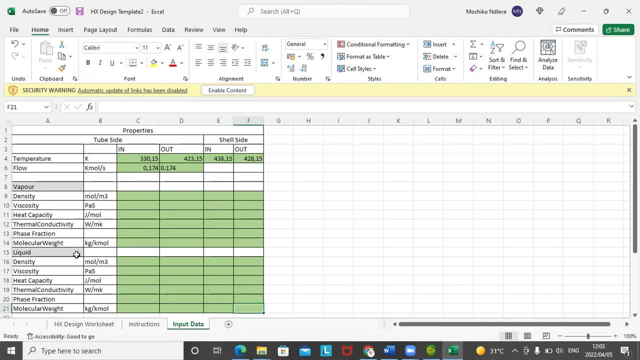 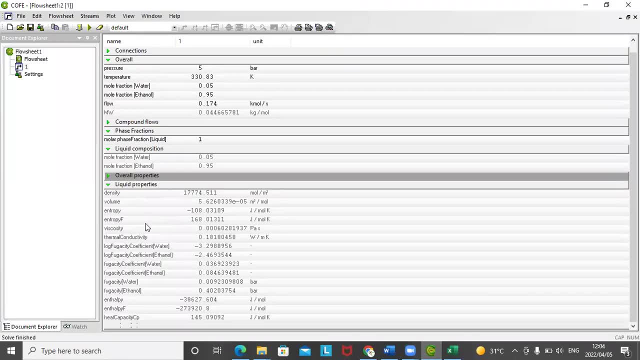 So let's go in, let's put in our data. Oh, already, the spreadsheet shows you what units you should be using. So follow the units as they are on the spreadsheet. So, first thing, we'll pick up our density. So our density here happens to be given in moles. 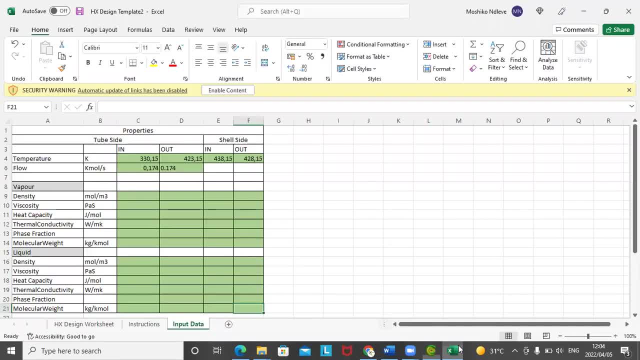 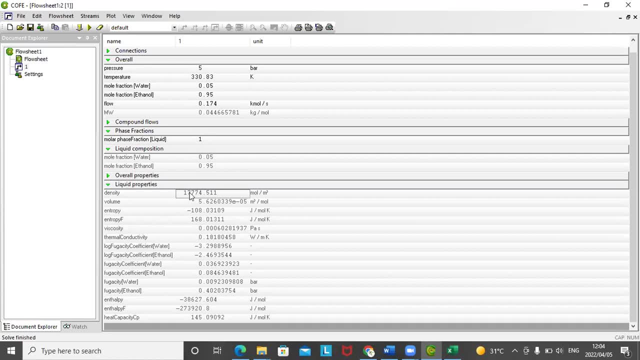 moles per meter cubed. We want it in moles per meter cubed, So that's the right value. So you can. it doesn't allow you to copy and paste, So let's just write them down. Let's see if it doesn't allow you to copy and paste. 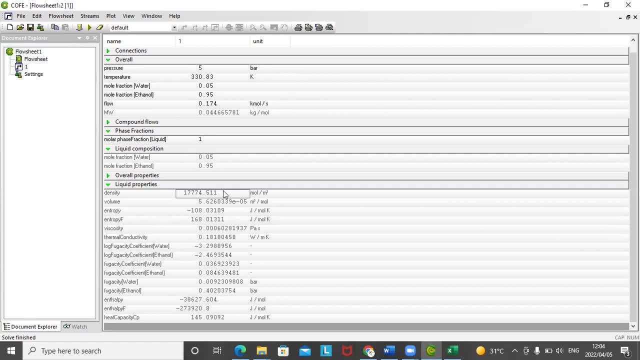 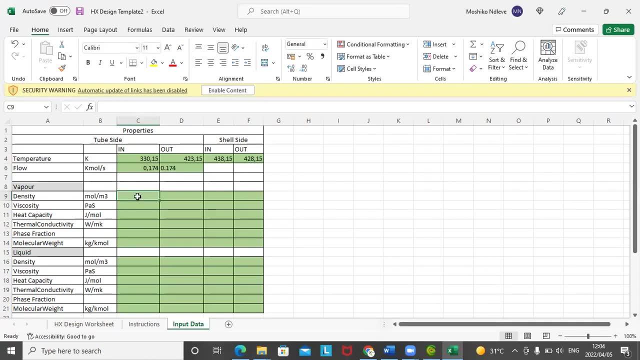 It should It doesn't? So 177.. That's the first value, 177.. So let's be careful not to put that in the wrong place. It's coming in the in the 13774.51.. That's our density. 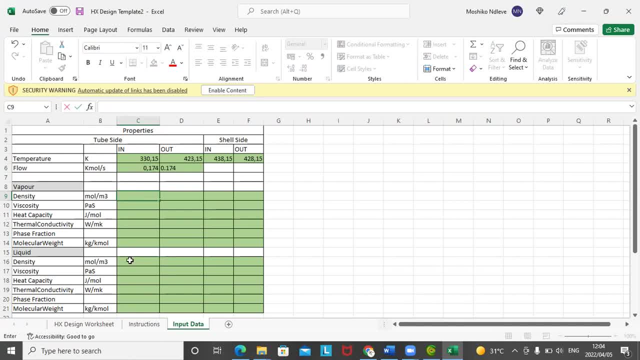 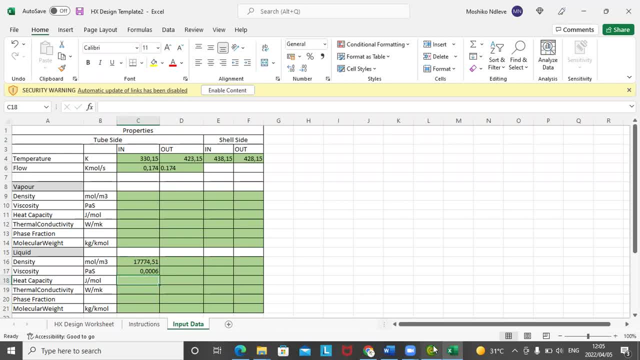 4. 4., 4., 4., 4., 4.. 0. 0. 0. 6. 0. 3. 06.. That's our viscosity: 0. 1. 2.. 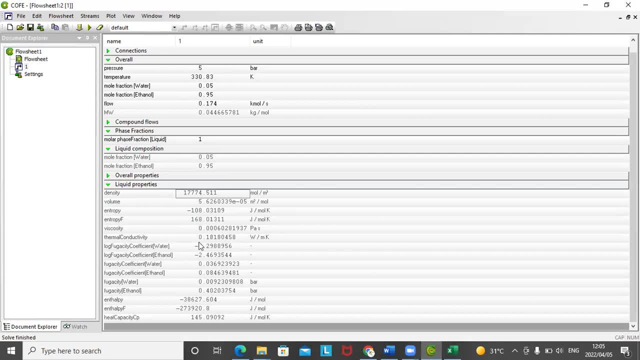 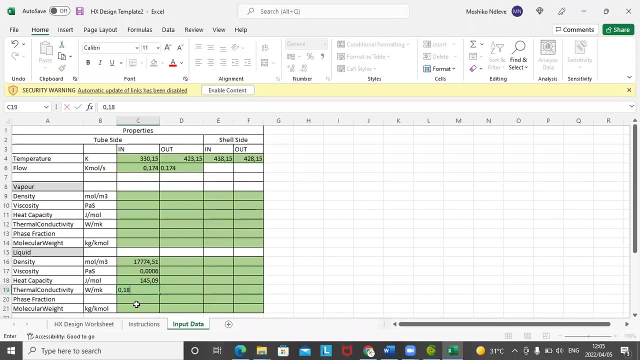 3. 6.. And our heat capacity? Our heat capacity, down here It's 145.. 0.. put that in 0 comma 181, and then your face fraction is one in this case. that's why i won't put anything on the, on the paper side- and then your molecular weight just confirm. 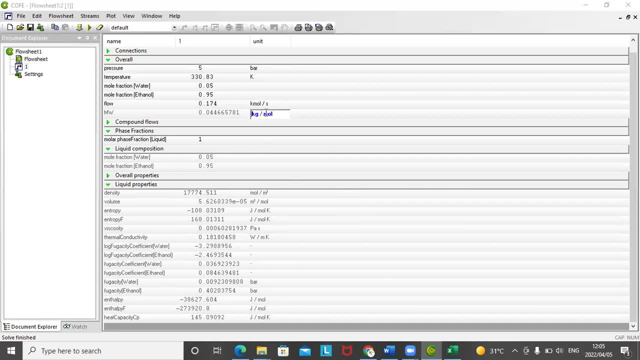 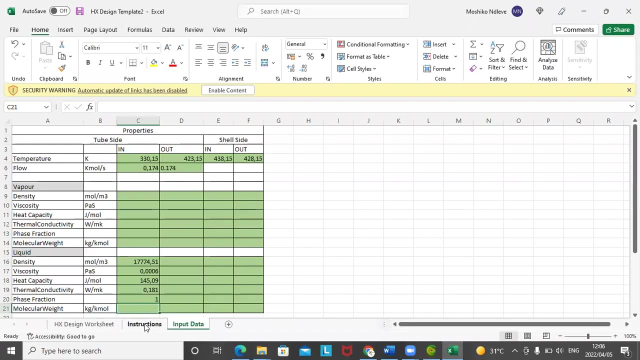 that it's given it to you in the right unit: kg per mole. we need it in kg per kilo more, which is, for the 4.6- let's go back 44.6- again highly critical that your units are exactly as they should. and then now we go to our, our outlet stream. 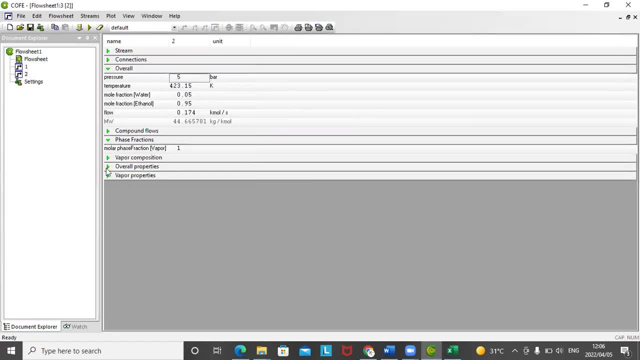 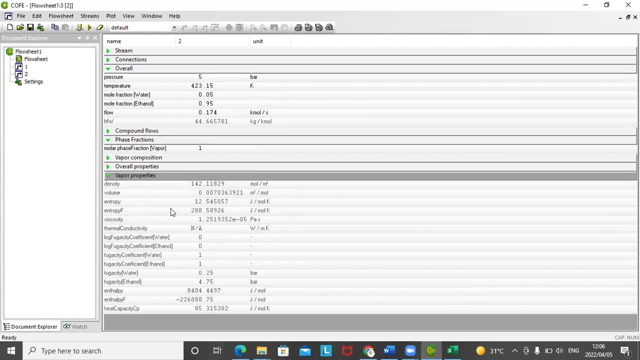 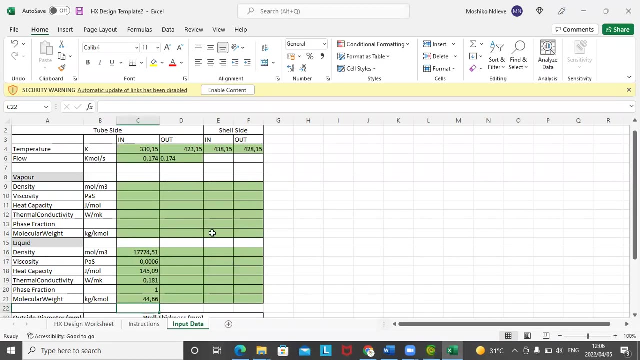 that that was like that, and again. now you've got a vapor fraction of one, so which means all your properties will be in the vapor phase. so let's get started again. our molecular weight is 4.66, so that hasn't changed. so after stream, 44.6 and we've got a phase fraction of one in the vapor. 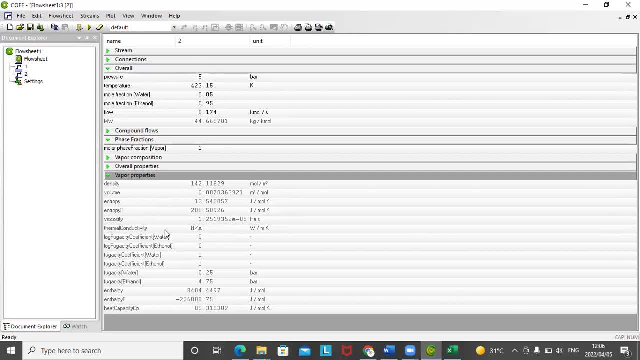 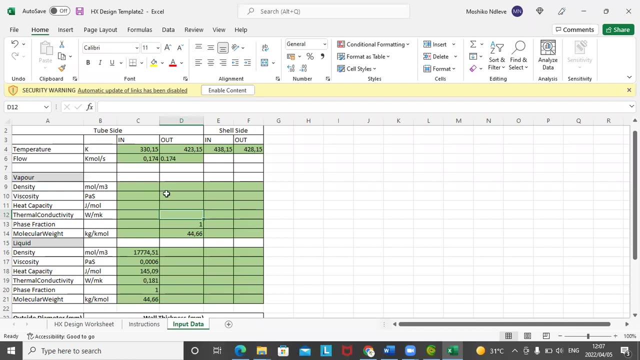 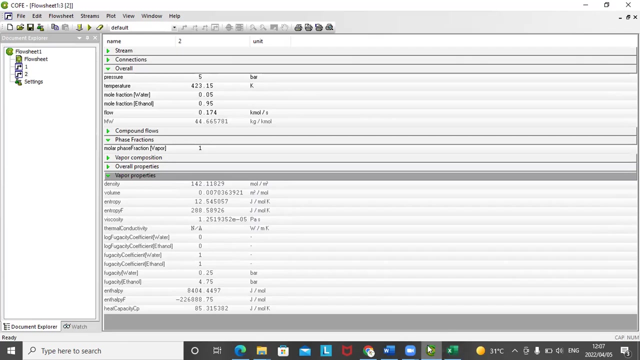 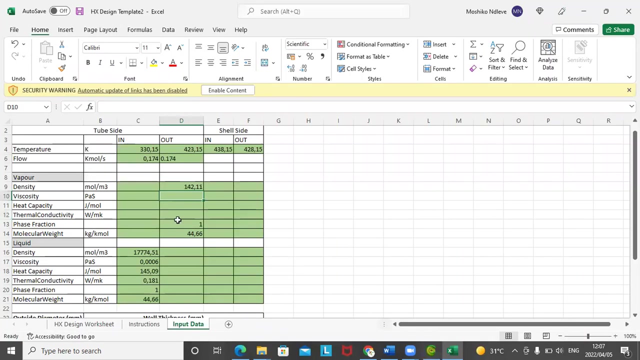 let's go look for thermal conductivity. our doesn't give a value for thermal conductivity again, so you leave it as it is. and then we're looking for density, which is 142.11. density is 142.11 and then your viscosity. viscosity is 1.25 um times 10 to the negative 5: 1.25 times 10. 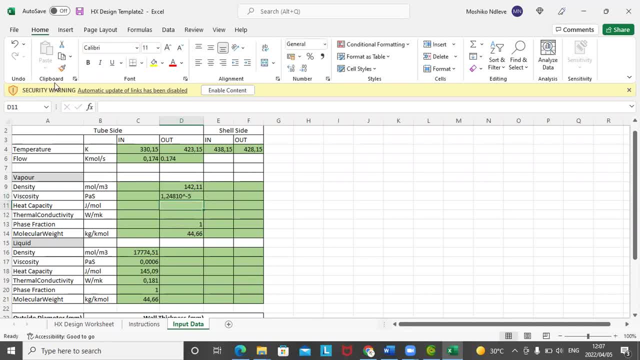 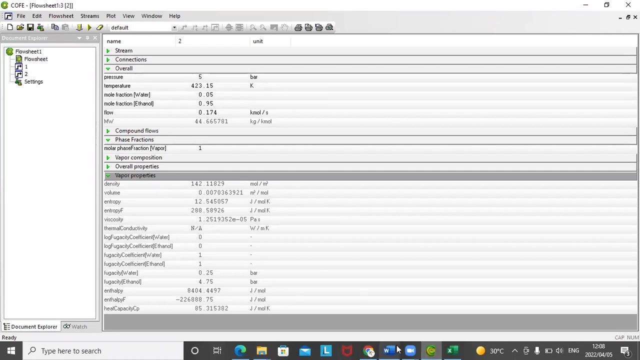 uh to the minus five. one copy there, because i haven't said it was two right color times. oh see, i'm coming to form times 10 to negative four. so it should give us the same value, yes, and then, um, our heat capacity, uh, cp is 85.315. 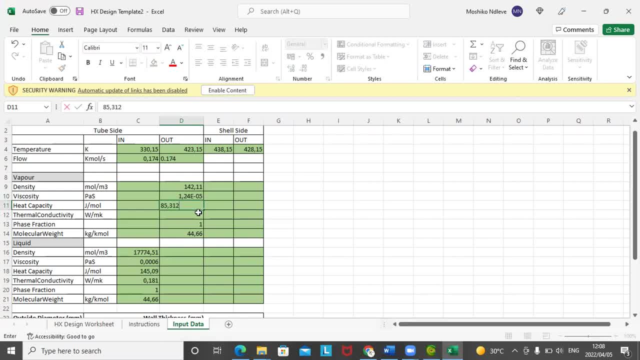 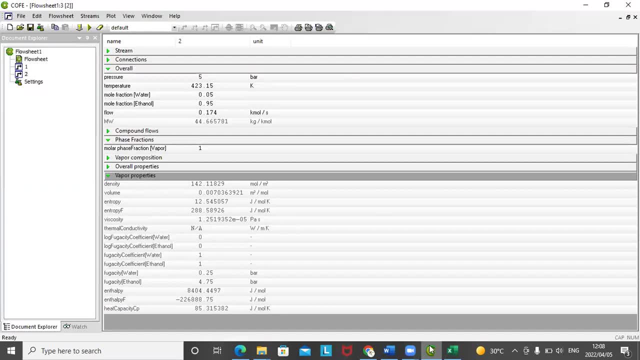 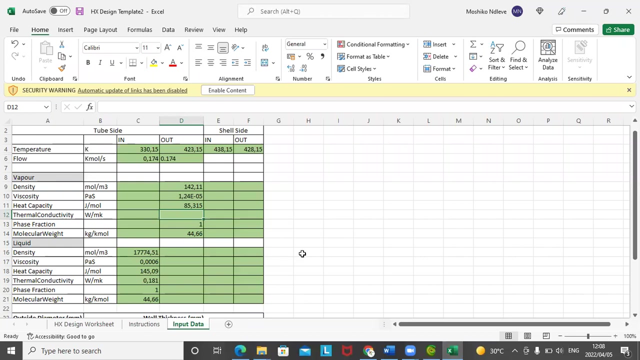 85.315, 85.315, and then our thermal conductivity, signal conductivity. uh, as i said, it was not given on this particular one, so which means that when you're doing calculations, if it ever requires you for a thermal conductivity, you'll use delivery. now let's go back to our special. i know we still need to do the shell side. 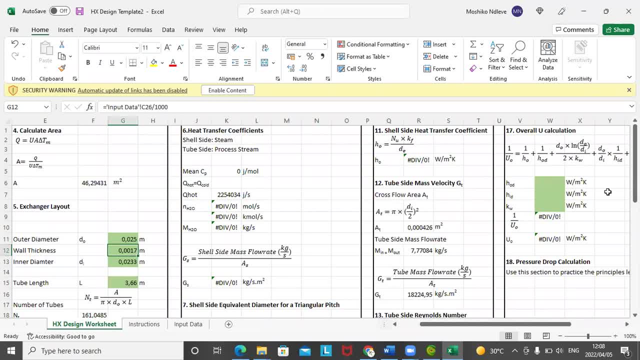 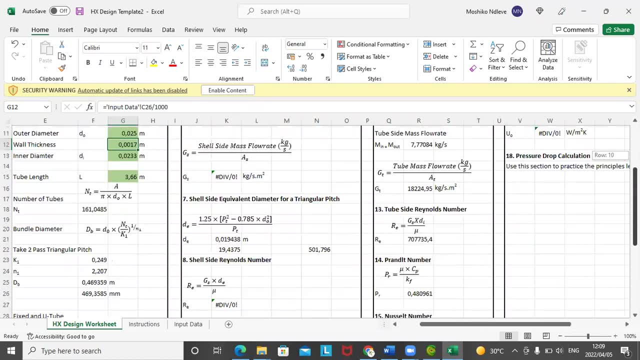 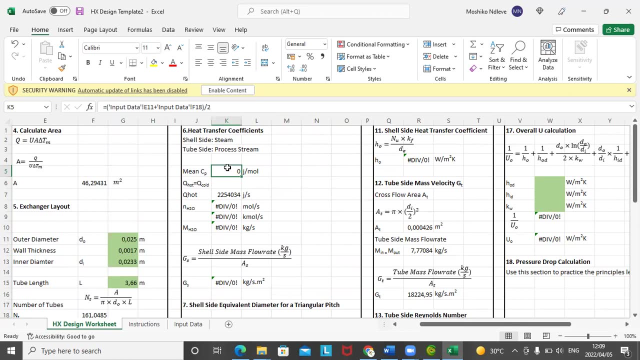 um, i just want to give you an idea to show you that most of the values should start opening up. so let's see um. you can see that some of the answers are starting to pop up. so this one needs this particular cp. so we're dealing with the shell side. 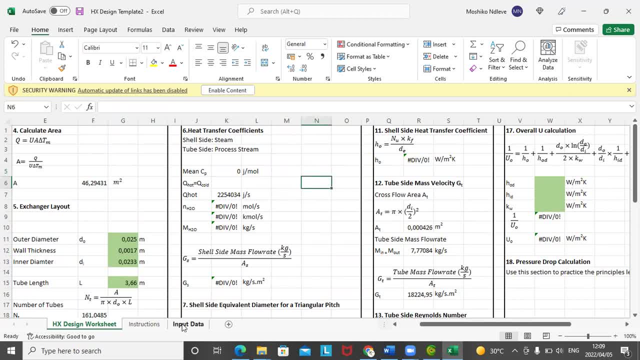 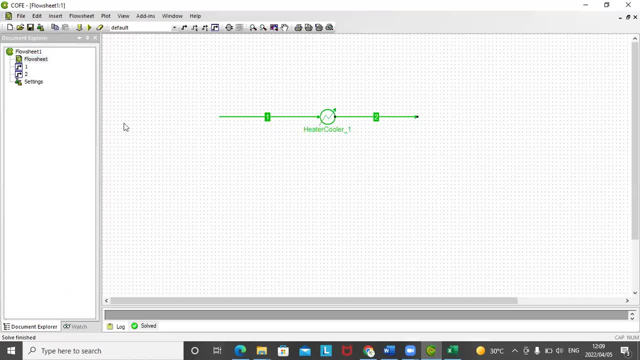 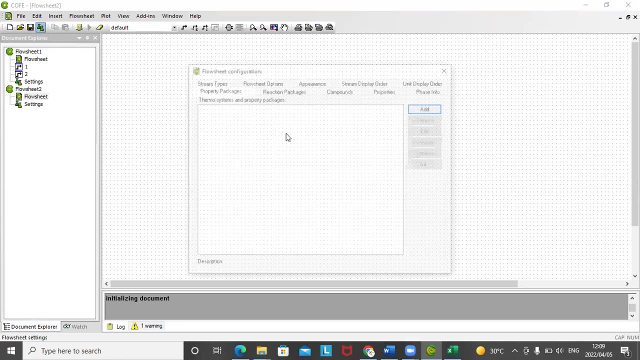 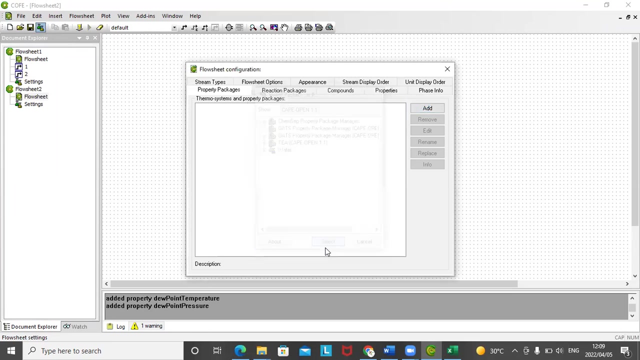 so this particular cp is of the bottom of the steam. so again, we need to fill out this section and in order to do that we need to do a new simulation. but now just water. so we're going to click new and then, here now, properties, add, add. and instead of jumping to chemself let's just do. 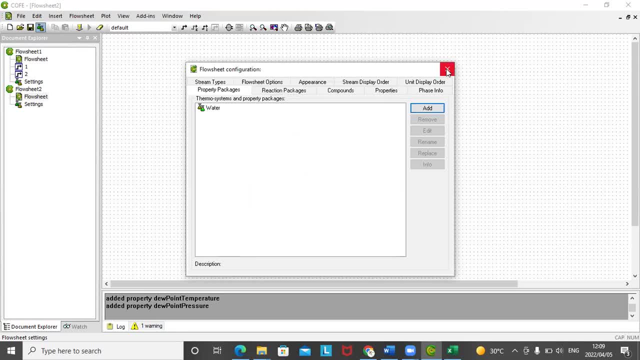 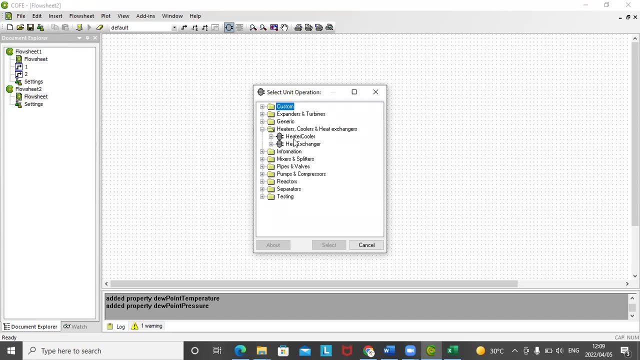 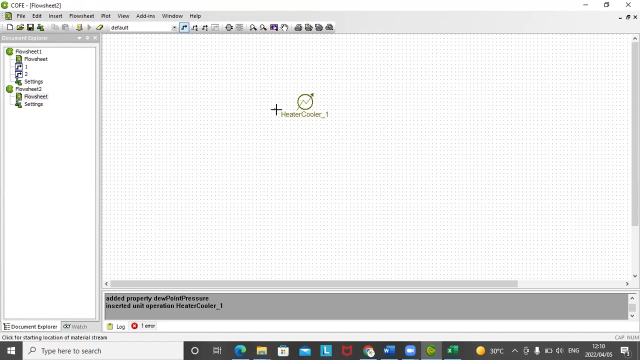 the water one. now assign property track in the cage, close that and again run it through a heat exchanger. so, as you can see, you are doing the two separately. you can do them on one simulation. um, it is actually quite easy to do, uh, but again it needs you to have a proper understanding of your approach. temperatures: 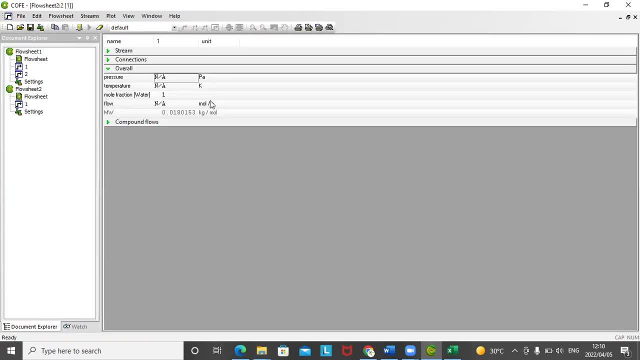 so this one is quite easy to do. we said our steam is at 6.6 bar. 6.6 bar, uh, it's coming in at the temperature of- let's go back- of um 48.15, and then the properties we're looking for now are not really dependent on how big your steam is. 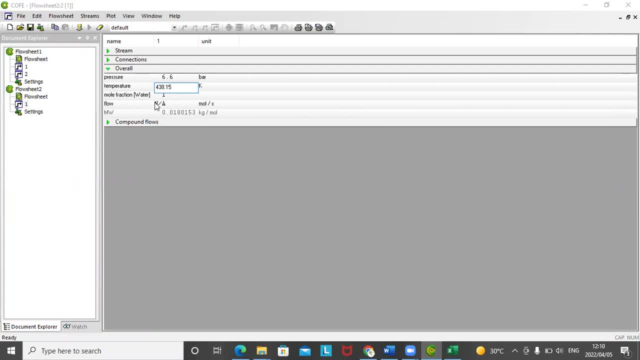 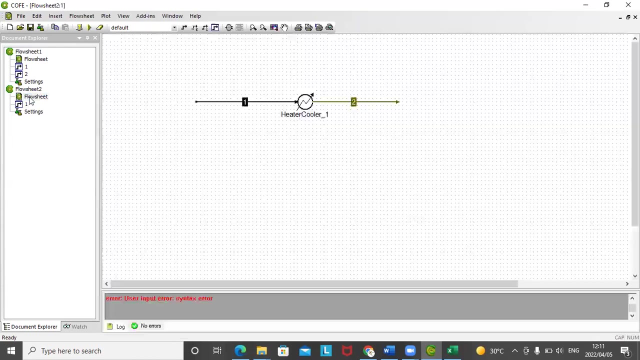 48.15. and then, um, we are going to do, let's go to kilomoles just so that we're, because we're used to, and let's just work with one kilomole. then, uh, what we'll then do is we're going to do a. 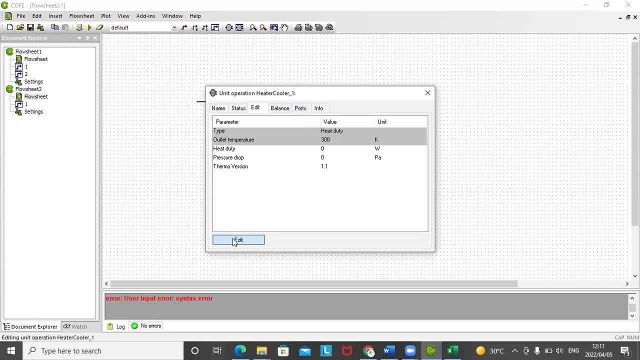 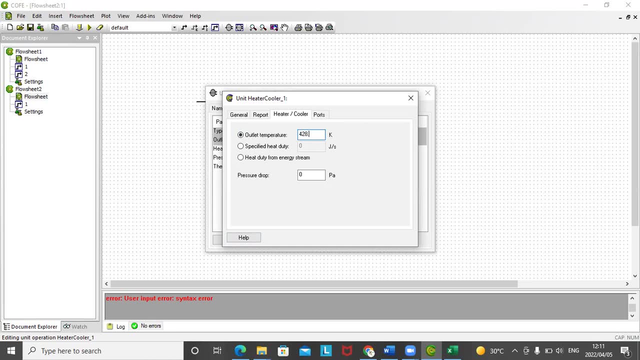 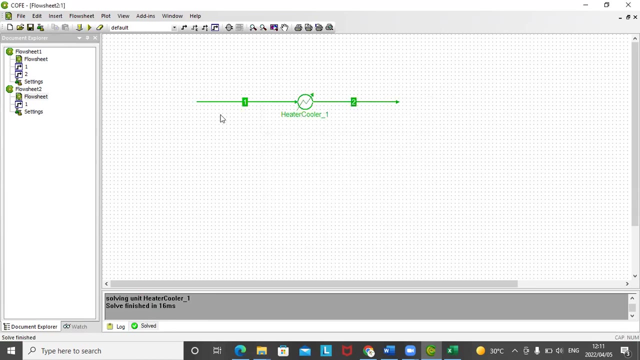 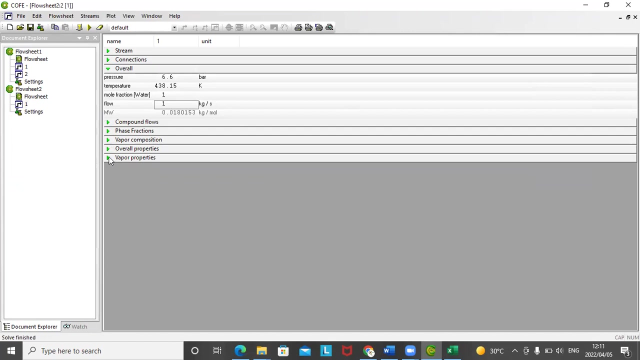 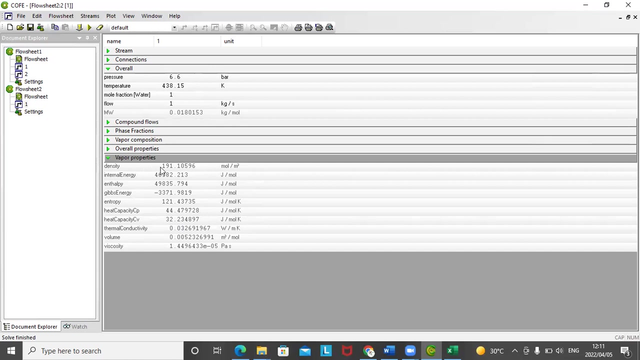 is uh. define our outlet temperature, which is 428.15. we run our simulation and we should be able to get all the information we need. so look at that. so again, your we're going to take the values we need. um, let's change that to what we're used to. 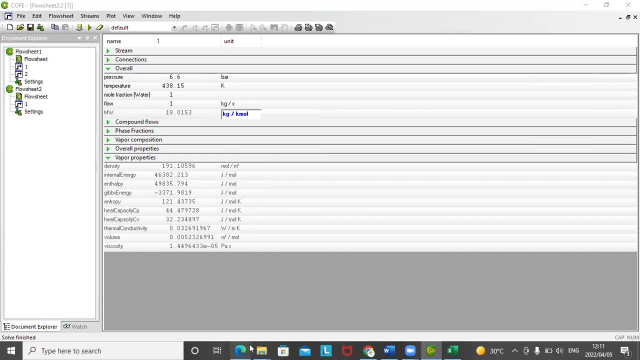 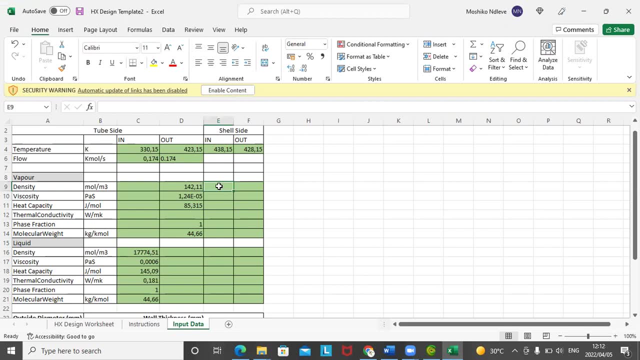 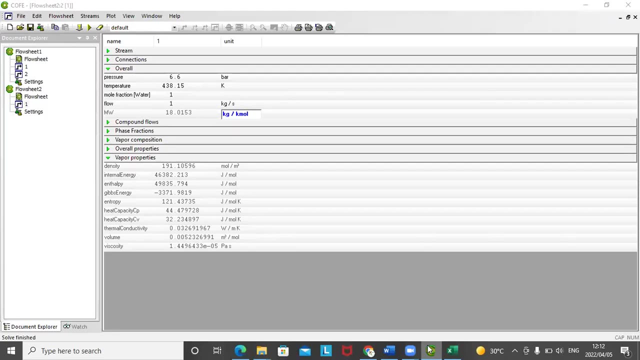 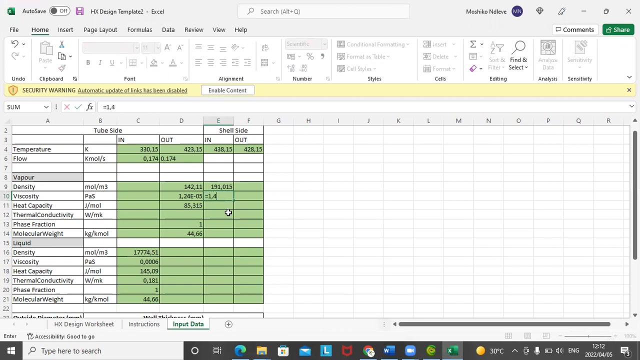 okay, so let's start. density 191.105 density um, so coming in it's just vapor 191.015. and next we look at the um viscosity, which is 1.44 times 10 to the negative 5 viscosity equals to 1.44 times 10 to the negative 5, right? 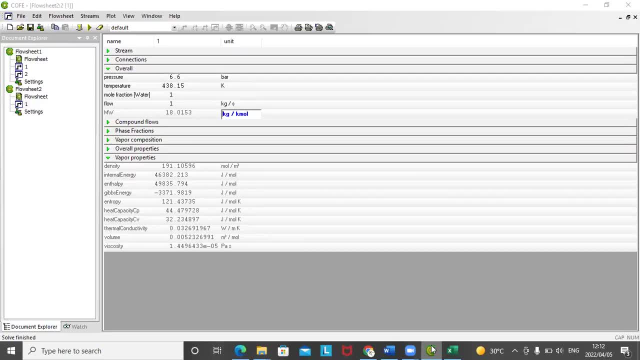 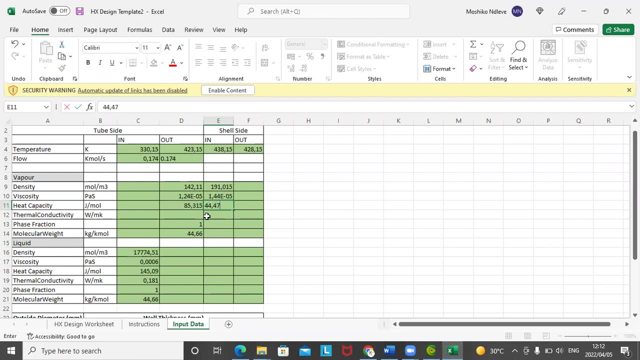 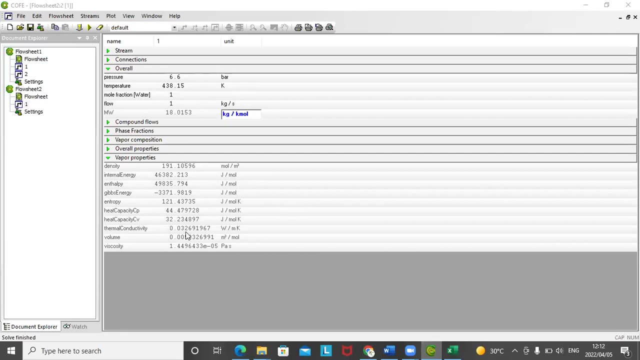 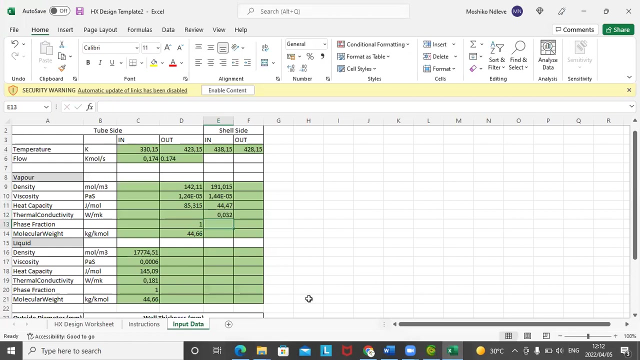 uh. next is heat capacity, and our heat capacity is 44.37, 44.47, sorry, 44.47. next, our thermal conductivity. our thermal conductivity is 0.032, 0.032 phase fraction- here we've got one- and then our particular weight is 18.01. 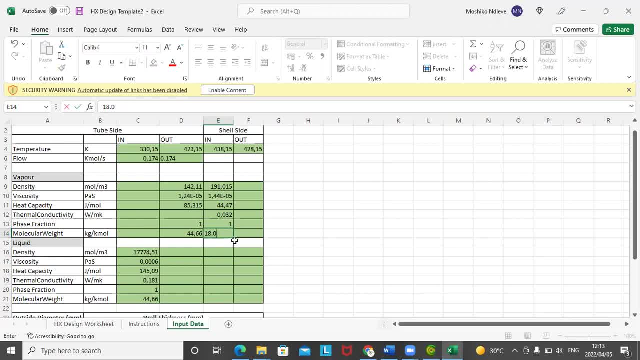 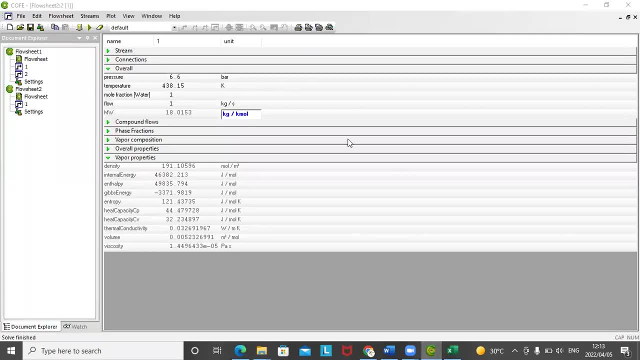 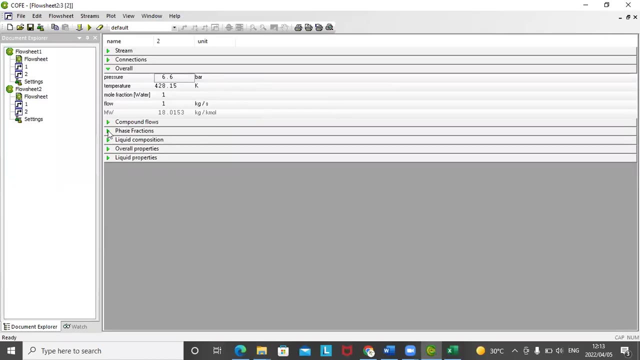 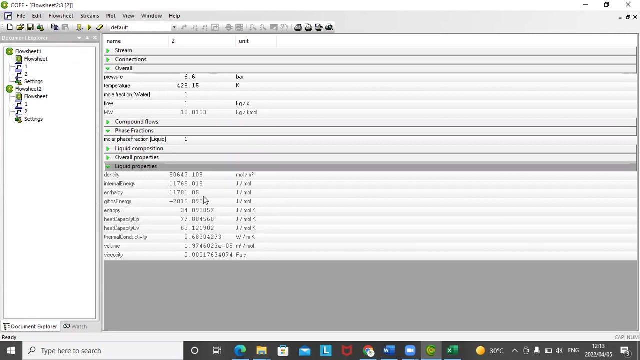 18.01. it is water after all. so that's when we define in the input and then output, we should have two fractions, phase fractions, but only liquid. so our density is 5643.103, 56.3. so out, we're going to put in the liquid. 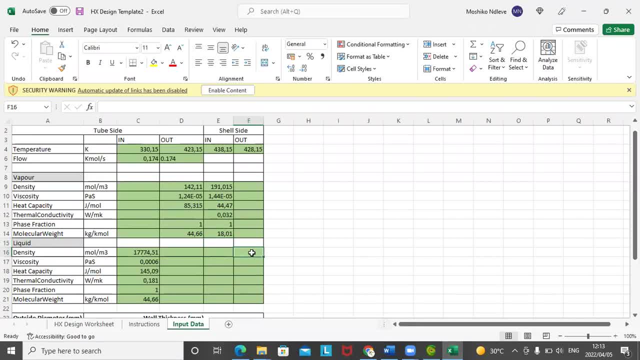 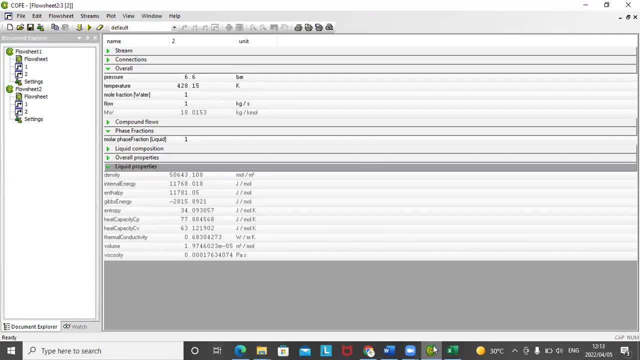 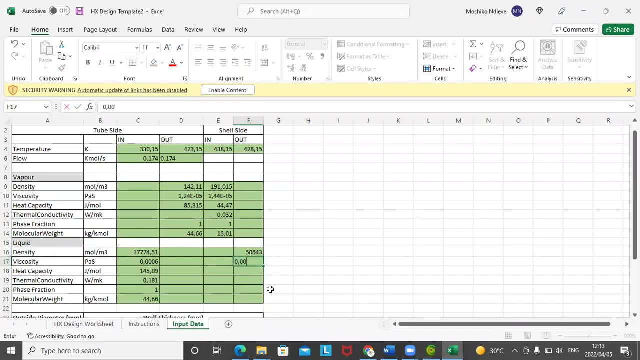 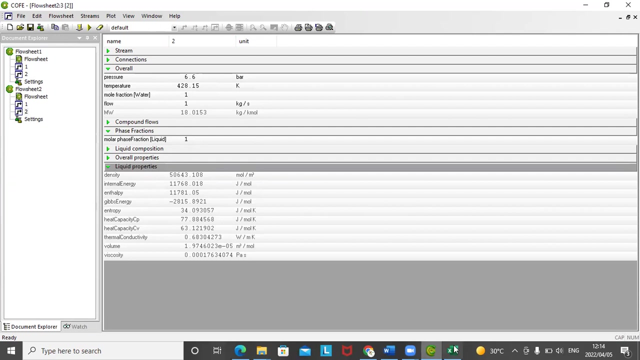 5643 so out, we're going to put in the liquid side 5643. i'm just going to go through this quickly, um, so we can get to the whole point of this and then i'll discuss. it's not point. triple zero one seven, uh, not comma. triple zero one seven six, and our heat capacity is 77.88- 77.88. 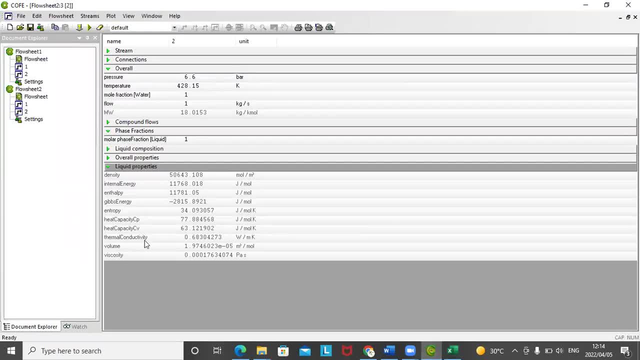 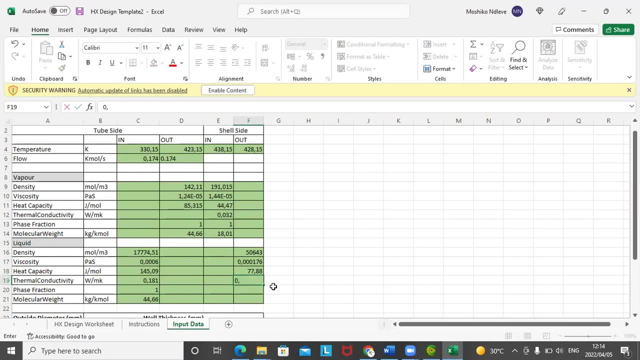 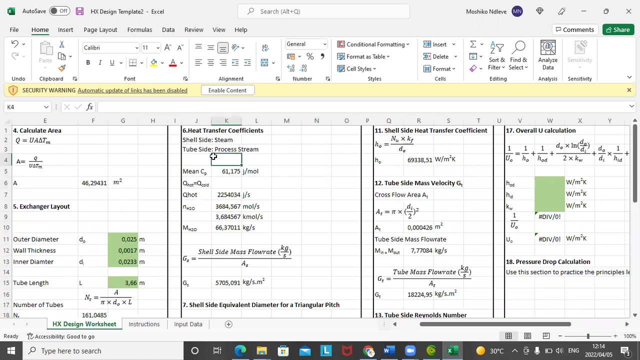 and our thermal conductivity. thermal conductivity is not 0.683, not 683. base fraction, one molecular weight, again obviously 18, 18. now let's go back to our calculations. um, we've populated most of the information and now you go back you see that in the calculated your mean cp for the shell side, it will give you the 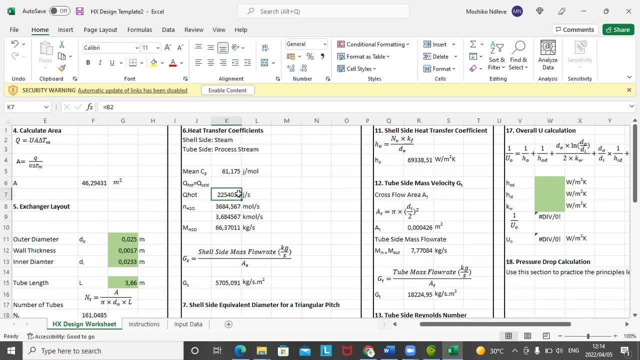 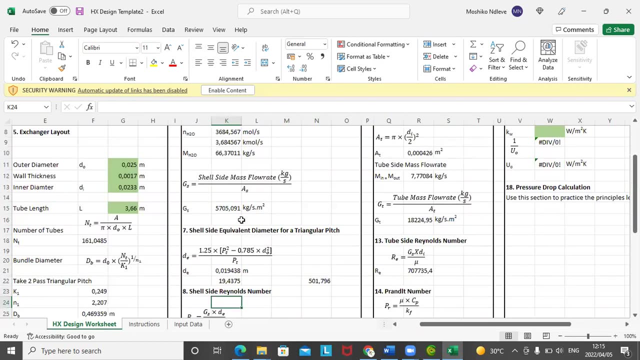 your, your hot and cold. uh, your hot and cold? um, the heat loss by the hot stream is gained by the cold stream. therefore, your calculator, you're going to be able to calculate the amount of water you need for that kind of cooling, which is 6.37 kg per second. this will give you the? um, the mass, the, the. 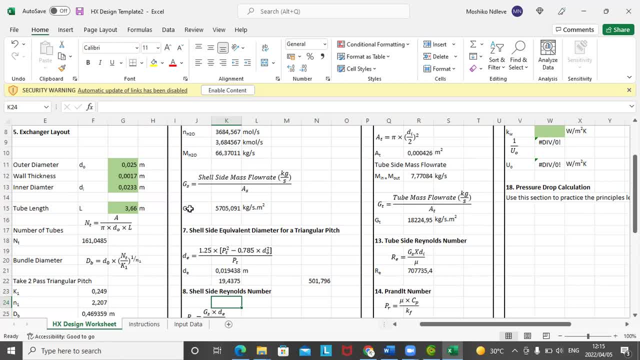 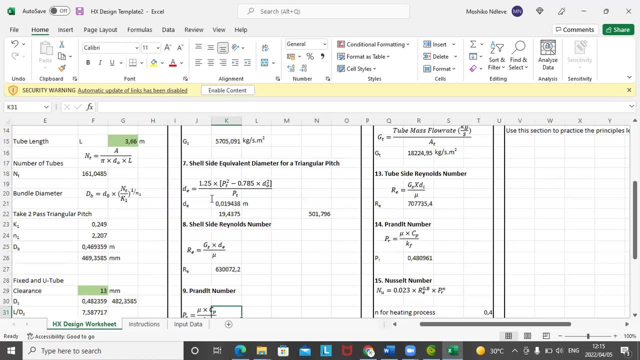 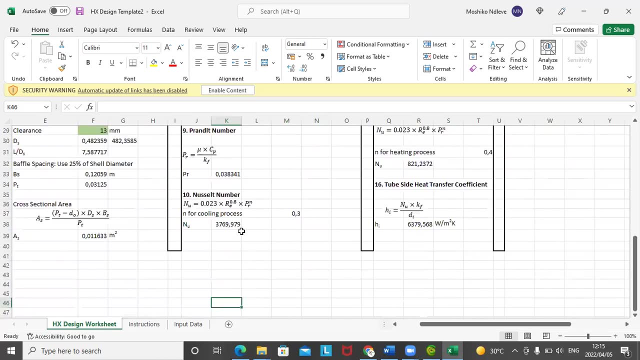 the mass velocity of your uh mass velocity of your um, of your shell steam, um. from that you'll be able to calculate your um shell equivalent, that your, your shell equivalent diameters, which will give you the Reynolds number, a planet number, and finally it's called the Gernasov number. i will go back to the 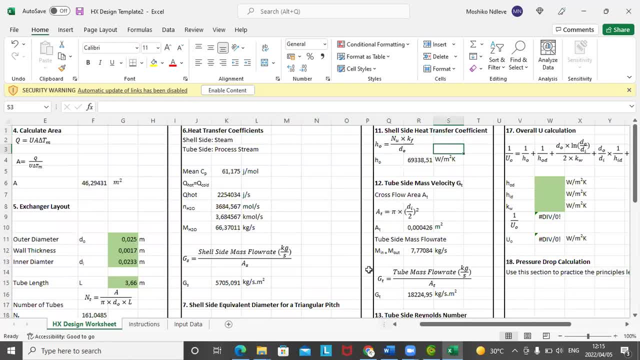 web spreadsheet, uh, today's to the web document. um, i just don't want a lot of time, just want to show you that with just um, the information we've talked about, uh, you can weigh the water concentration and So far we are able to get as far as your on your heat transfer coefficients, and the only things that we're missing will be your, will be your, your fire, your factors, which is HOD and HID, and your, your productivity of your, of your, of your field. 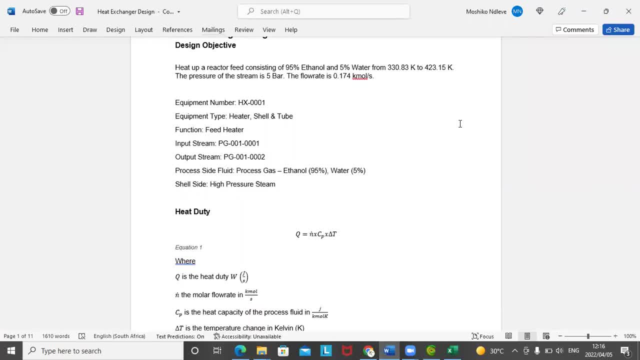 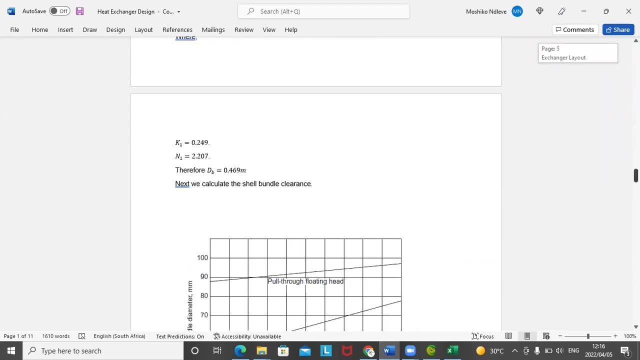 So let's go back to our spreadsheet. So, so far as you see, it's almost completely populated. Now we can come back to our document And, as I said, I do have to rise to. you have seen the gist of it in terms of how it works. 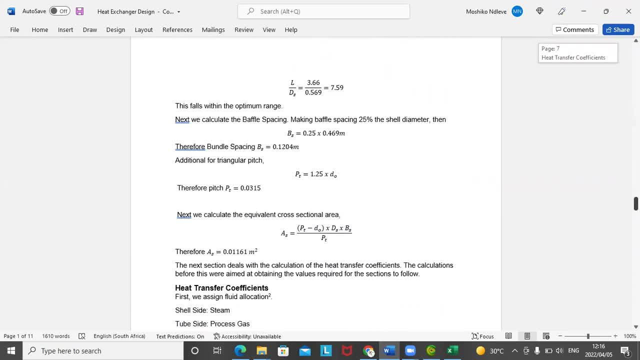 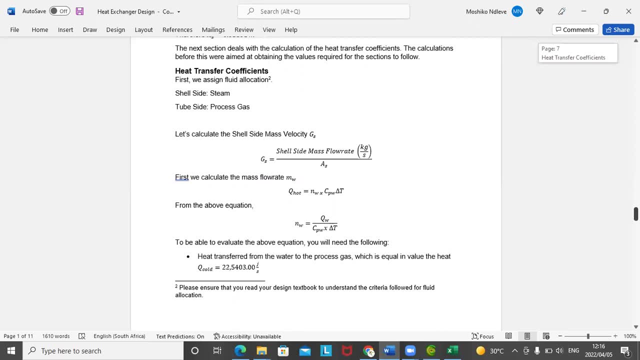 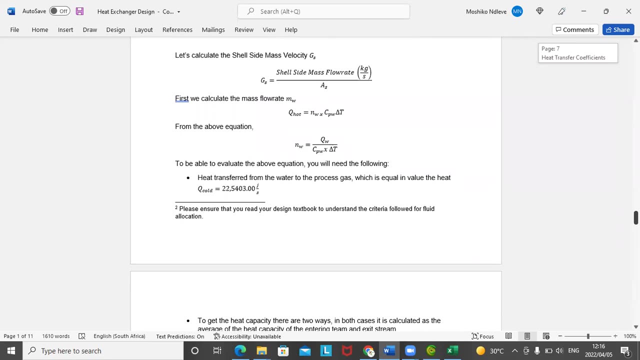 So your, your, what document will give you a step by step detail in terms of how everything is done. As you can see, you have to assign your, your fluids, you know. give you the formulas and show you how everything works. Everything is derived. giving you explanations as we go where to read, what to follow up on. you know how to get your heat capacities. 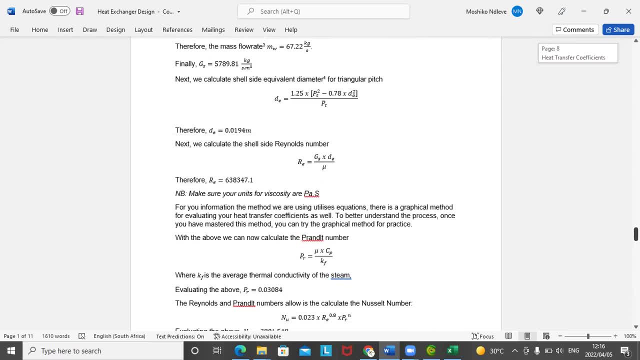 So, property tables, or using a simulator, which is what we did, I'll take you on to how to calculate the Prandtl number, bit of information on where it is. but, as I said, most of that stuff is found in your textbook. 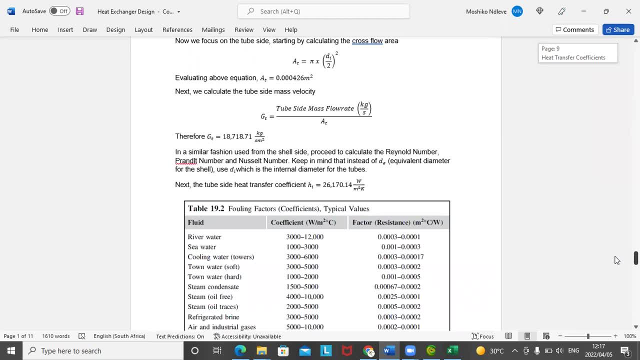 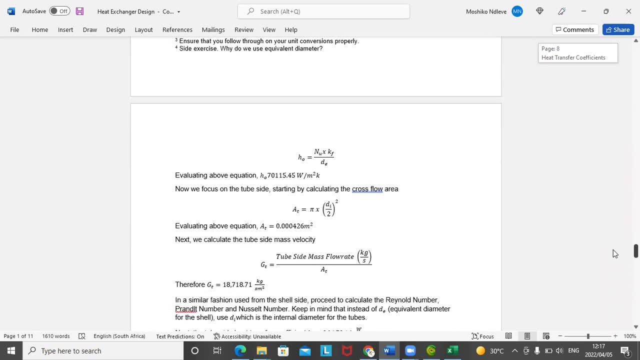 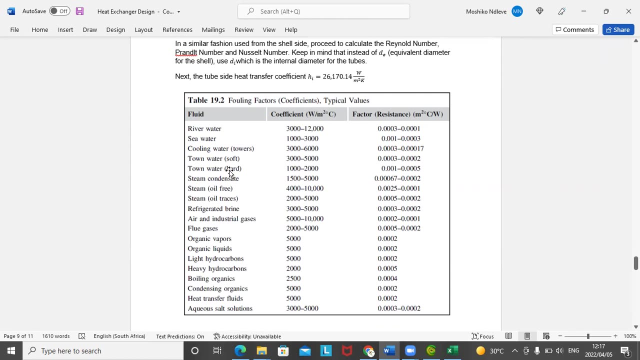 We'll proceed to calculate the Nasalt number. And again, this is, this is. and then, for the truth side, it also gives you the formulations on how to do that And in terms of everything that's there, And finally you get to this table which will give you your, your typical following factors, and we are using: 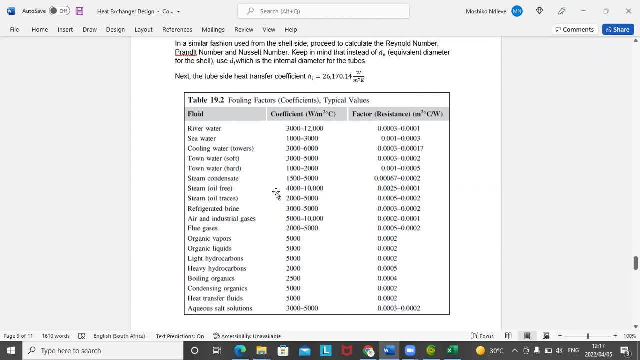 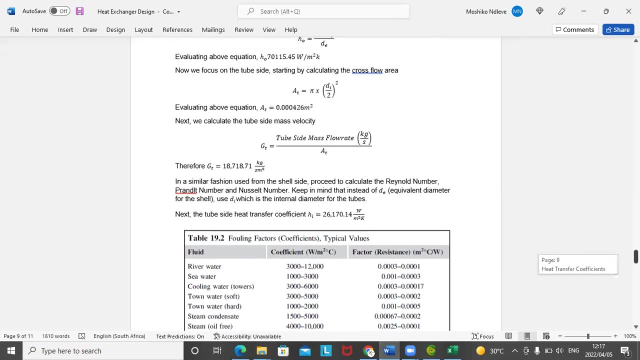 condensate steam, which is between 1.5 and 5000.. So for that one, let's take some in between. So let's just make sure that we assign the right ones. And so these are typical following factors. So so what you then do is: 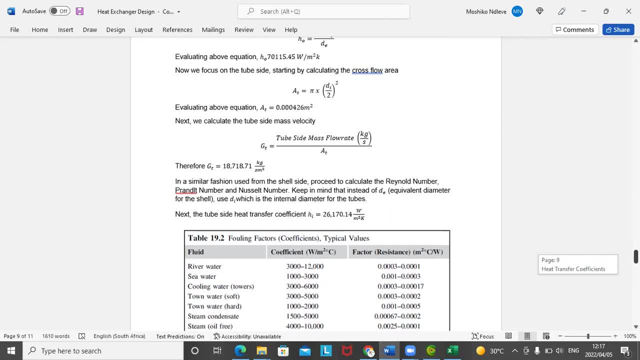 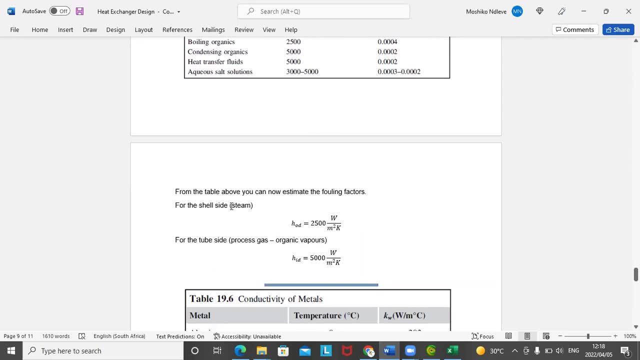 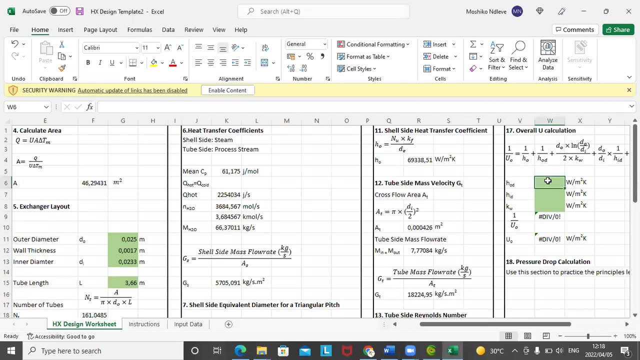 Next, the heat transfer coefficient HI is 26.16.. So what would? from the table above we can show that the estimated following factors: so for the shell side, which is the steam HOD is 2.5.. So just take that directly from the table right: 2500.. 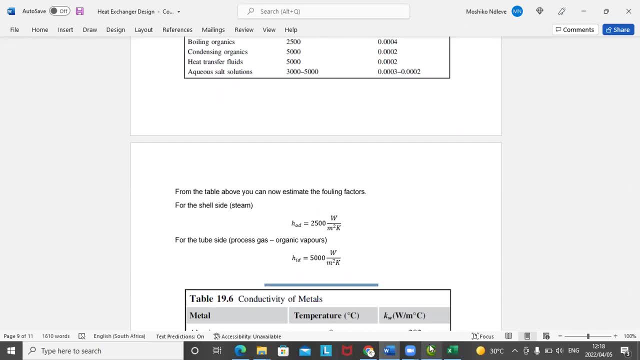 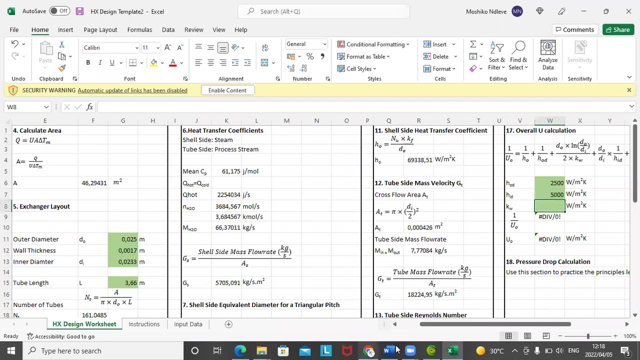 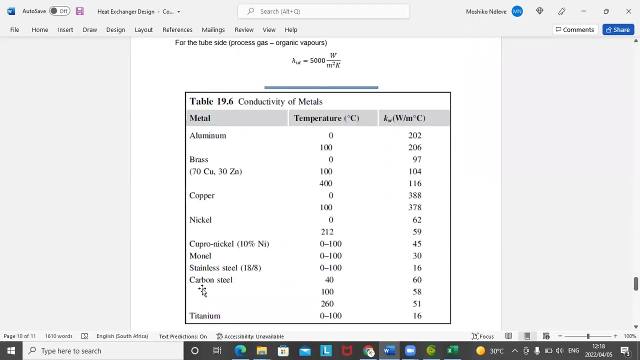 And then next, From the table, ID is 5000.. And then, finally, we need the conductivity of the metal And in this particular case we're working at about. So you look at, you look at your temperature ranges, so it will tell you that, for example, your brass can go up to 400 degrees. 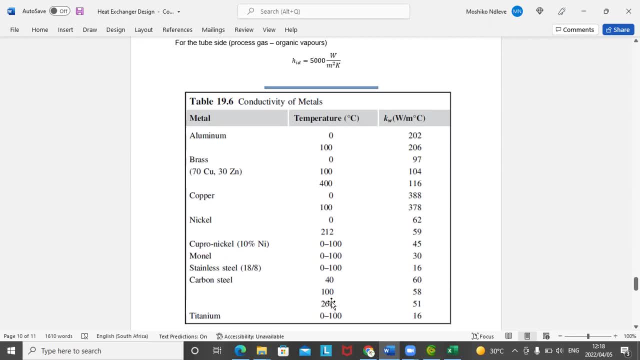 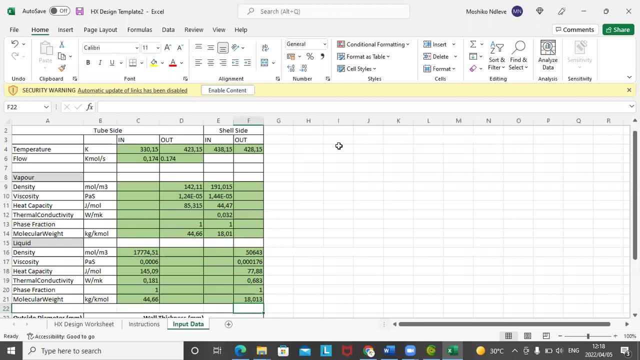 And then your carbon still can go up to 260 degrees. So in our case we are working at the highest temperature we're working at- let's just go back to our table- is 423, 423 Kelvin. So if you take that and minus 273.15, 155. 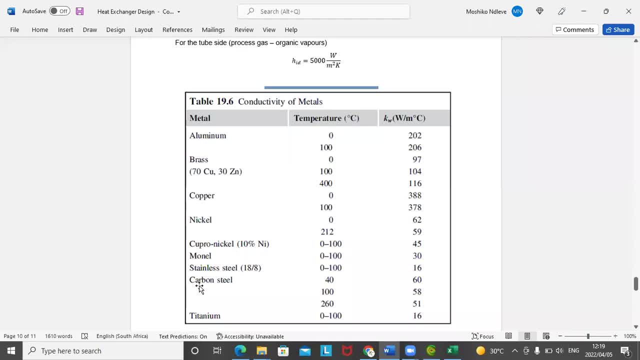 So if you go back to our table, we can see that carbon still suitable for this, aluminium could be suitable for this. So depending on Which comes cheaper, you will then choose that. So for now, let's just go with carbon steel. So with carbon steel, if you're working at the range of about 100, your conductivity is 58. 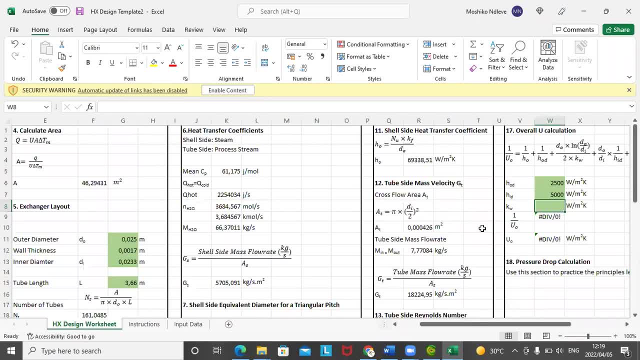 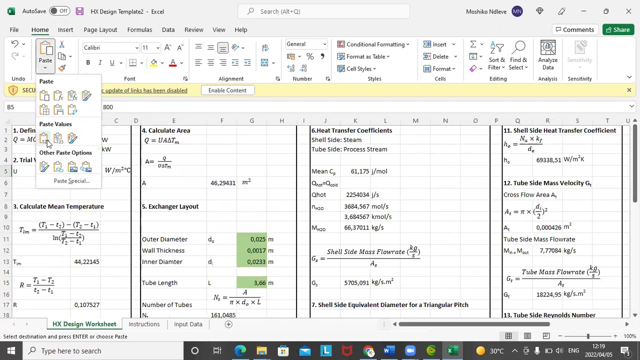 Come back here and come to our spreadsheet and we input 58. What that will do is it will then calculate your U value. Now, if you remember, the initial U value was an estimate, right? So what we need to then do now is we need to take that U value, copy it and then come paste it as a value on the estimate. 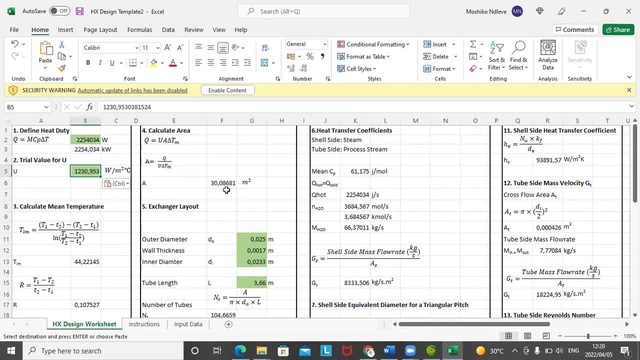 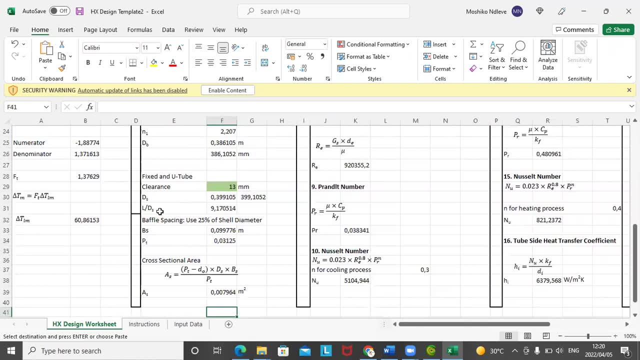 And what you'll see happening is that things will start changing. Your area, for example, now, is smaller. right, There's a little. there's a place where we put in a calculation of L over D, which is your tube length over your shell diameter, 9.17.. 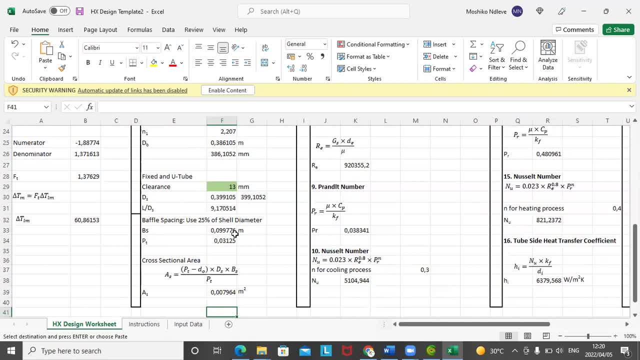 It's between 5 and 10.. Which means our exchanger is 9.17.. Which means our exchanger is working in the approximate right area. And we then come back to check. our U value is now 1,, 2,, 3,, 6.69.. 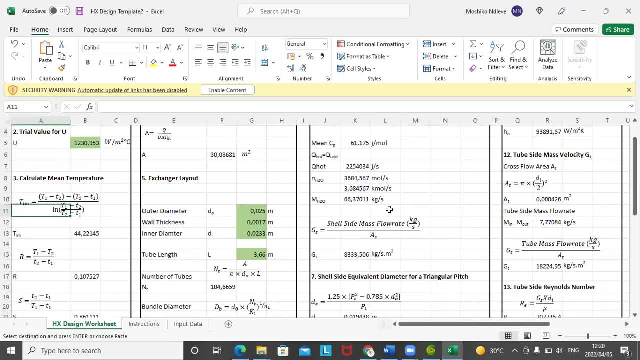 We then copy that again and compare it to the one we have here. So again, you pick the number. Now it gives you 1,, 2,, 3,, 6.69.. You go back to your U value, you copy that and you continue doing this until the numbers converge. 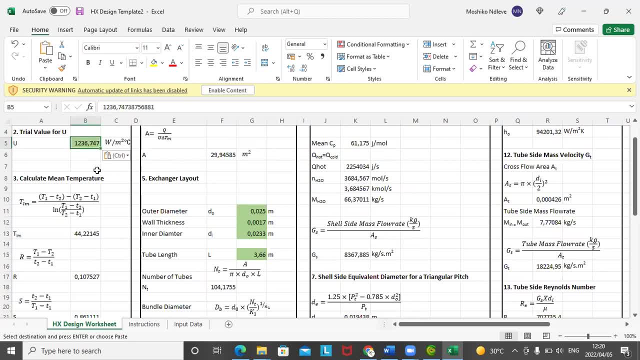 And what do you mean by converge? And what do you mean by converge Until the numbers, until the estimated U value, the current value and the new U value are exactly the same. Let's go back again Now. they are the same. 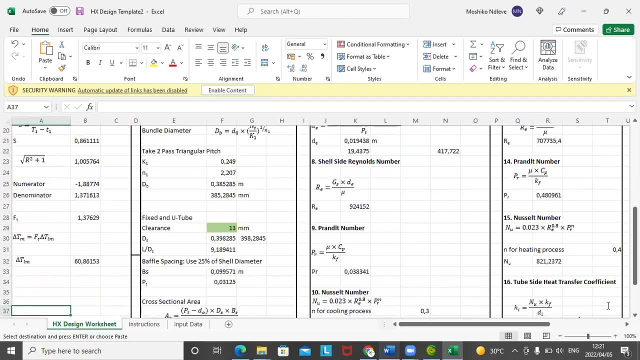 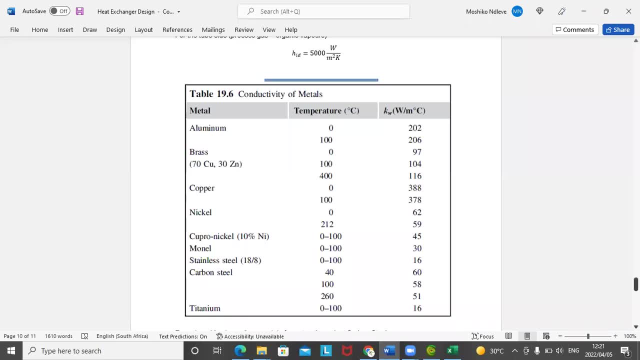 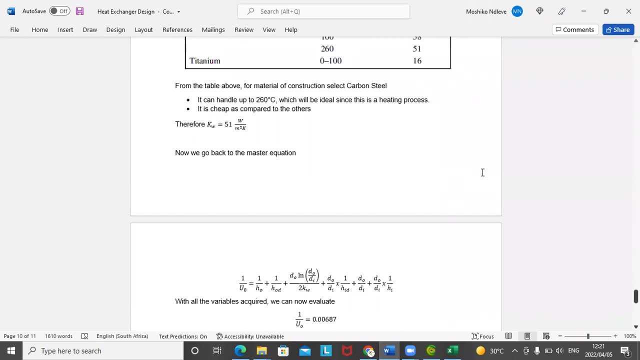 And then from our L over D, our L over D is still below 10.. Now you come back to your instructions. That's actually it for this lesson, And one challenge that I put in for you is what you then need to do is, obviously, you'll be able to populate your. you'll be able to put in your new value. 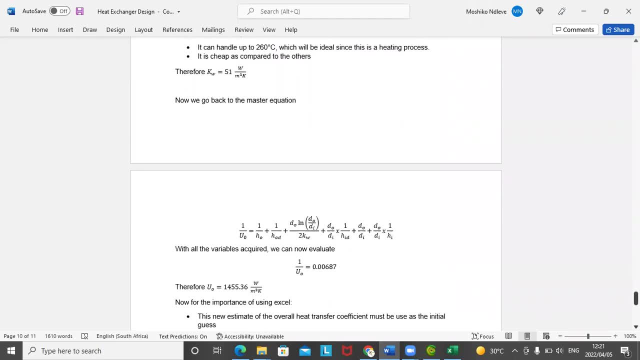 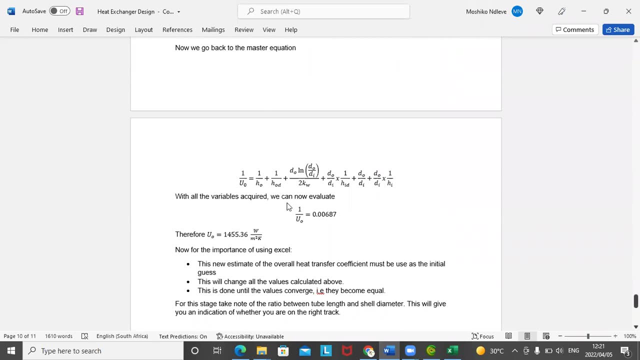 This is based on that particular estimate value that we have, But you'll be able to calculate your final U value, And in our case it was 1,200.. And then what I have here is just a few notes for you. For example, the importance of using Excel, especially when it comes to iterations. 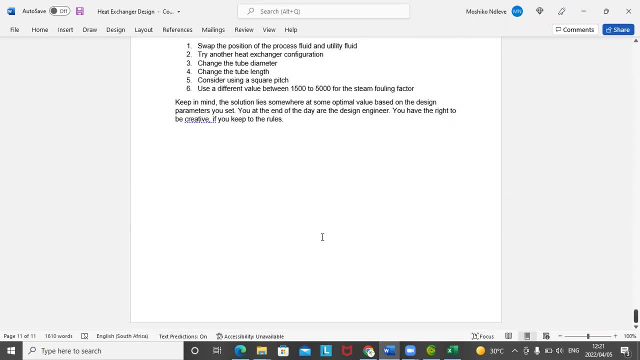 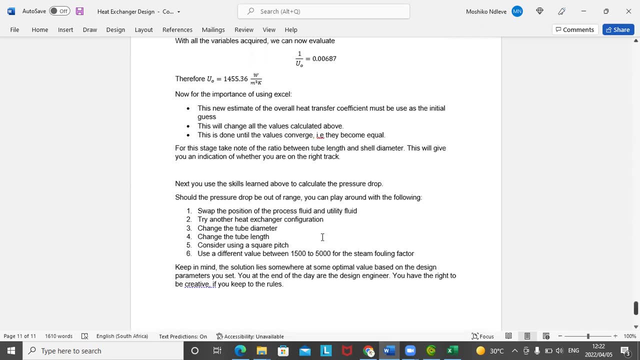 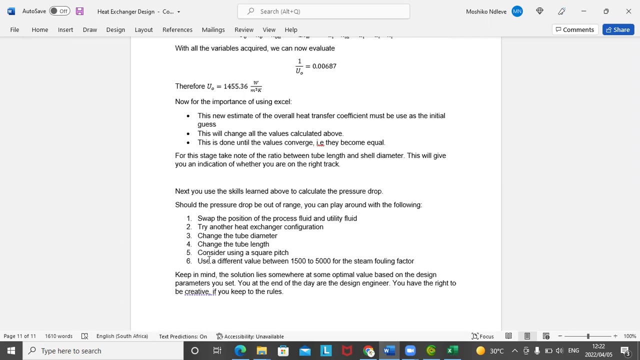 So it is quite important for you guys to using things like Excel, because one it allows you to do iterative calculations, to pick up, And then what I'd like you to do now is you can do this. What I'd like you to do now is to use the skills that you developed here to check that you can then come back to the spreadsheet that we have. 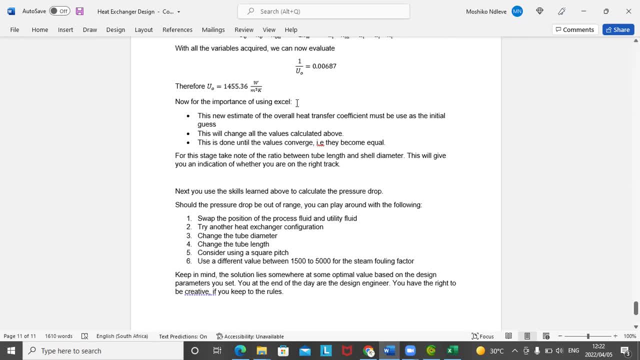 And these are the different ideas that you can use to see if it works. So that's it for today. I hope the lesson was quite informative. At the end of the day, the aim of it all is to try and help students to get better results in their studies. 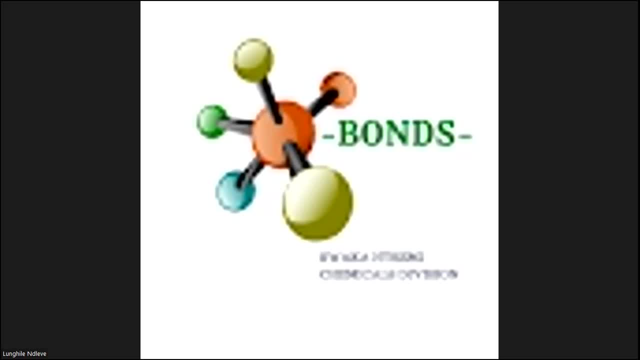 And to also have a broader understanding of the discipline of chemical engineering, as there is so much in it, especially engineering design, which is a personal favorite of mine because of the flexibility And the fact that man design is one thing that we as chemical engineers can say we own, because it happens to have that one section called reactor design, which only we can do. 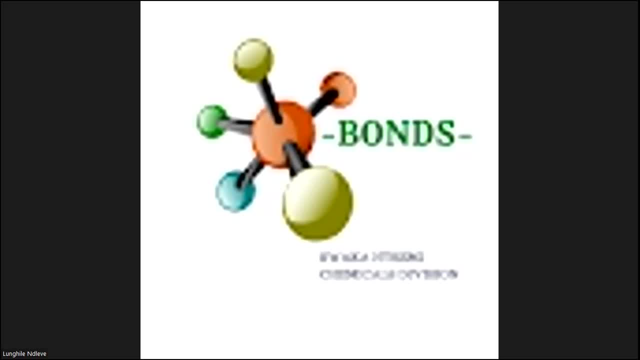 So enjoy your studies this year, guys, And I hope all goes well. Cheers, Bye-bye, Bye-bye.